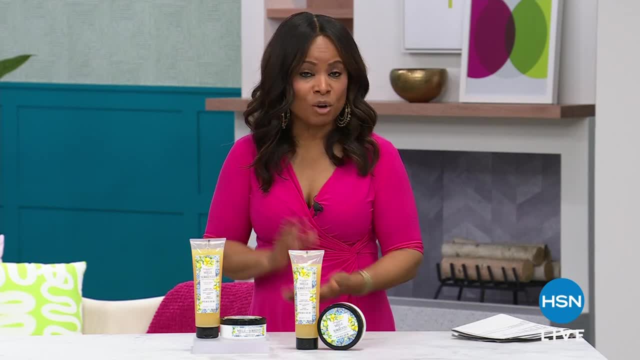 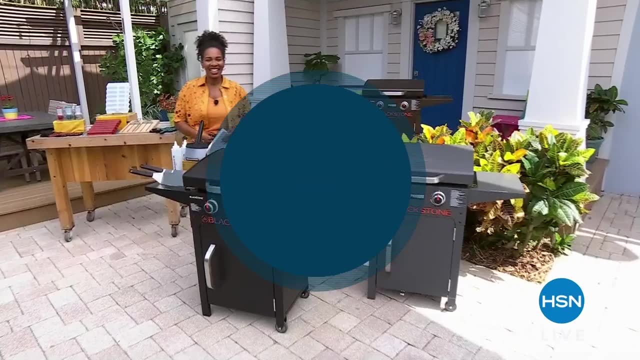 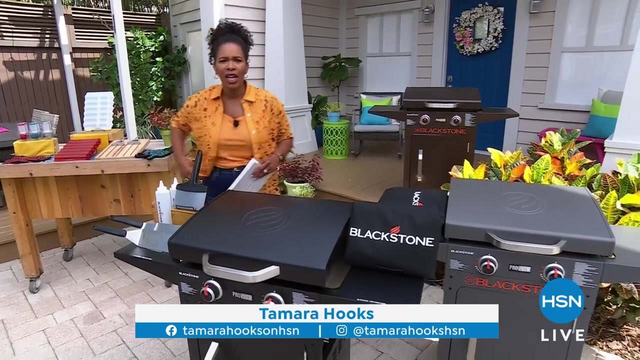 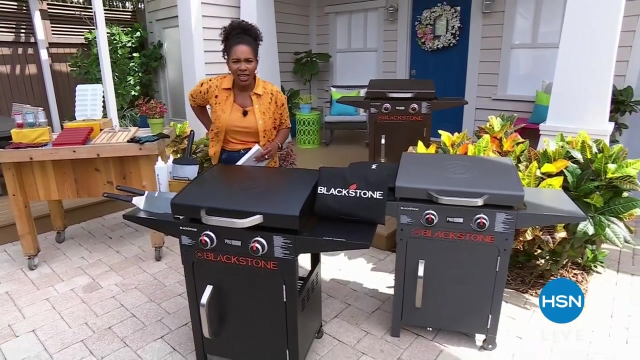 I want to thank you, Amanda and Skip. We're going to see you both tomorrow for the big two shows, Tamara's coming up next with a look at our best value of the day. Thank you, Marlo, It is. I wish you could be out here right now. It smells so good and it's all because we are cooking outdoors. This is what we love, isn't it? This is our today's special. Now. we featured earlier in the day. A lot of you have already gone ahead and picked yours up, But if you haven't and if you're staying way, 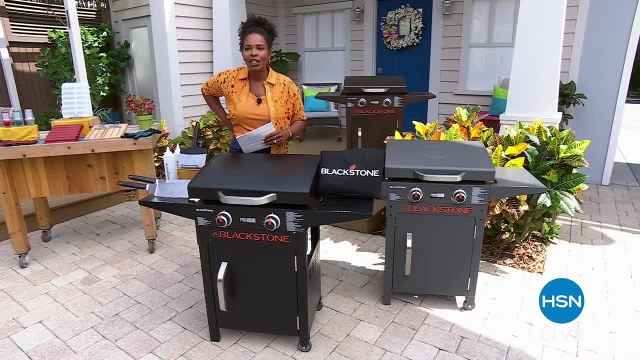 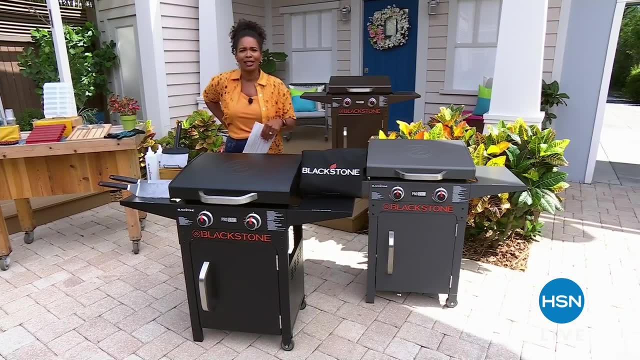 a minute. I'm usually intimidated by cooking outside, But this is a new. This is something that's going to be easy for you, Very simple: It's from Blackstone, The one and only time you're going to see this as a today's special this year. And here we go. 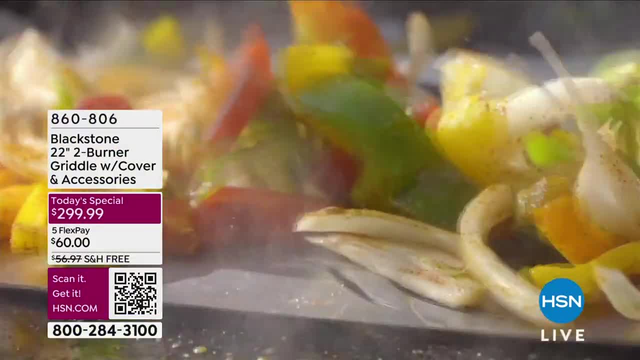 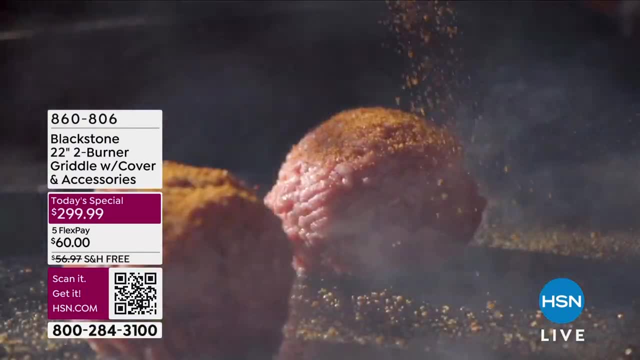 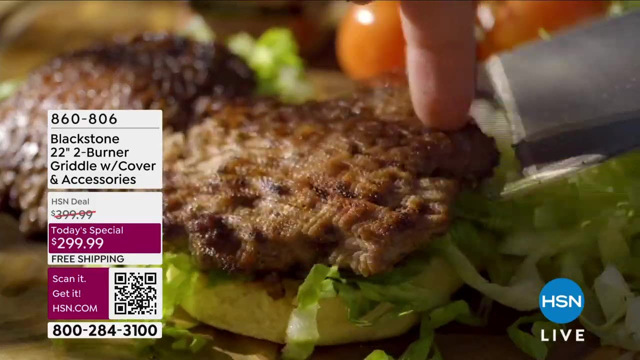 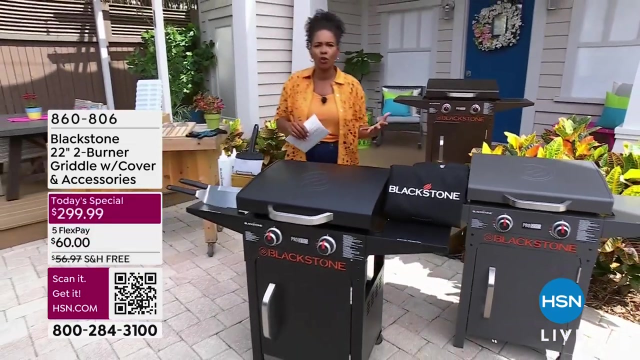 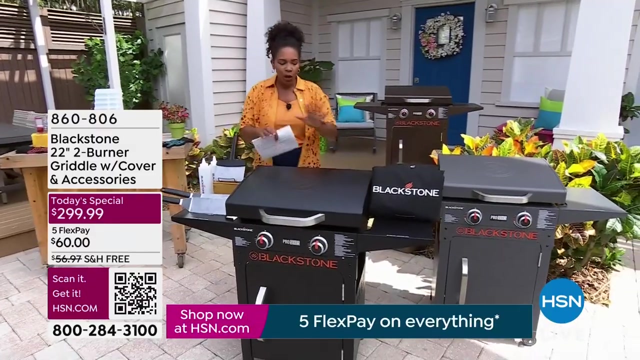 So look at all the food that you're going to be able to cook. Could you do that on a regular grill? You couldn't, because all of those chopped vegetables and and all the shrimp and all the food and the muscles would go sliding through those grill grates, But not when you have the Blackstone 22 inch two burner griddle. So think about all the things that we love to cook indoors, like on our cast iron grill, and those kinds of things on our griddle inside. You're doing it outside in a much bigger way. We are going to show you how it works, But I just want you to let you know that all you have to do is cook. 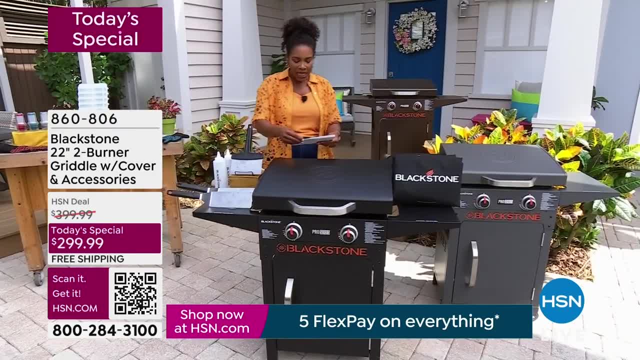 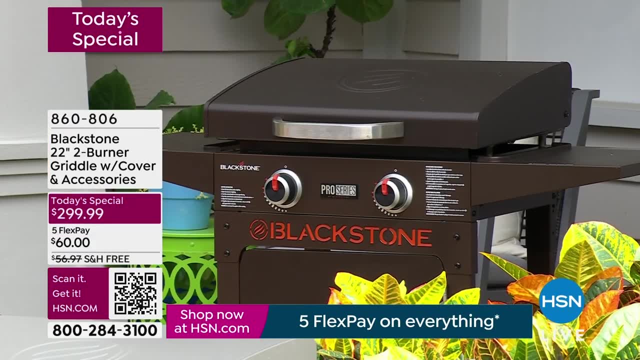 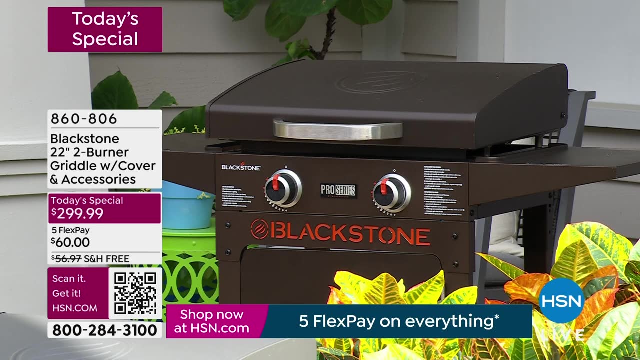 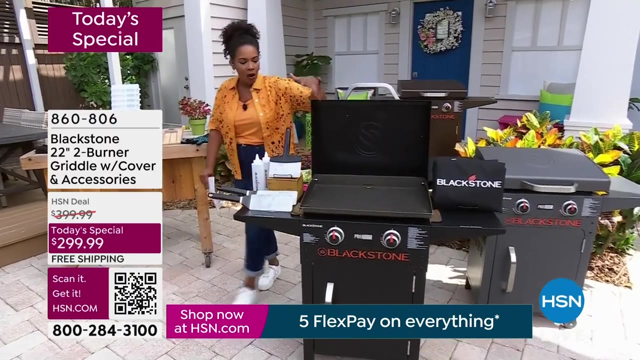 Choose a color. no matter which one you want, We've got them for you now. This one is black, This one is gunmetal. You can see that color, And then, right behind me, we have it for you in this really pretty bronze. They're all very cool. So we've got them all for you. right now. Let me kind of take you on a quick tour, and then we're going to get to cooking and eating. OK, So what I mentioned- 22 inches, This is what I mean. Look at all of this cook surface, And then you even have the ability to have two separate. 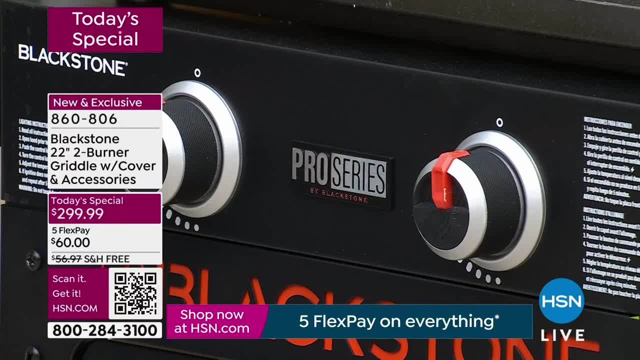 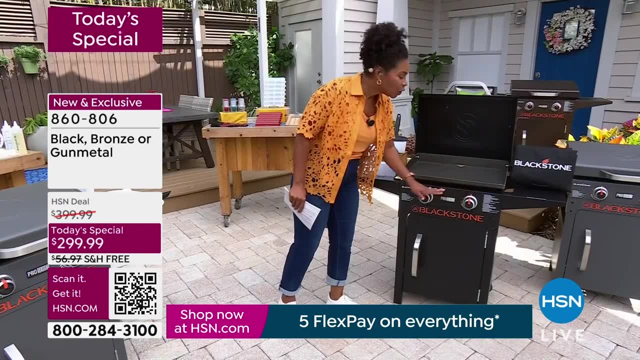 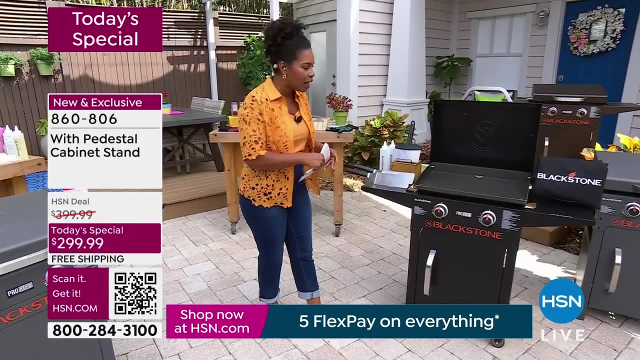 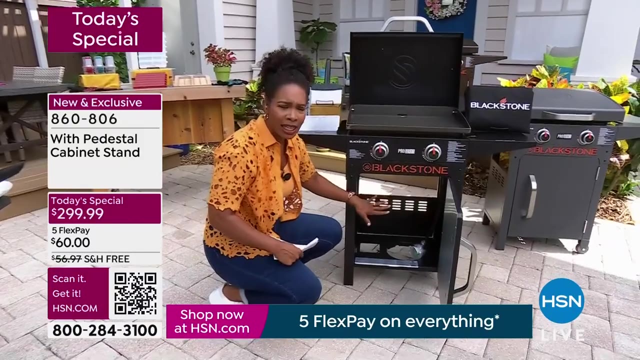 Heat control elements. And I say heat control because when you're cooking with fire you can't control the heat. You don't know how hot it is and you have hot spots and cool spots. But with this you can control the heat in two different areas of this 22 inch surface. You can cook a lot of food all at the same time. What are you cooking with? You've got a space down here, a nice little hidden door for your propane tank, So this is where it sits, up off the ground, So no worries there. And then you just close the door and it's. 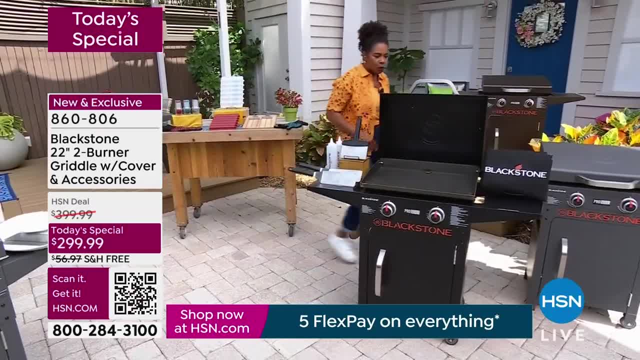 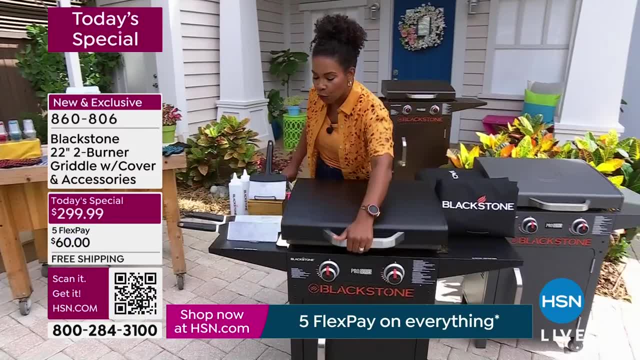 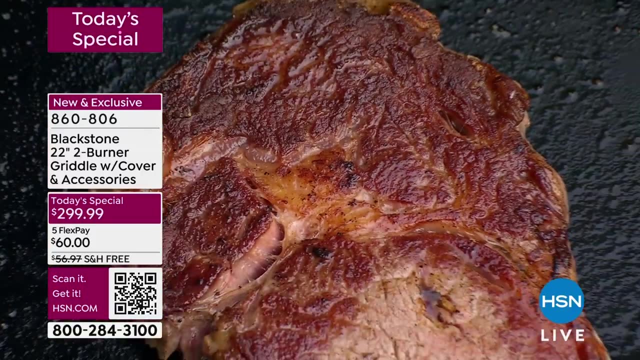 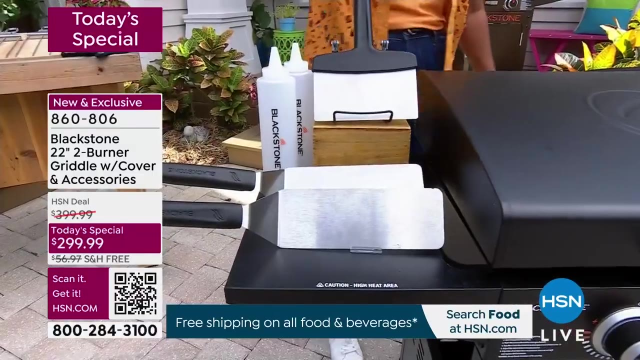 nice and taken care of on either side of your griddle. You're going to see you've got side table, So this is where you can do your prep. You can put food. when it's all done cooking, You can put all your condiments, any and everything that you need. What you're also going to get are these two stainless steel spatulas, And these are the one. These are the big, the long ones. So when you're doing steaks like that, when you're doing burgers, when you're doing eggs and potatoes and sausage and peppers, 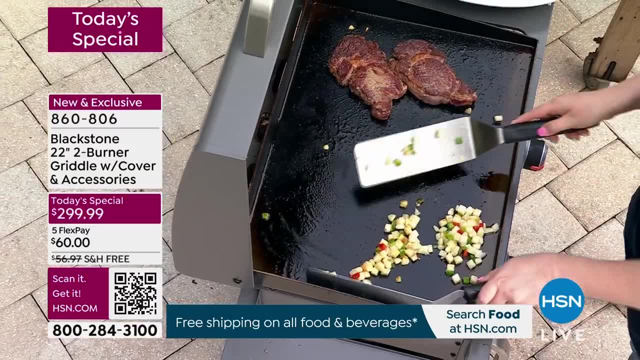 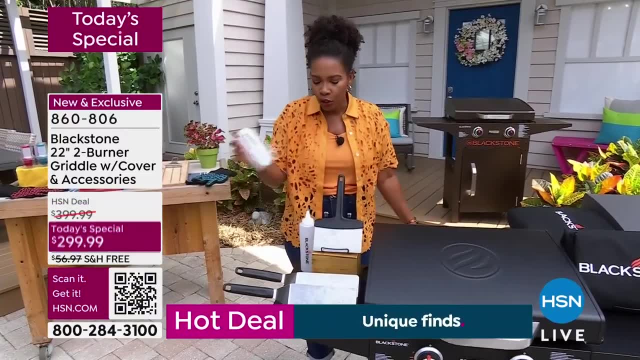 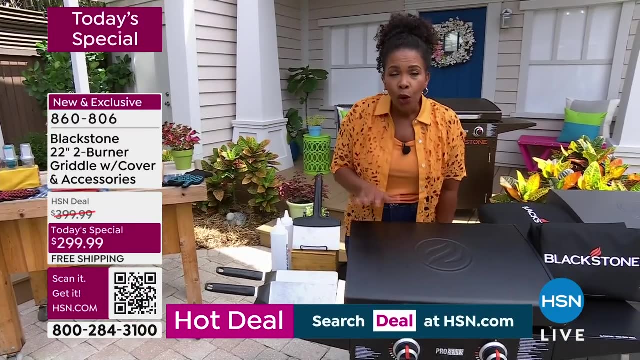 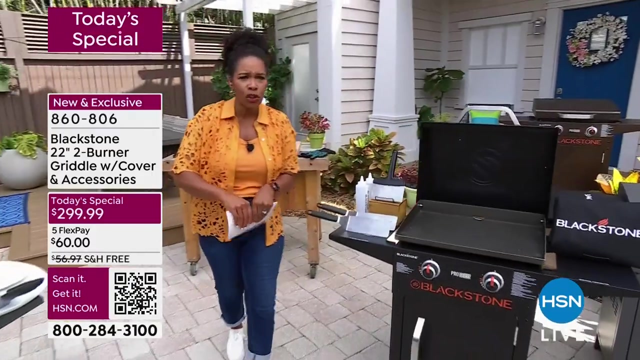 You've got two of the stainless steel spatulas. You're also going to get two of the squeeze bottles. What are you going to put in here? Anything you want. You put water when you're cleaning the grill, You can put your olive oil. You can do lots of things with this. This is your scraper and this is your best friend, because this is how you clean the grill And it's very simple. when you scrape, I'm going to show you real quick and then you're going to see this in action. when you, when you're done cooking and you want to scrape that grill, You take this scraper. you scrape everything to this little area right here. 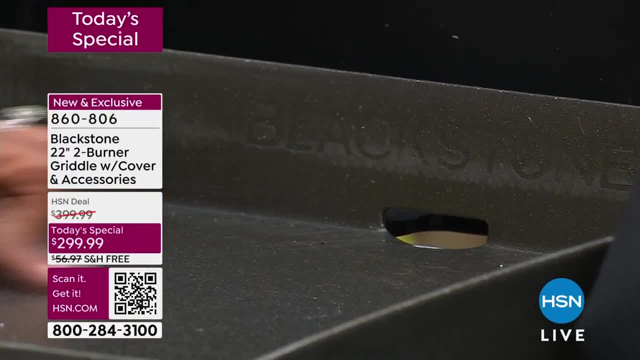 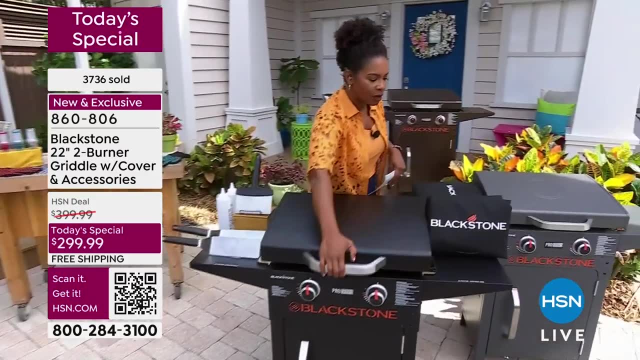 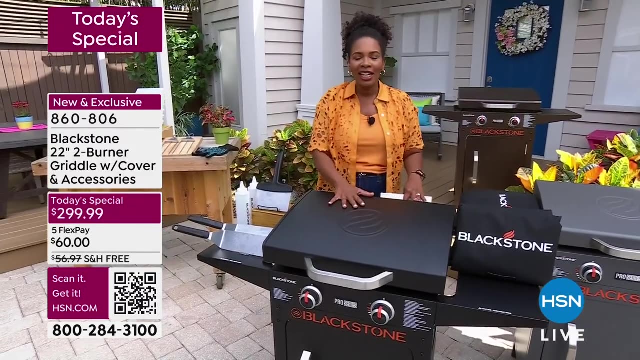 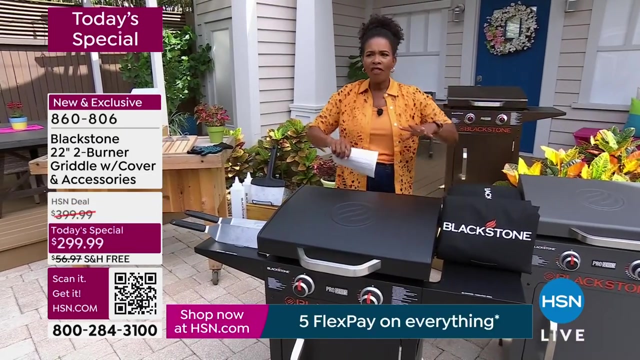 Because that's where all of the extra- you know the burn pieces- they fall right into that area and then you just collect them and throw them away. Really simple. I'm going to close this down and share that. you also get a cover for the grill, So the griddle. So when you're not using it, you're probably going to be using it, probably a couple times a week once you get it home, But on those days that you're not using it, you've got a really nice cover so that it stays nice and protected. This is from Blackstone and this is the one the 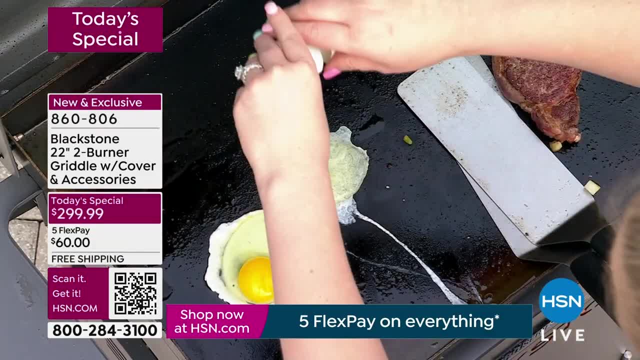 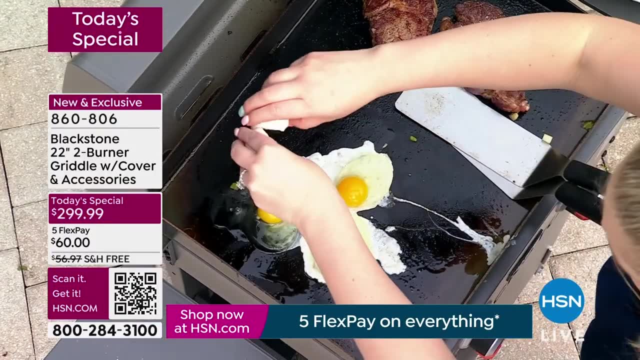 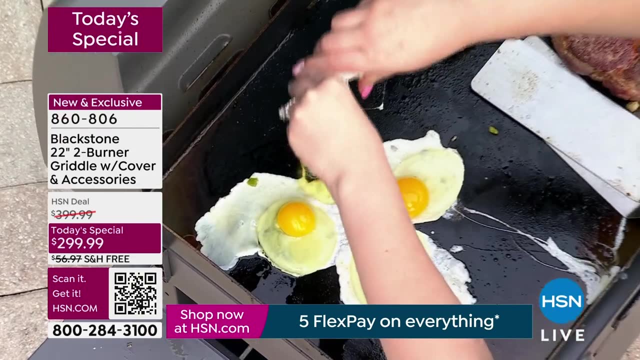 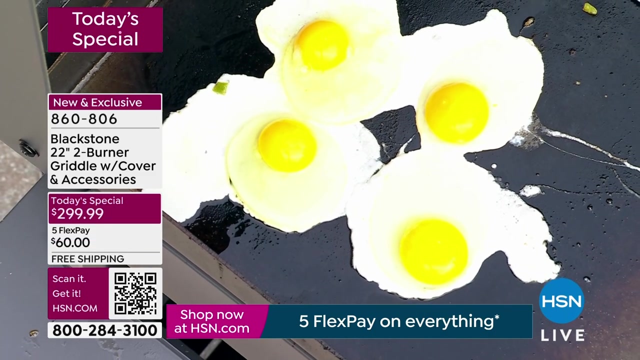 first Blackstone today special that we've had and the only one we're going to have this entire year, and just in time for outdoor cooking season. Now know that we took one hundred dollars off the price. Know that we've got it for you on free shipping, So it's a great savings right there And you're going to get restaurant quality style cooking every time you cook. Taylor Mock is joining us. Taylor, look at you. You started without us. I know that's OK. You know because 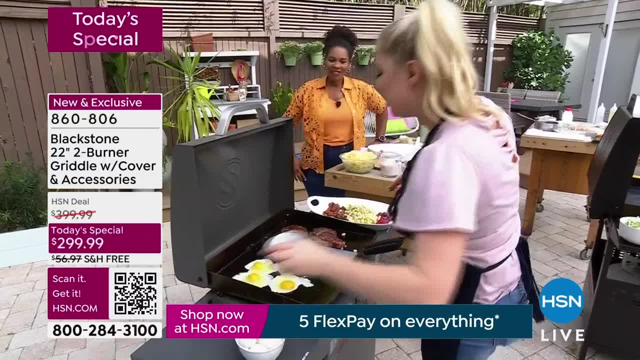 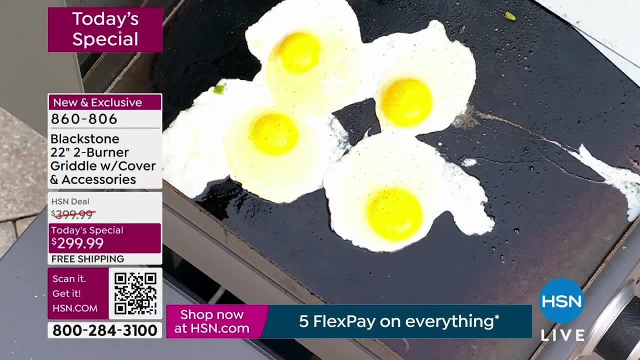 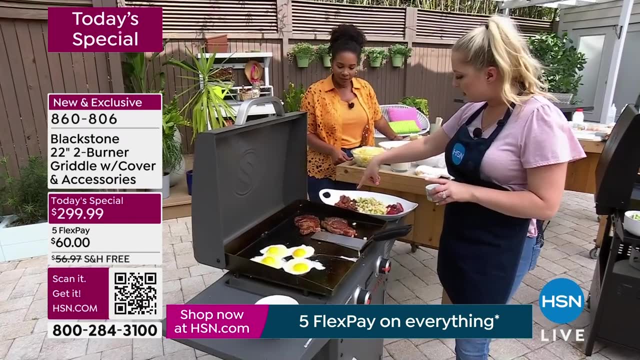 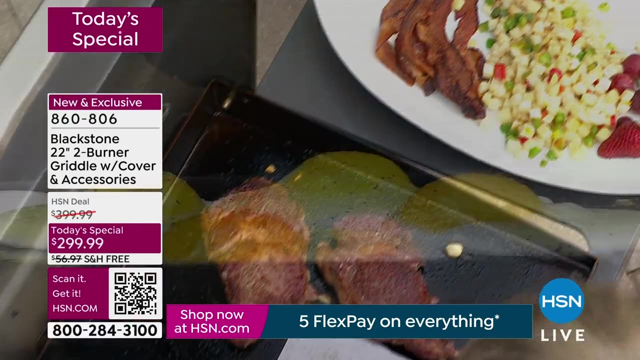 it's so quick, It is so simple, It puts out the best food. I said: you know what Tamara is busy over there. I'm going to get to go, I'm going to get to cooking. And in that moment of time they were just telling everybody: those colors, I have made hash brown potatoes with peppers and onions, Nice bacon, Those are about six, seven pieces of bacon. I've got steak sizzling. Those are Curtis Stone, Delicious, delicious. And then I've got the eggs, four eggs here. So you know, you said it best. This is, this is for anybody. 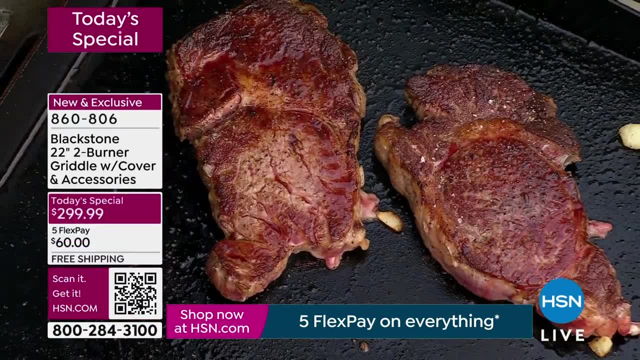 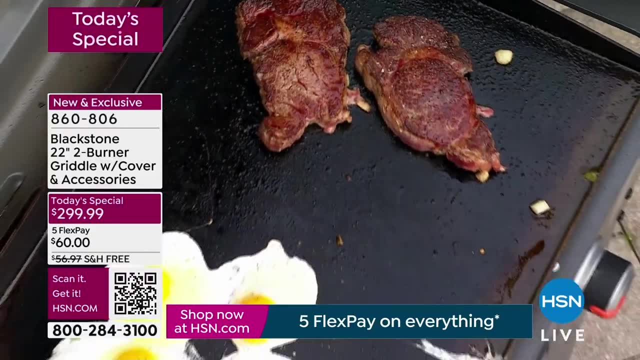 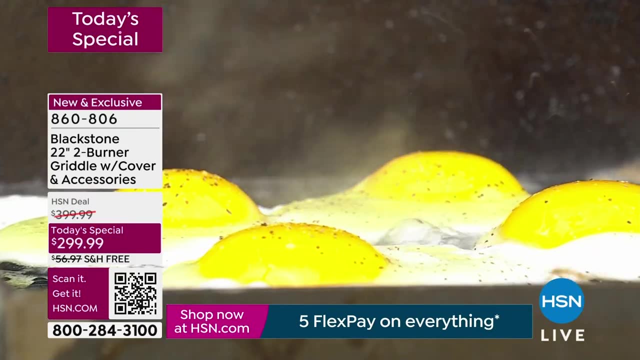 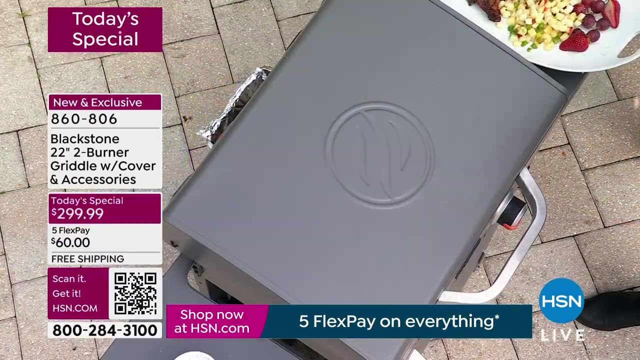 everybody. This is easy. This is truly something that I'm so grateful I came across two years ago. Yes, Because it's made me so confident in my kitchen and outside of my kitchen. Yeah, And what I mean by that is because my confidence on the Blackstone, I can now cook with more confidence. inside, too, I really can, because I'm like: well, I know I can make all that on my Blackstone, So I should, I should be able to make this inside. You know what I mean. The Blackstone is easy. This is not 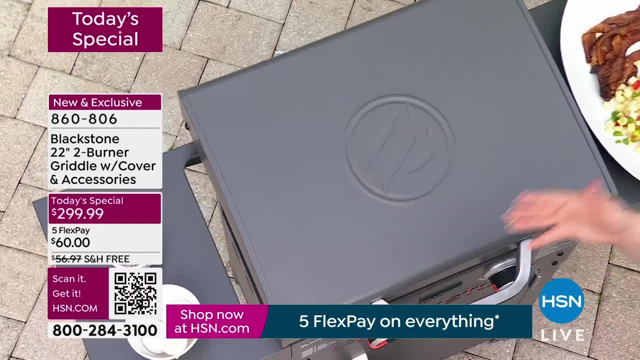 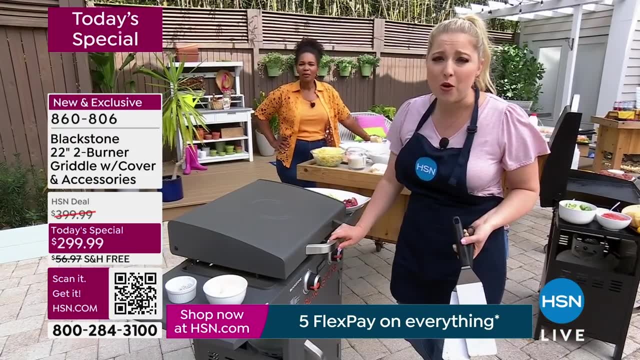 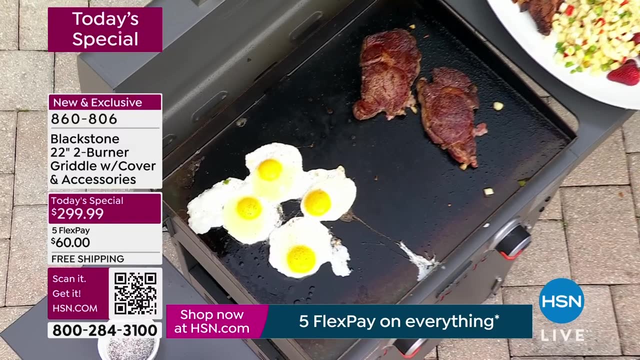 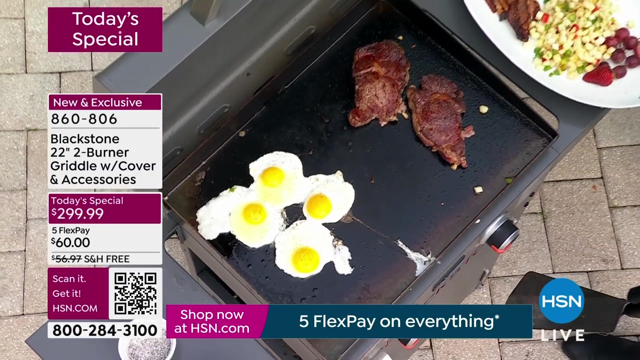 complicated. This is from for anybody. truly. We have 10 year olds cooking on the Blackstone with their moms and dads learning how to cook. Yeah, So we have 95 year old customers who say: you know what? this makes me feel comfortable. There is no open flames that I have to be prepared for, that kickback. This is safe, This is sturdy. Most importantly, Tamara, it's easy cleanup and, really most importantly, it gives the best taste ever. It's the kind of cook surface that you wish you had space to cook on. 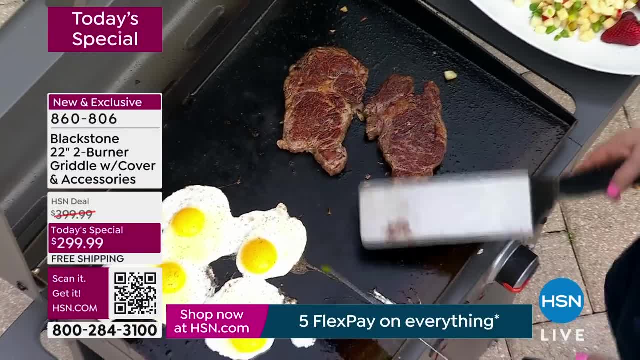 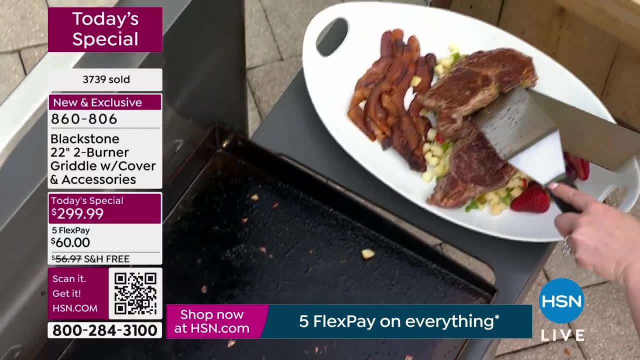 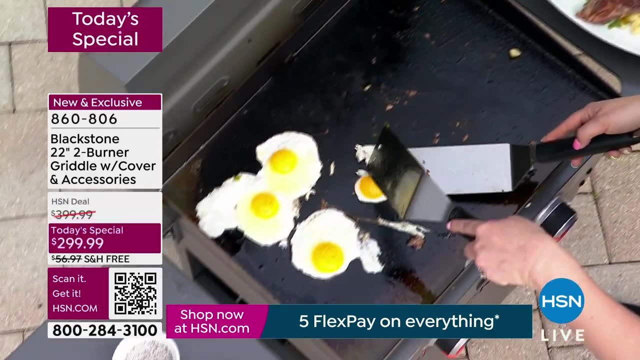 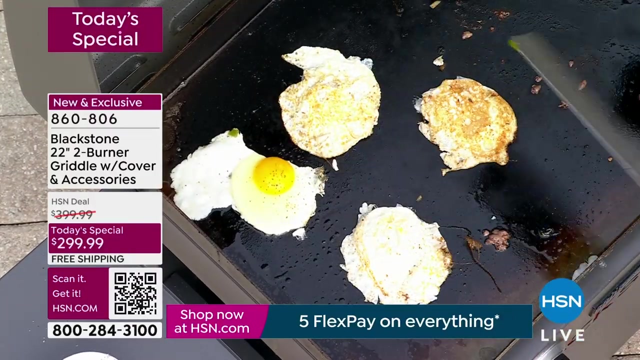 It's the kind of cook surface that you wish you had space for on the inside, Yeah, But you don't. You wish you had a you know one nice griddle inside, But most of us do not have space like this. But now you've got it outside So you could actually cook the entire meal all at the same time, Oh, without having to do. Well, I have to do this part first and then, Oh, and then I try to keep it warm. Totally, You don't have to do that with this. Well, what about the separate uses of pans you're using inside? You've got the pan for the eggs, the pan for the 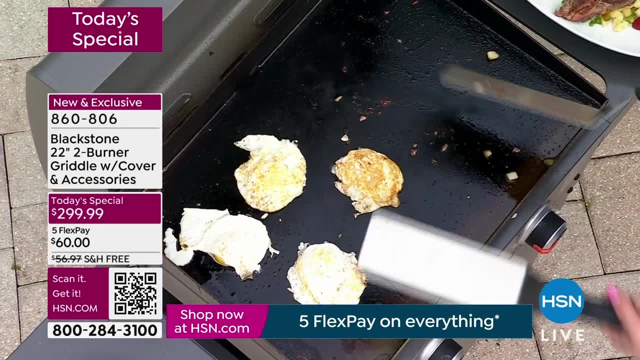 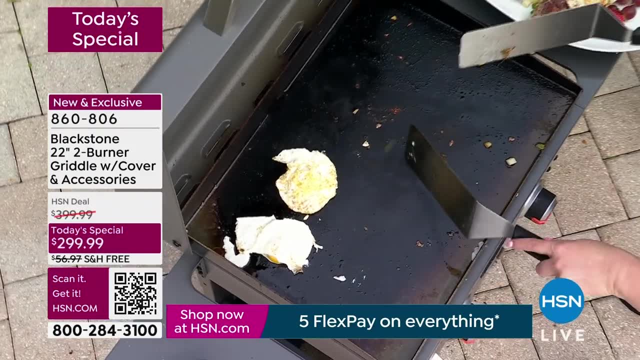 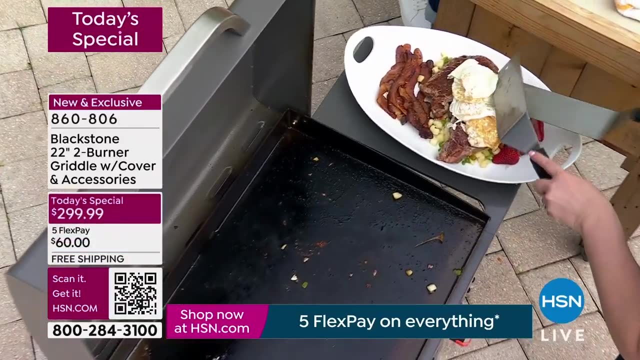 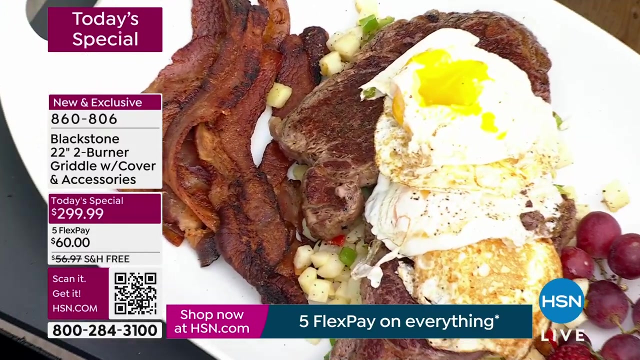 steak, the pan for the bacon, the pan for the potatoes- I mean, I can make a song out of it. There's so many pots and pans that you're using. That's right. And look at me, I'm only showcasing one unit, one cold rolled, beautiful steel. Yes, That's going to stand the test of time. Look at that steak and eggs and bacon and pop on this egg. So pretty, Get in there. Don't you love to have breakfast like this in the morning, In a matter of minutes, Yes, In a matter of minutes, Without having to go out. 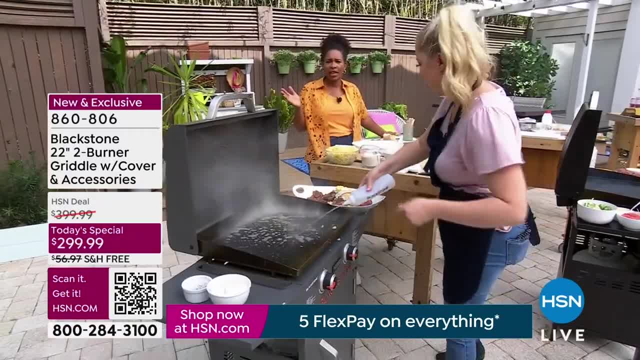 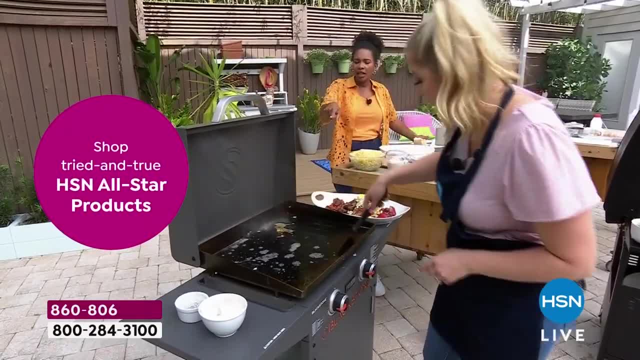 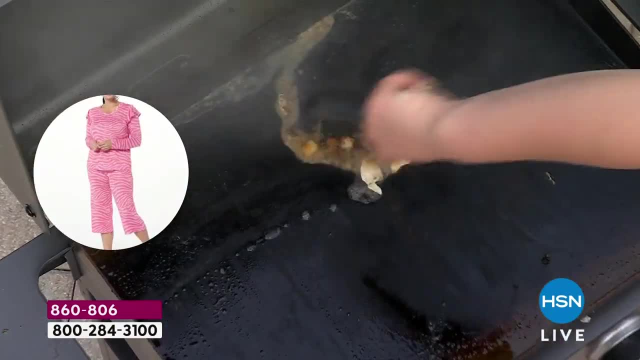 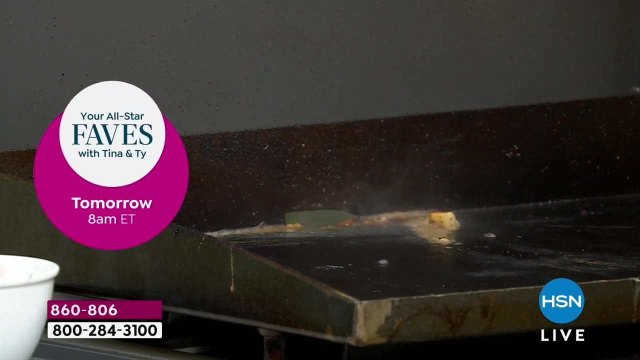 and order it and hope they make your eggs right and hope they make your steak to the temperature that you to your liking. Now you can actually do it at home And then, when you're done, This is it. That's water, and you scrape and water and a scrape And that is it. There's no having to wash it with soap. Think of it as your grandmother's cast iron skillet. You're not going to want to wash that with soap, Right? How do you take care of it? You rinse it off with water. You want to cook it? You're cooking on high heat, So you're killing a lot of those things. 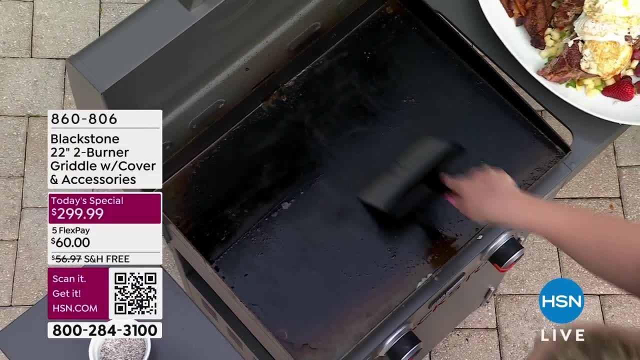 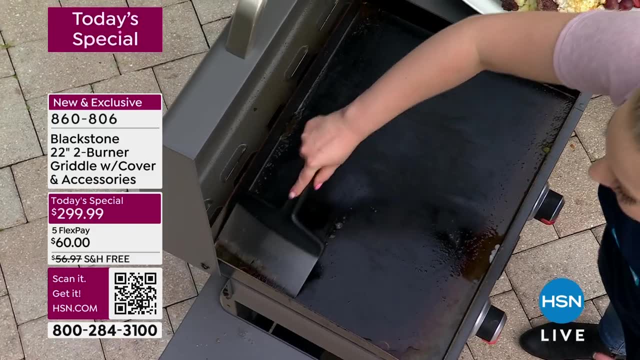 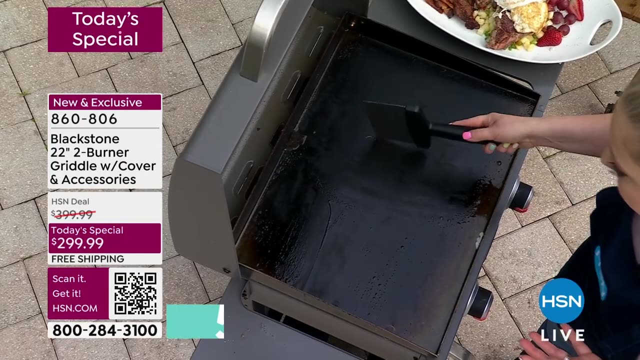 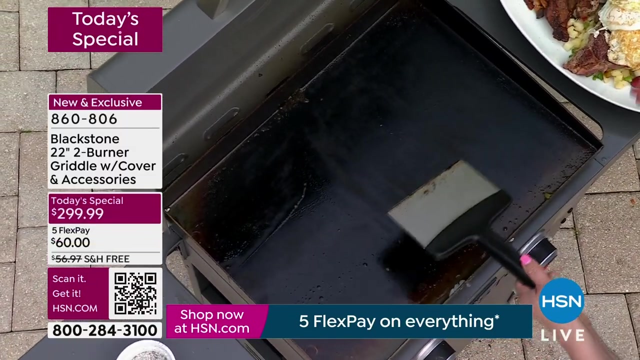 But then you want to rinse it with water And then after that you want to protect it by adding some more oil to it. You want to keep it coated with oil, because when you coat it with oil, that is what's concealing and locking in the moisture and the flavor. Cold rolled steel will stand the test of time. This baby, it's not going anywhere. No, There's a reason why we give you these metal spatulas to chime on here. There's no denting of any sort. You can. actually, if you really wanted to, Tamara, you could cut a steak on here. Wow. 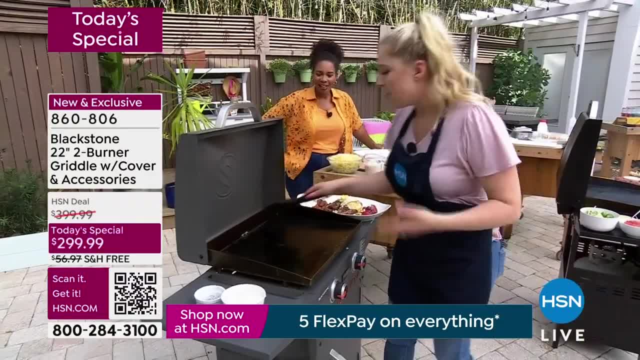 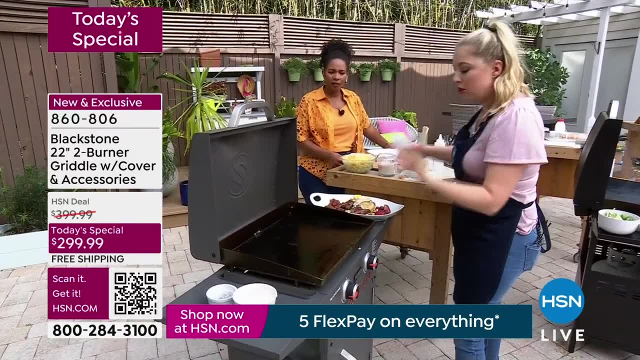 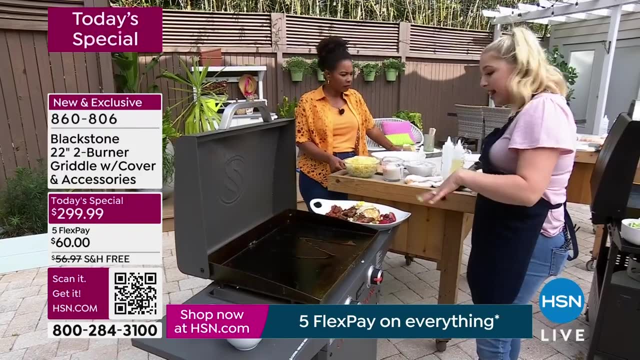 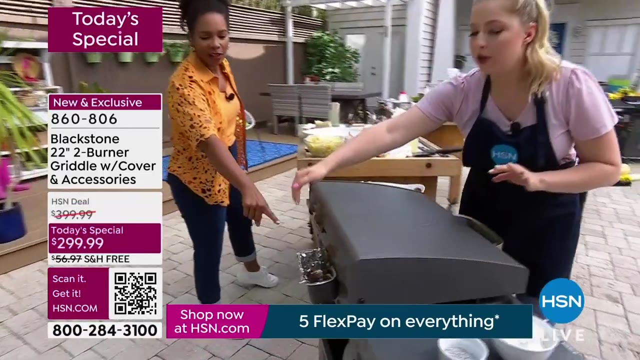 You've seen that at your famous hibachi places, right? Yes, Where they cut the steak and things like that. If you really wanted to, you absolutely could. I just want to say that because that's how hearty and the most incredible material this really is. And you're always cooking with oil, right? Add your oil. I'm always cooking with oil and then, just, you know, let it, let it marinate. You can spread it out. I love to show the back of the unit here, OK, Because this is where the goodies go. This is my cleanup is really throwing this away. This is 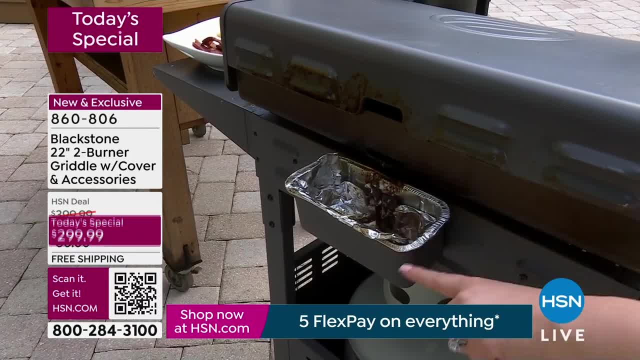 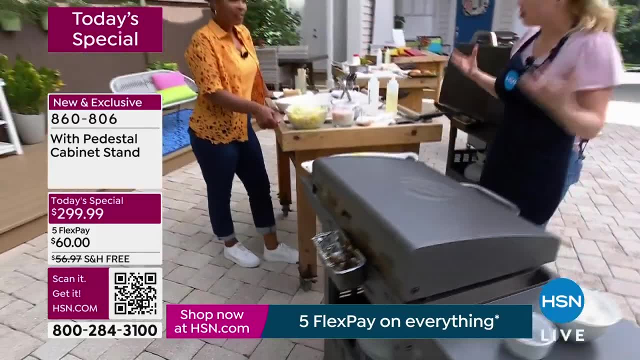 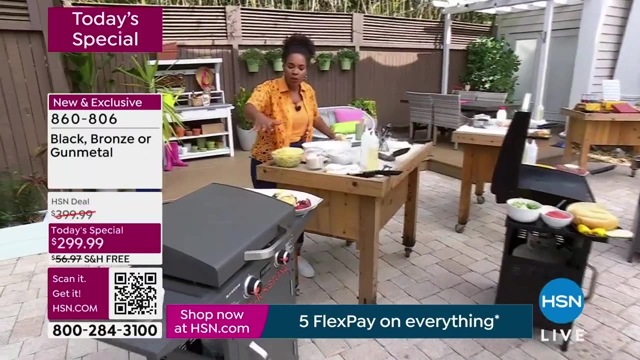 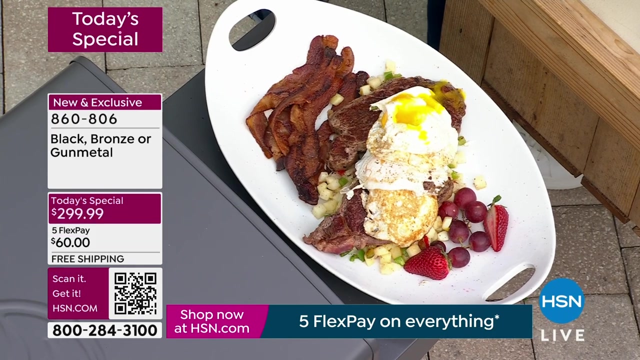 you know you can do two different things. You put tinfoil in the back, or you can buy those aluminum disposable pans- Yes, Those liners. I've seen them at gas stations, I mean. you can get them anywhere, Big box stores. You can buy hundreds of them for dollars. So that is your cleanup. Sign me up And look at this. You made enough. This could be bread, This could really be any meal, But you made enough breakfast for dinner or whatever you want, The entire family all at the same time. Nobody's cooking. Nobody's eating first, Nobody's eating. 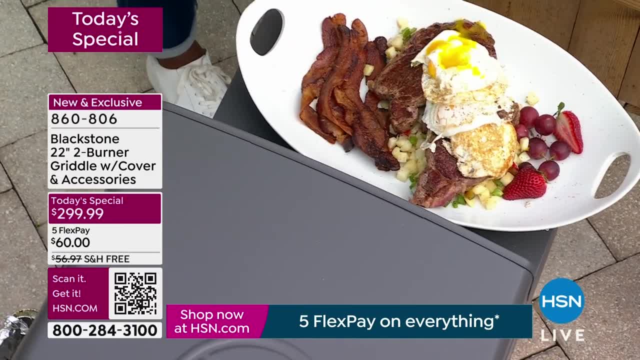 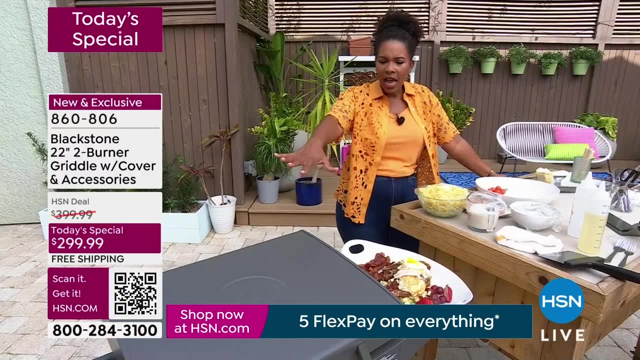 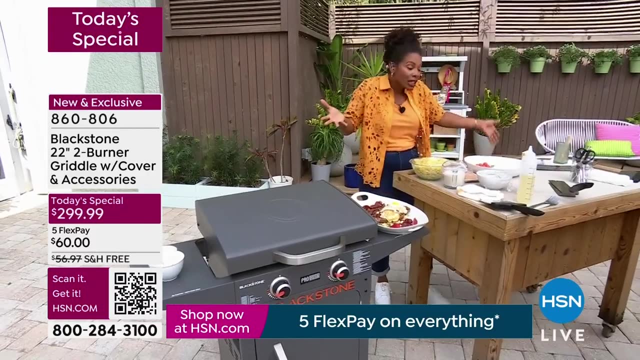 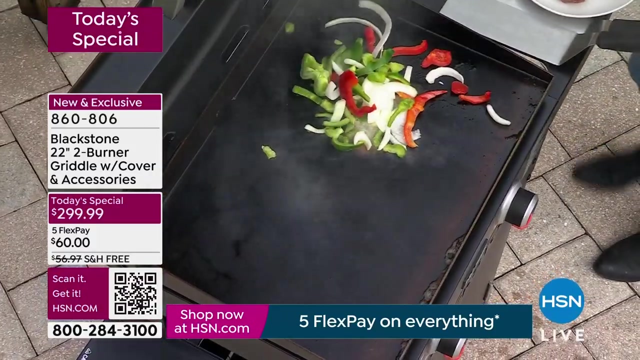 cold eggs, because it's all done together, because you saw Taylor do this right here on your griddle- And I say your griddle because I want you to get it home- This one is the gunmetal color. We're going to move to the black when there's also a bronze color, But they're all good And, like I say, just in time for outdoor cooking season, We want to be out, We want to be enjoying the weather as much as we can. Oh, it's a beautiful day today too, And Taylor, like this is the deal. Taylor's a pro when it comes to cooking, when it comes to. 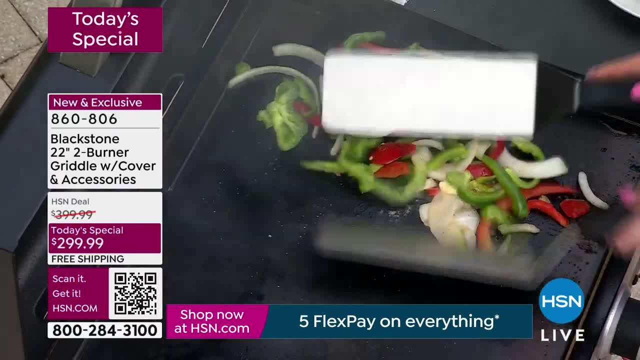 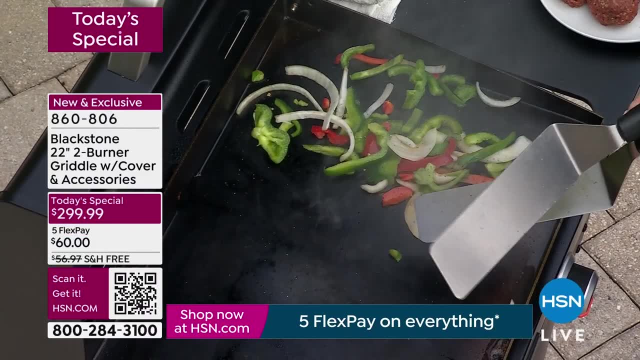 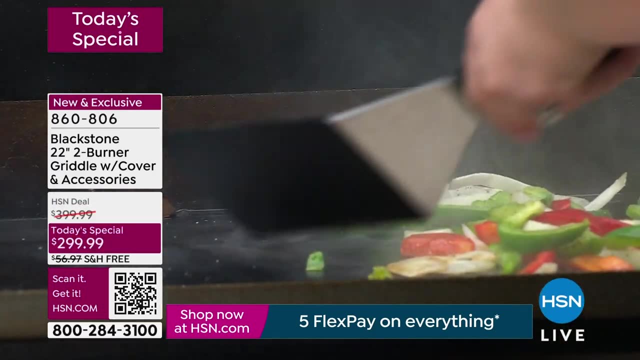 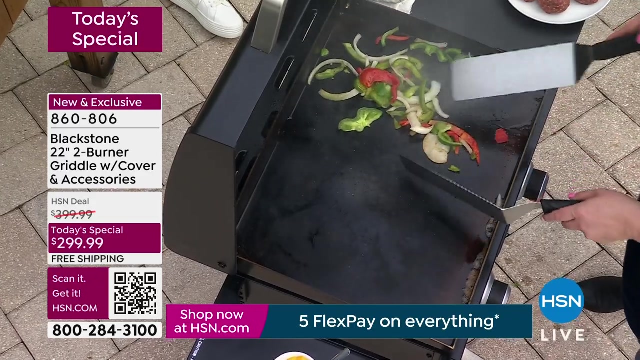 teaching us how to cook, But you don't have to be intimidated with No, not at all. And honestly, Tamara, I love you for saying that. She's making me feel so good. I'm actually. I'm not a pro, I am. I'm a home cook, I love to cook for my family And I love the black stone. So if this makes me look like a pro on here- and I am proud of that, because anybody can do this, Yeah, Body can do this, And I've repeated that so many times because when you get it home, you will see. 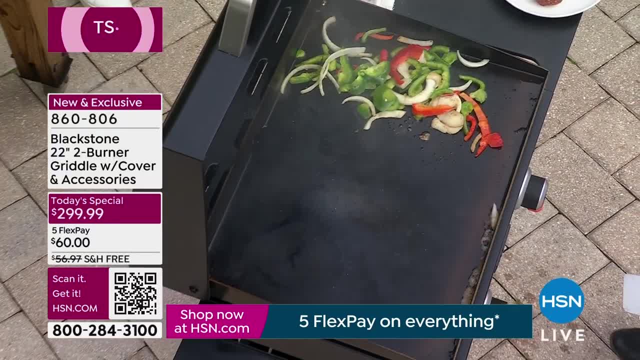 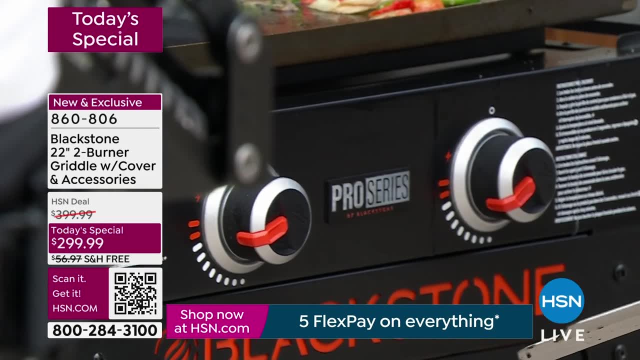 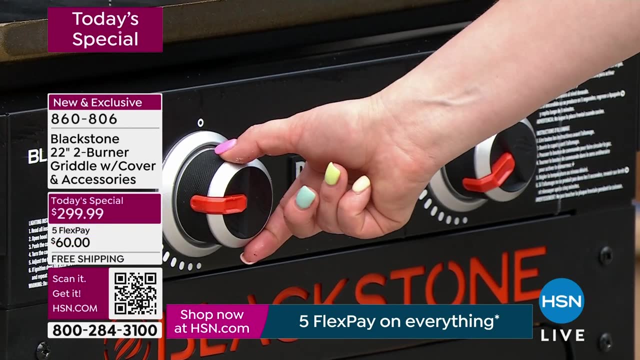 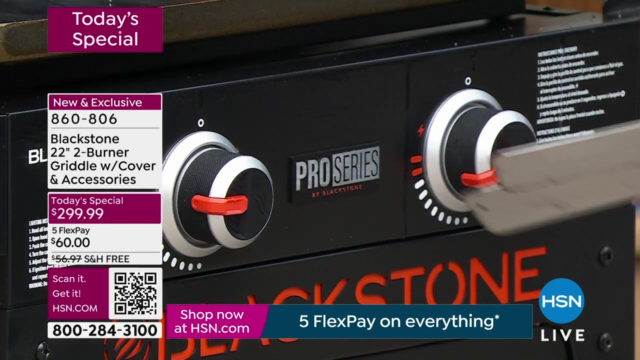 exactly what I mean. Now I want to talk about the two burners here. Tamara, Yeah, And I know you talked about this earlier, but you have two sides of your unit. here We have what's called H burners. OK, Each side is going to house its own heating method, So what that means is: on here I'm going to crank this to high because I'm about to make smash burgers over here. I have this on medium high because I'm cooking my veggies, So I'm able to showcase two different meals My veggies are for. 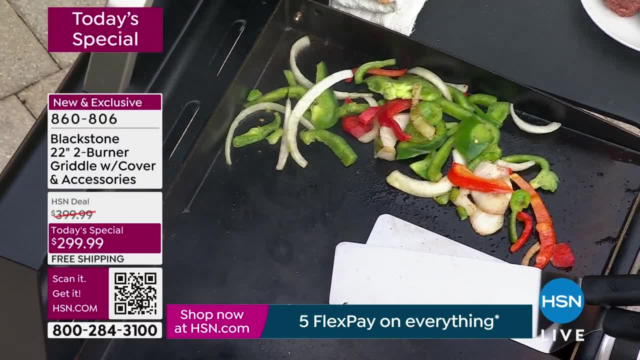 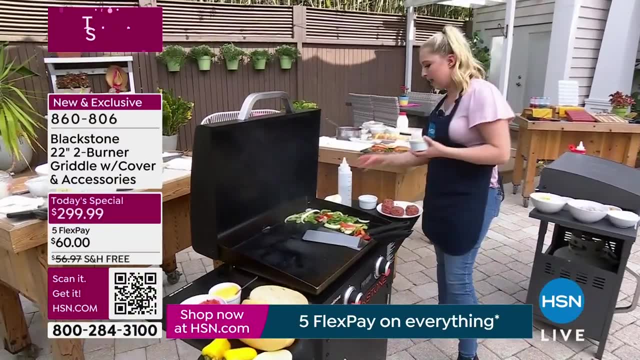 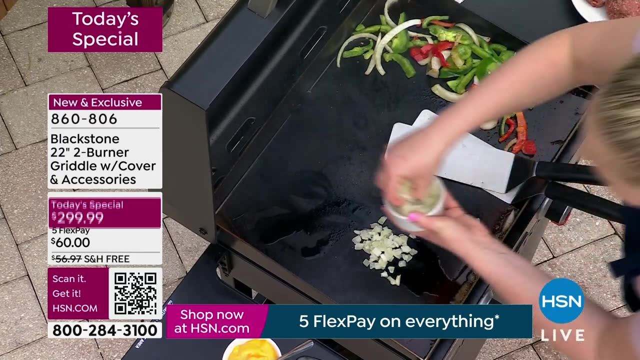 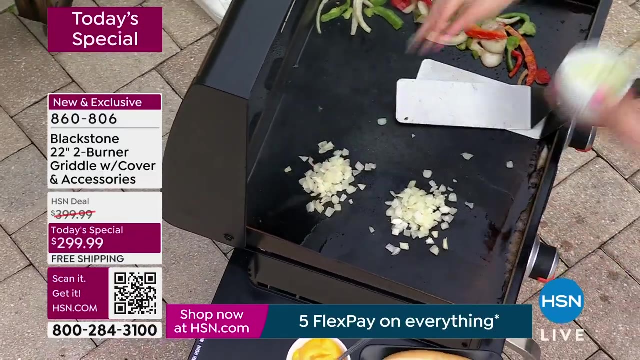 my Philly cheesesteak later. But I'm going to slap down some good old smash burgers And truly it's the best of the. Have you had a smash burger before? Surely you have, I have, but not in a long time. OK, I've got my mouth all ready for some smash burgers. You got your mouth all ready. I love this. I'm actually making Chicago style smash burgers. I do a little bit of chopped onions. Nothing's better than a good caramelized caramelized, however you want to say it. Pardon my crunch. I'm eating bacon, The crunch. Can I put the bacon on the smash burger? 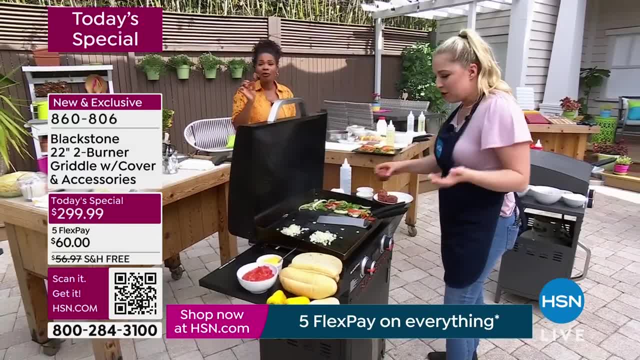 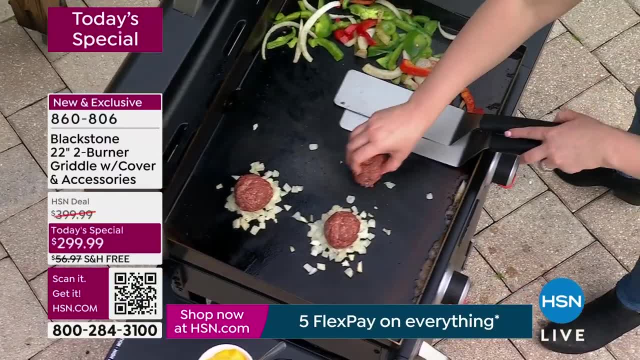 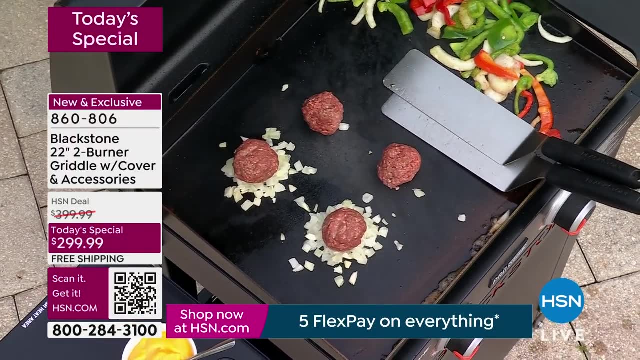 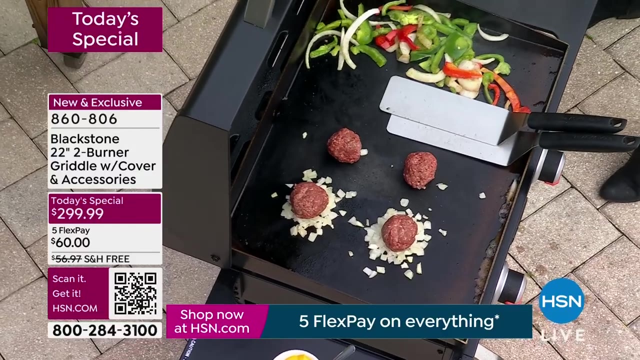 I mean, I put the egg on the smash burger, Why not? Oh, you sure, Here, Listen, I, you. That's the joy of this is you can do anything. I've got 80- 20 beef here. But if you wanted to use turkey meat, if you wanted to do ground chicken- and maybe you have an allergy to something, maybe your tofu, you're vegan, Those are. That's what's so wonderful and spectacular about this. I'm actually going to show you a little trick camera. OK, Because I know you're getting your own blackstone. OK, You're going to take parchment paper. 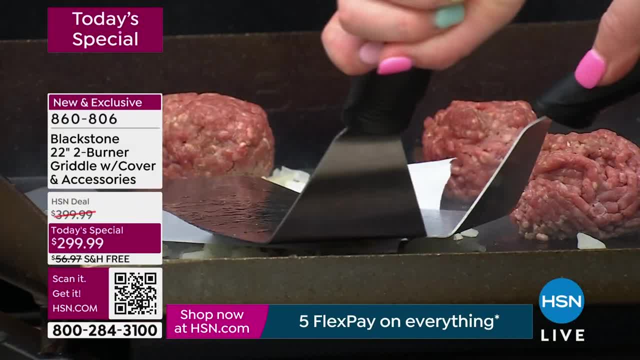 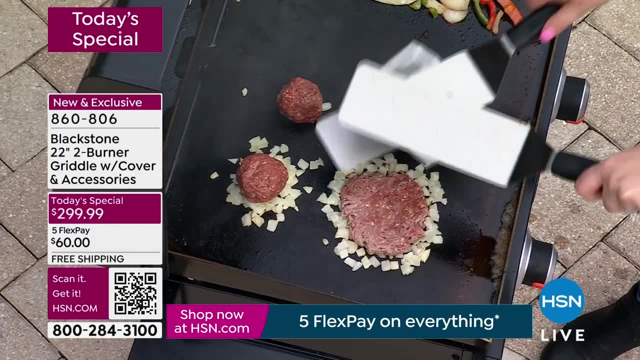 Yeah, You're going to put it right here And then you're gonna smash your burger. OK, I'm using parchment paper because it allows for the The spatula and not to stick to the meat. Would you see that? Oh, you just have fun smashing around If you want the kiddos or? 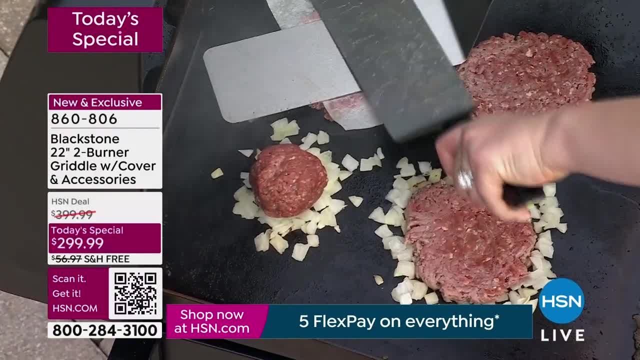 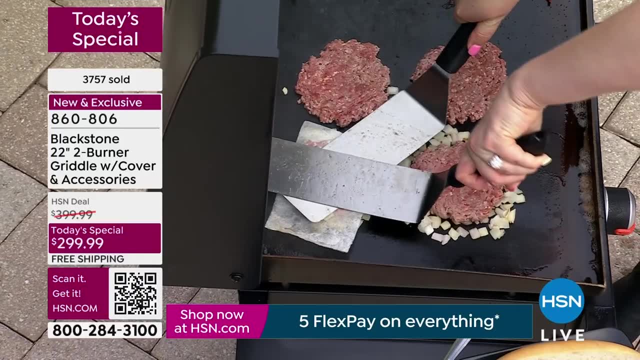 the grandbabies to do this part. They love this. Oh yeah, Not dangerous, They're just smashing it down. There's no open flame. you're not dodging flames when you're doing that Exactly, And then that's it. That's all you do now with a最後. 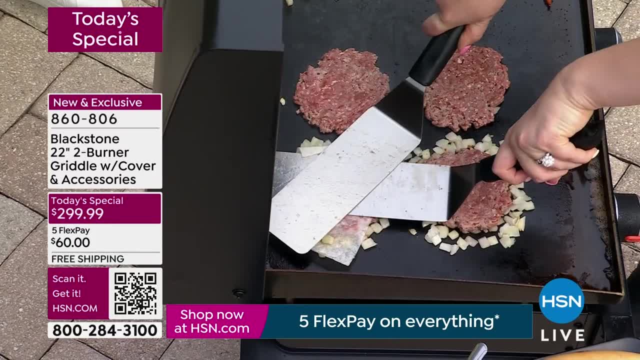 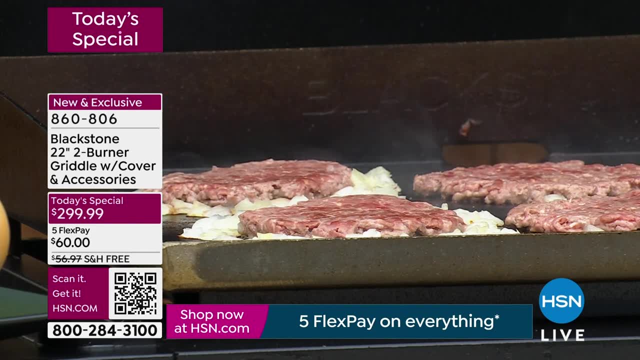 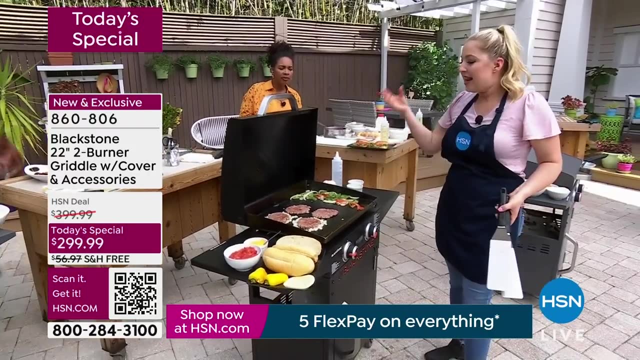 Burger. what makes a smash burgers so delicious when you go to those popular drive-through places that you know we love to go to? what makes it so delicious? what makes it delicious is the griddle, it's the flavoring, the thousands and thousands of burgers they've cooked over time and it houses and it locks in those flavors. this is a. 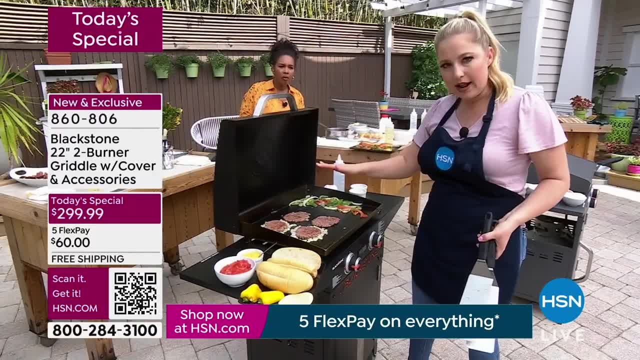 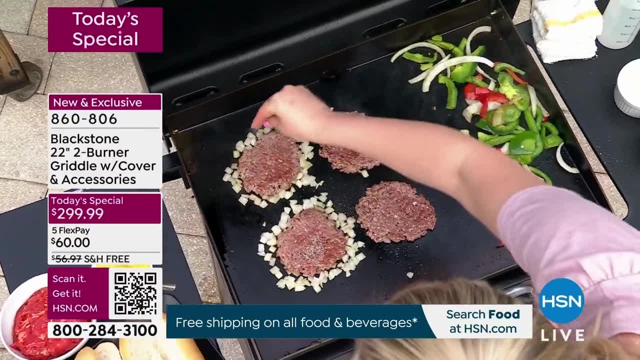 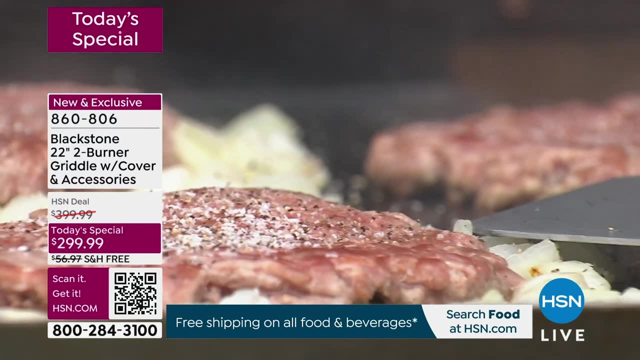 memory card. so when you cook and cook and cook on it, the flavors are only gonna get better, right? oh, that's why- and it's nice and crispy, and there's a little trick- you want to make sure and add your salt and pepper once you smash it down. also, you want it as thin, I mean thin, thin, thin as you possibly can. and 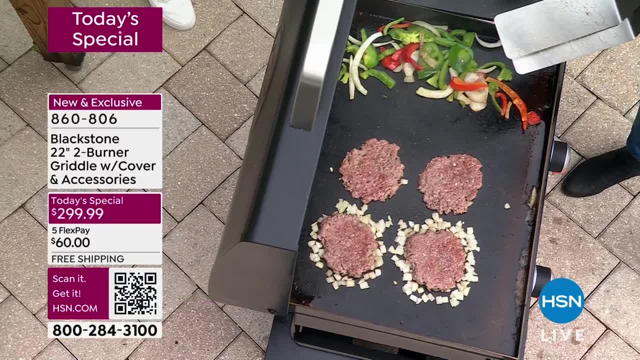 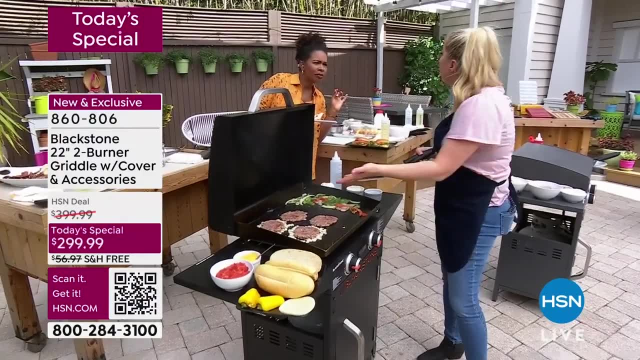 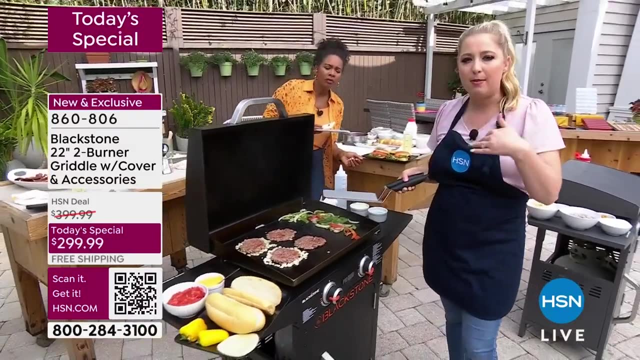 you almost want it burnt like crispy, crispy edges, because that's what makes it so delicious when you go to those popular fast-food places. now you're talking guilt. yeah, no guilt, because I know I'm not putting a bunch of extra lard in it, I'm not putting a bunch of extra fats in it and oils, I'm in. 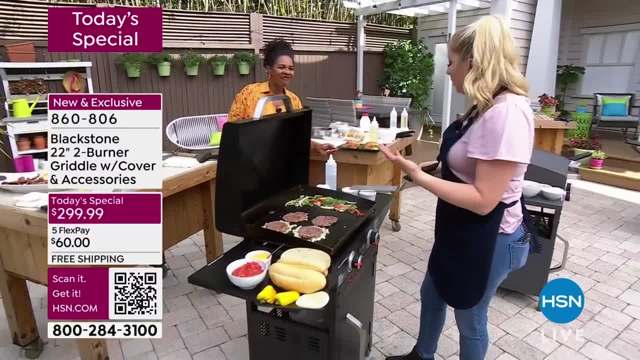 control. I'm not putting a bunch of extra fats in it and oils. I'm in control, that's whether I'm using avocado oil or a healthier oil. you can totally do that and you're doing it at home when you want it, when you have a taste for you. 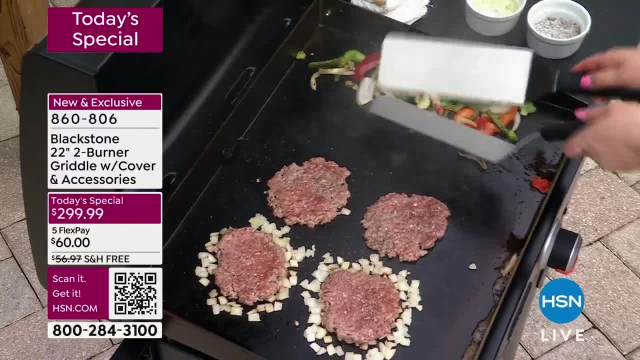 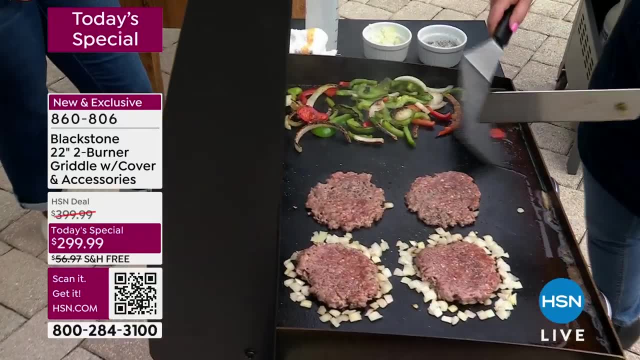 know, yeah, and it's your. you know, and that's the thing. like you said, the more you use it, it's gonna have your seasonings, your flavors are in, entwined into the griddle, yep, so that even if you have a good burger somewhere else, uh-huh. 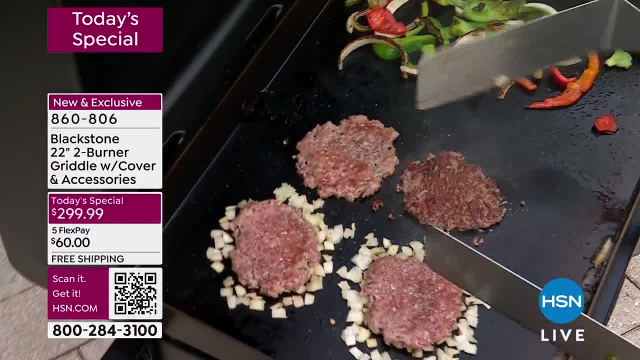 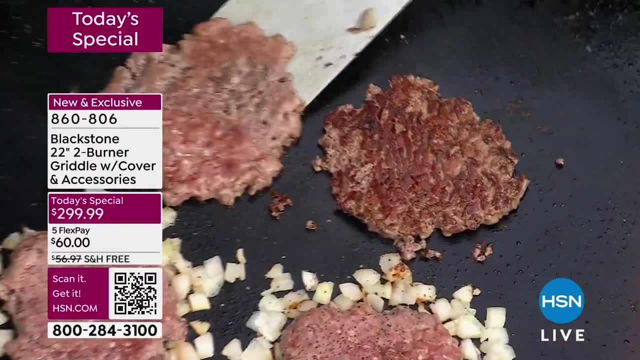 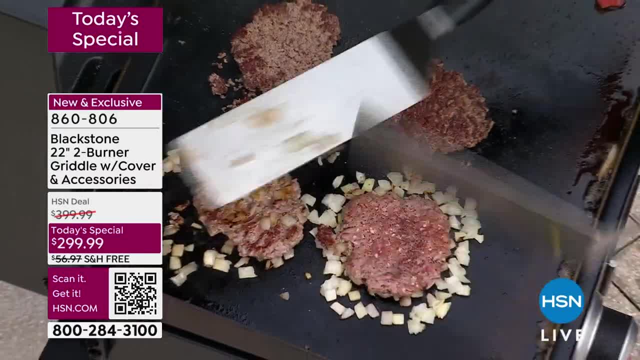 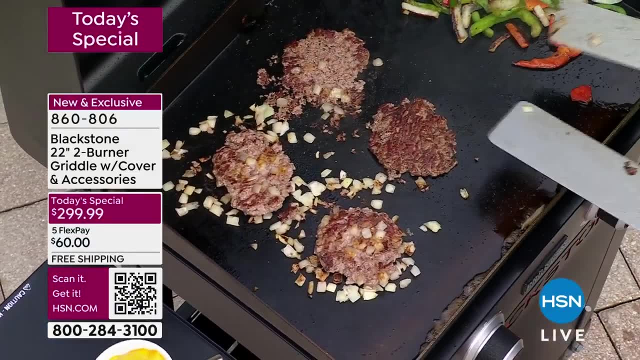 do you want a lattice burger? so that one didn't, here we go. this one's better, it's got the, and then, once this cooks down, on both sides again you're gonna add your cheese and then we're gonna stack it and this is an absolutely quick, incredible. 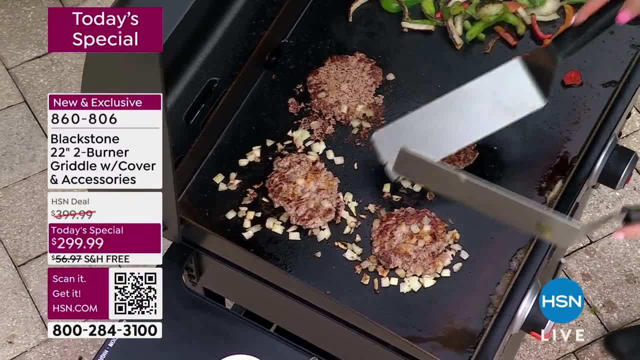 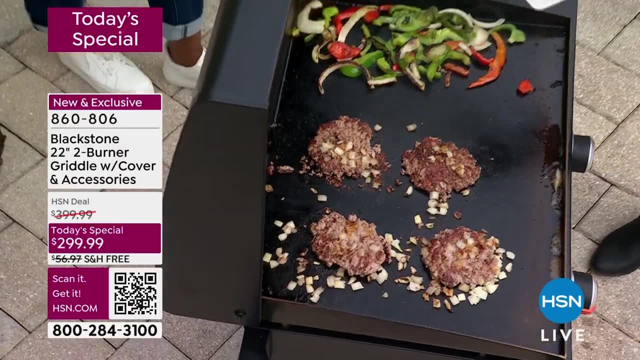 meal, whether it's Father's Day barbecuing, maybe it's a quick Mother's Day brunch, maybe it's after church on a Sunday and you know all the grandbabies are over the family's over. you don't want to go to a restaurant, spend $300 for. 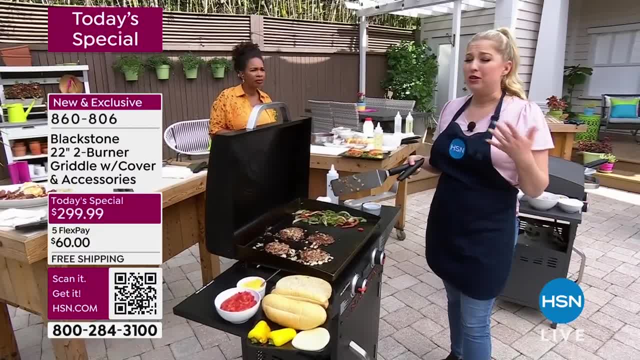 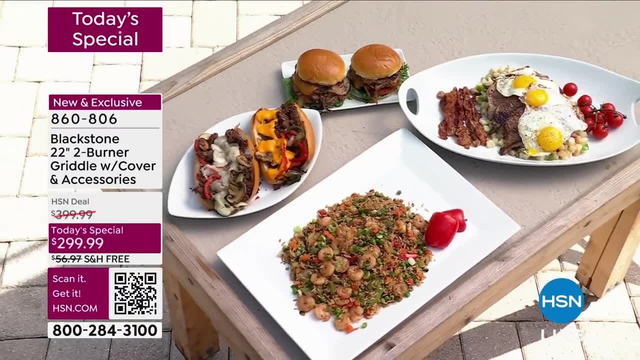 the whole family. yes, sit in the line and then most the time your food's not that great. no, your grandbabies are ready for a nap and you're like we got to get back. it's such a hassle. why is that to yourself? and you know what? because up. 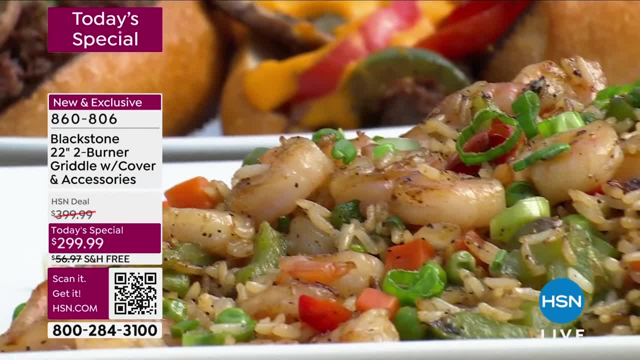 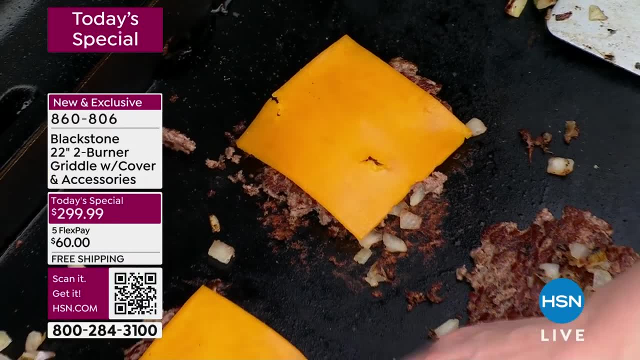 until now, we didn't really have a lot of options, but there's something special about seeing your food being cooked- yeah, because you see it's cooked with love- and seeing the person who's cooking it and giving you the food and saying, oh, I don't want cheese on mine. you're like: okay, no. 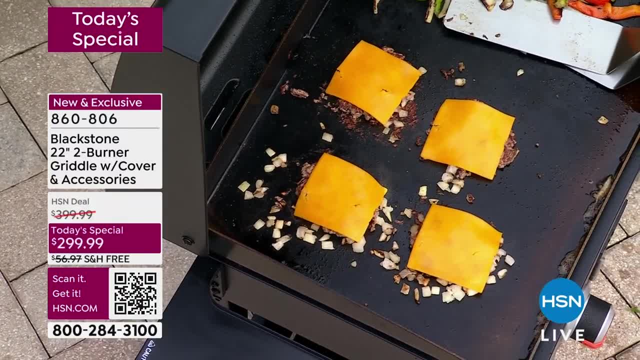 problem, yeah, and it's literally the beauty of it- made to order right in front of you when you have it at home. that's what I think, that's really what you're going to love about it, so I don't want you to save this for just special. 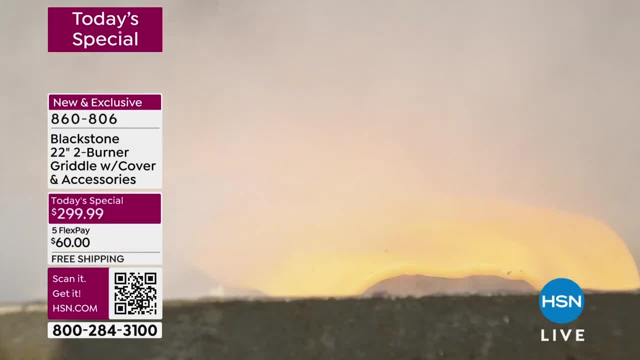 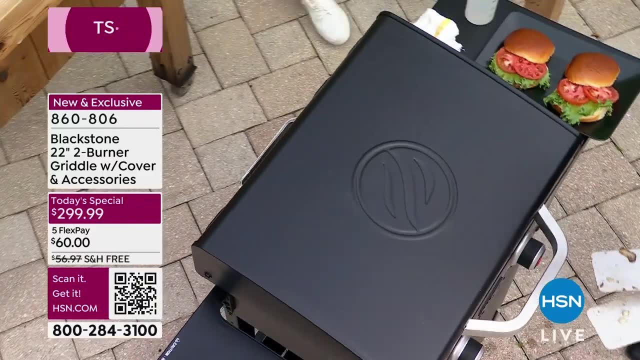 occasions like just fourth of July and those kinds of things. no, this is every. this is every day. girl, I'm on this thing all the time. I have disappeared in my actual kitchen. I'll go in there and make a salad, but this is my life. now is the. 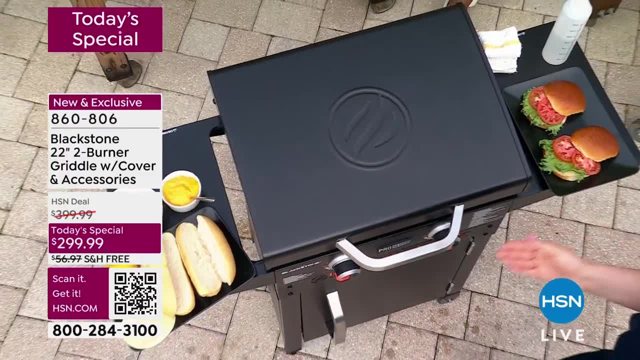 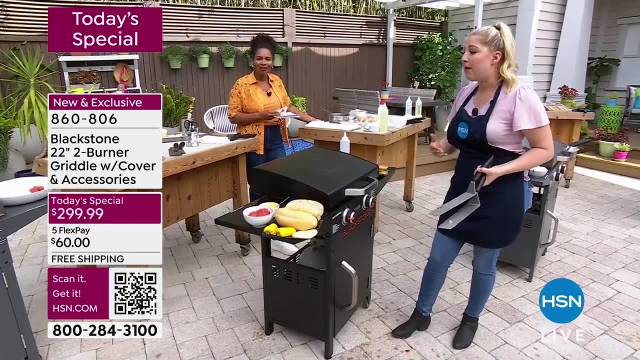 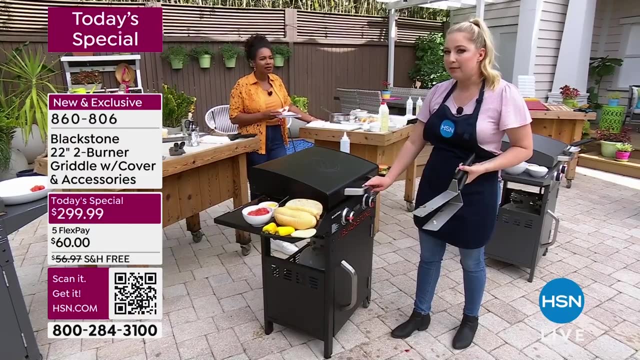 Blackstone, and it's because I've got a two-year-old little baby girl. she's she needs my attention, especially around dinnertime. I'm busy trying to feed her first, get her ready for her bath, also cook dinner for my husband, and I finish up the work from the day, so this has been such a time. 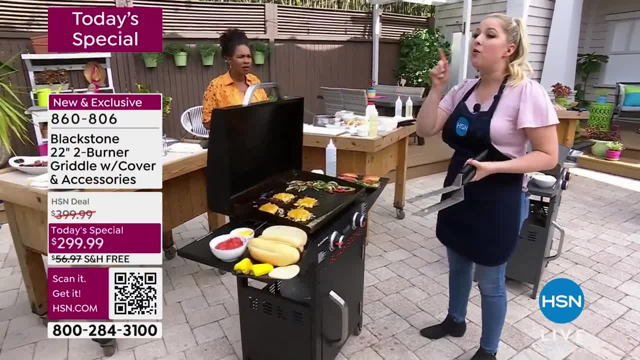 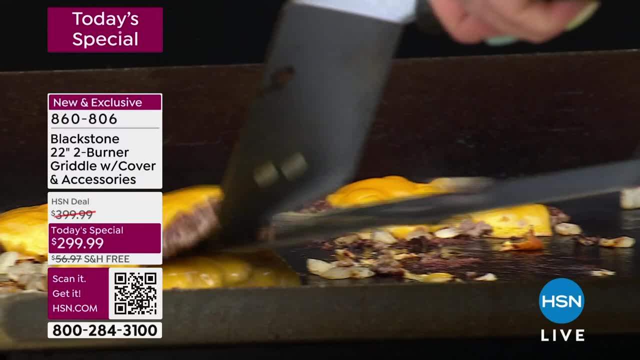 saver in my life, when I feel confident enough to say: honey, I will get these burgers done. probably, give me ten minutes. you go ahead, start feeding her her dinner. right, let me get these burgers done. yeah, so by the time we actually get inside to eat, it's ready to go. 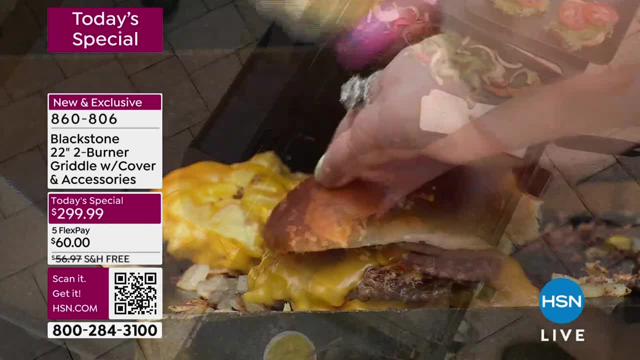 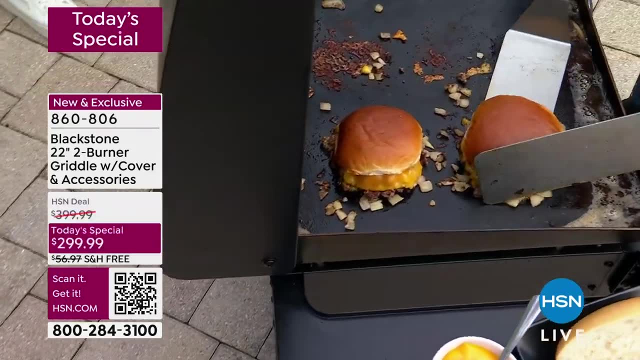 and think about that. you could get the burgers done, you could get the potatoes done at the same time. oh yeah, anything else that you wanted to put on it, absolutely, and they're all done at the same time. all done at the same time. and I'm still prepping for a cheesesteak on this side and think about it and then 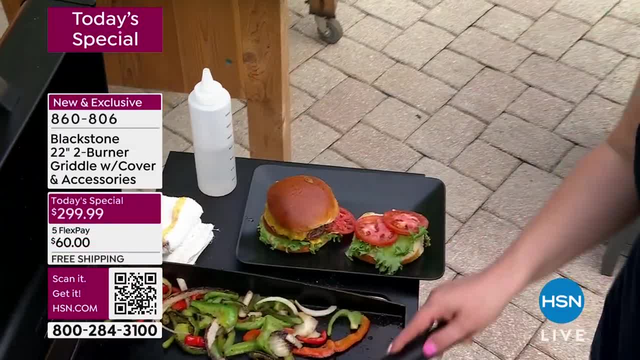 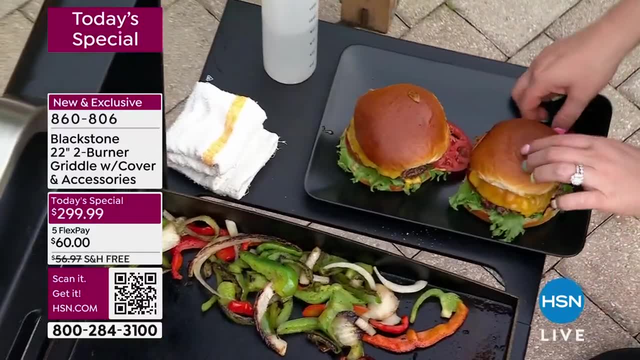 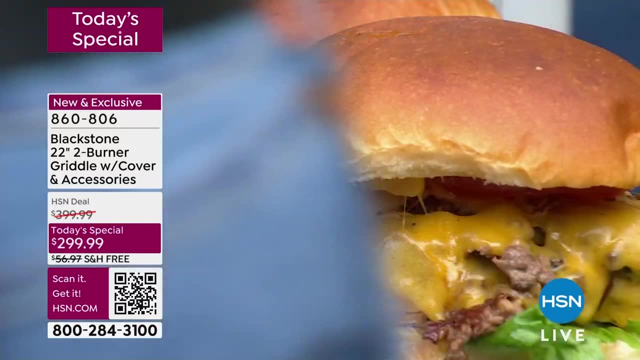 you're not having to stand in the kitchen for another 20-30 minutes, washing pot after pot, pan after pan, because you did it all on the griddle. well, it's funny because I've been saying this throughout the day. I said my husband, I'm gonna put tomato on here. my husband always says: honey, your foods delicious. 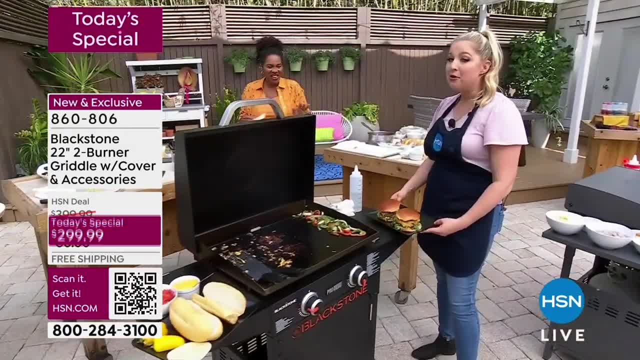 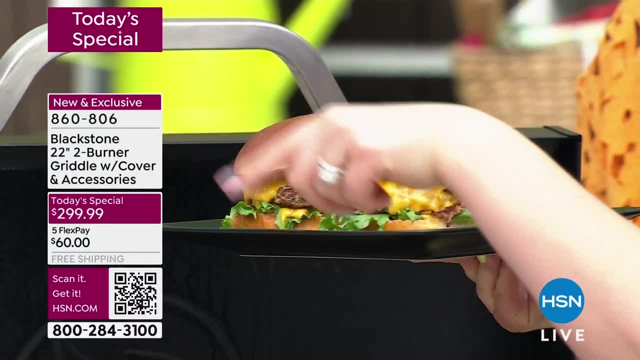 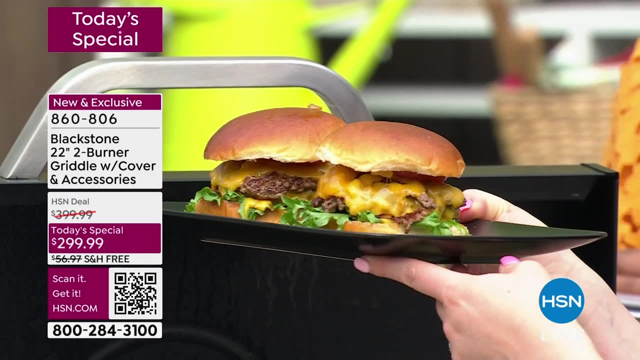 but now I got to do dishes and so he knows when I cook on the Blackstone there's no dishes. hey, you're cooking on the Blackstone tonight, right, it's easier for everybody. it takes the stress off, the pressure off. look at those burgers. and you know what, if you went out to a restaurant order that, how much would you? 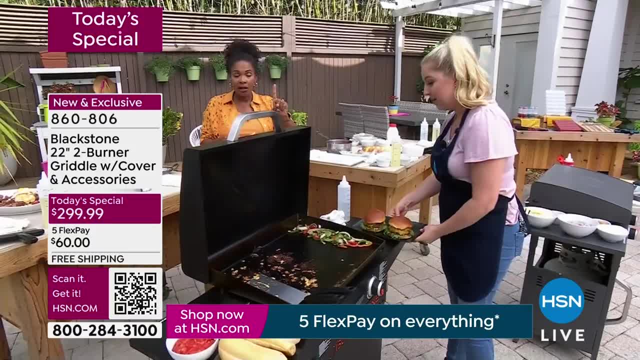 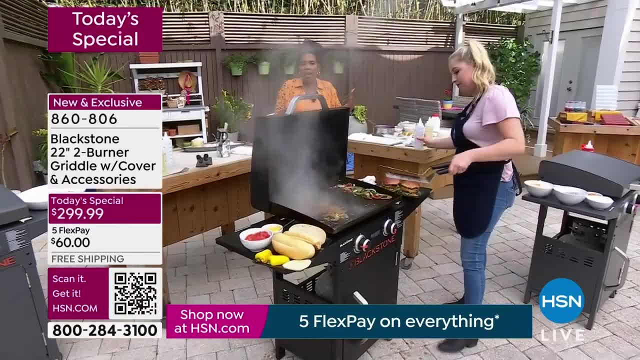 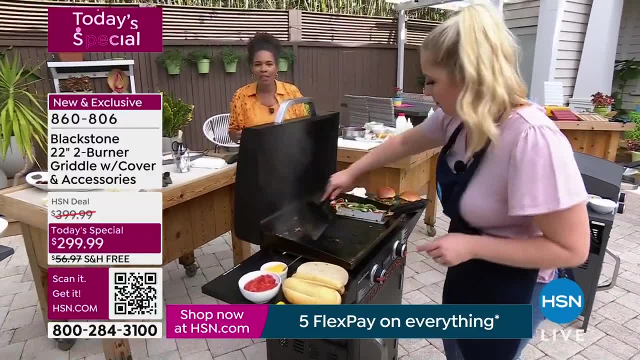 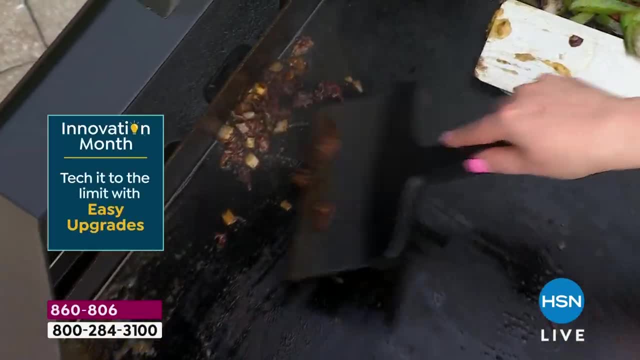 And you're using it once a week, couple times a week, every day. yes, different meals. it's completely up to you whether you want to do something real, fun and easy, like smash burgers, or whether you want to go a little bit fancier, like your steaks, your rib eyes or your stir fries. 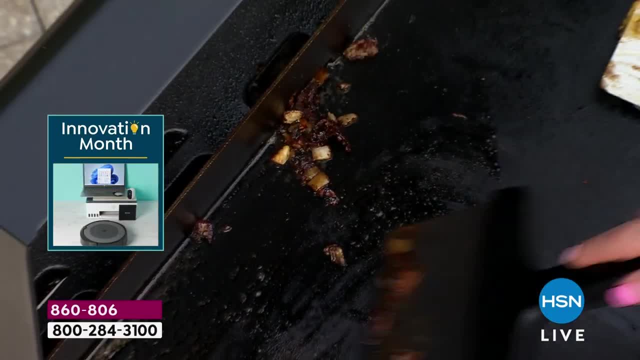 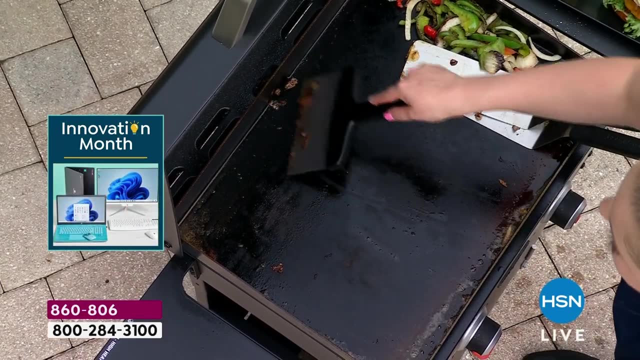 your stir fries, Pasta. Wait, you can do pasta. on here, You can do pasta. you know what I love to do: shrimp scampi and muscle scampi. yeah, because, remember, those things are not going to be falling through a grate like it would on a traditional grill, for sure. so this 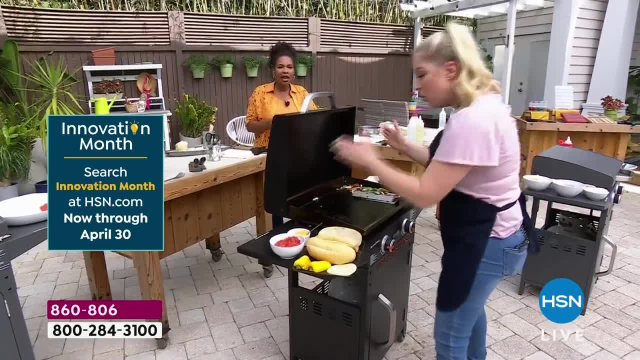 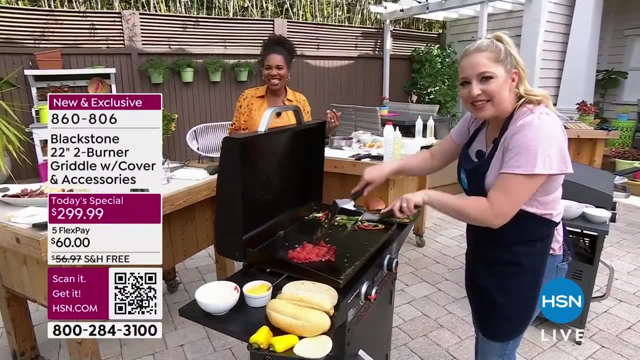 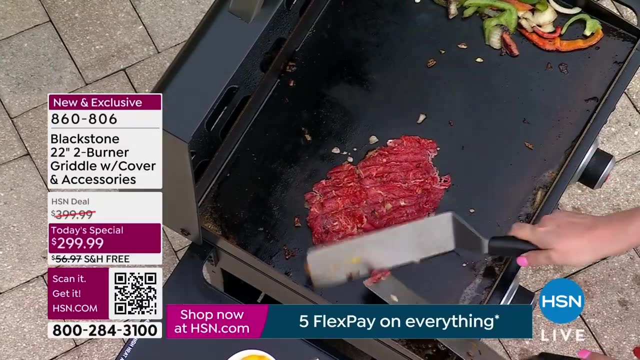 is completely a different element. you're not having to worry about that. okay, we got to get on to our philly cheesesteaks. okay, i see some folks who are standing by. are you wait, are you? this is the thing, this is the joy about it. all you're doing is choosing your color. we've got. 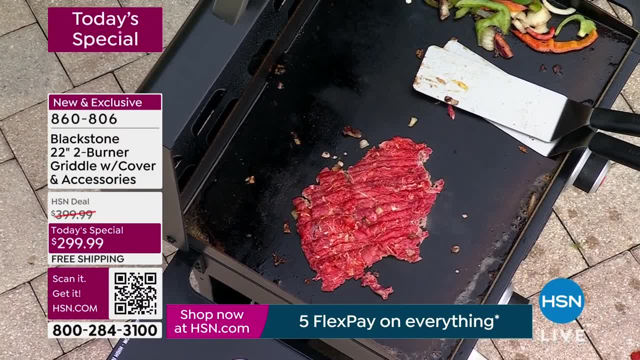 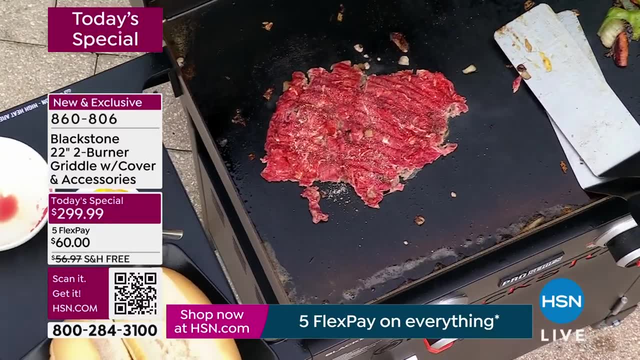 it in black. that's what taylor's showing you right now. we also have it in the gunmetal color and we have it in bronze, if you want the bronze color. we have fewer than 100 left and that's for the, not only for the rest of the day, it's for the rest of the year, because it's not going to be. 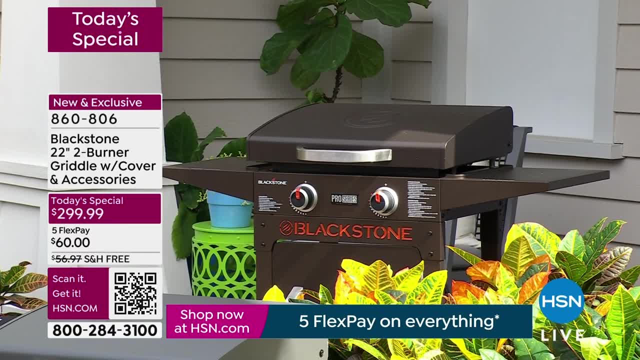 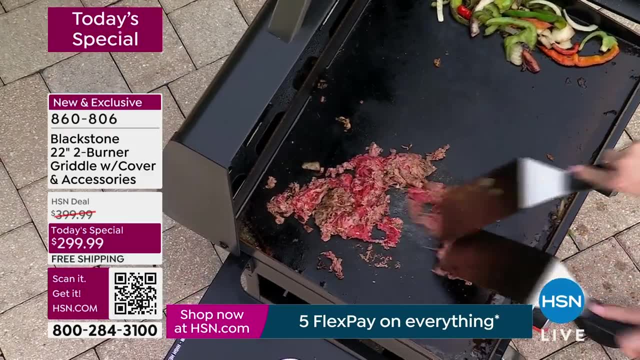 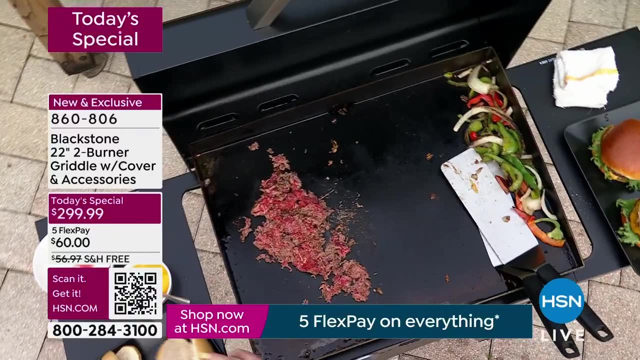 a today's special again. that's right for the rest of 2024. so if you want that bronze that you're seeing right there, please don't wait, um, and remember we took a hundred dollars off of our regular hsn price, um, and it's free shipping and we'll send it to you and you're going to get those. 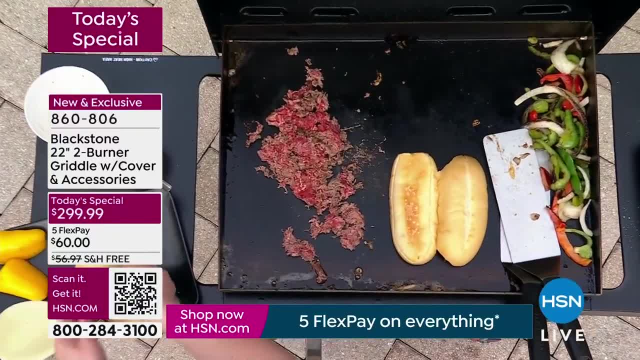 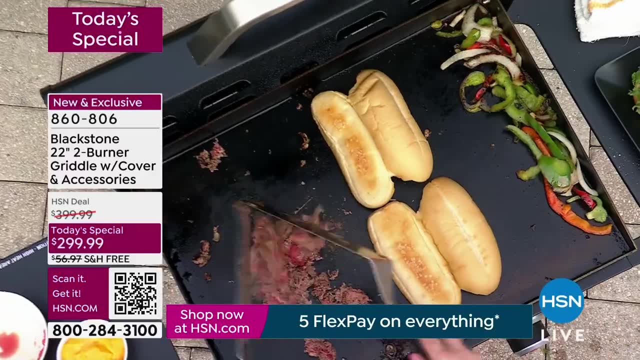 two spatulas that taylor is using you and the scraper that she's been using. those are all stainless steel. yep, you're going to get the cover for the griddle. you're going to get the um, as you can see on the side, where you can prep your. 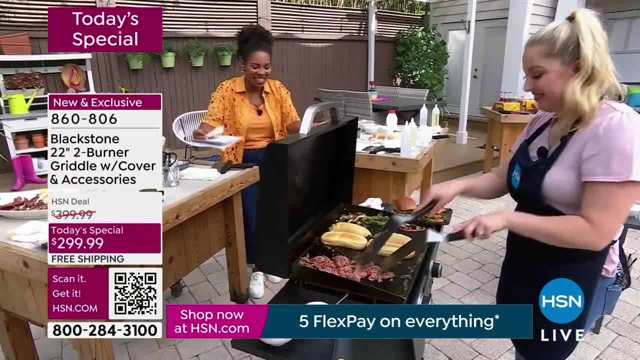 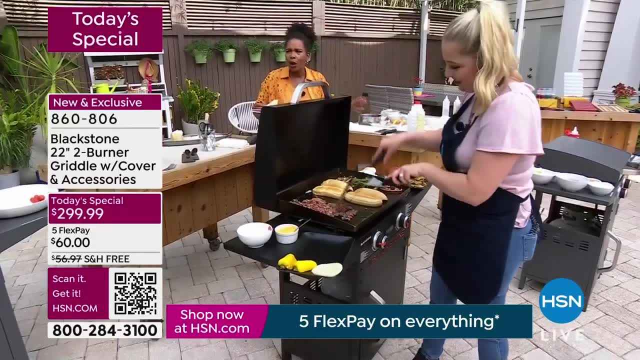 food and have your food. all done your best, your best friends on either side. i don't got to go inside for anything. all you do is add your propane tank and the food, but blackstone is doing all the rest of it. so go ahead and pick yours up. so what do you? this looks like. oh, this is the cheese that. 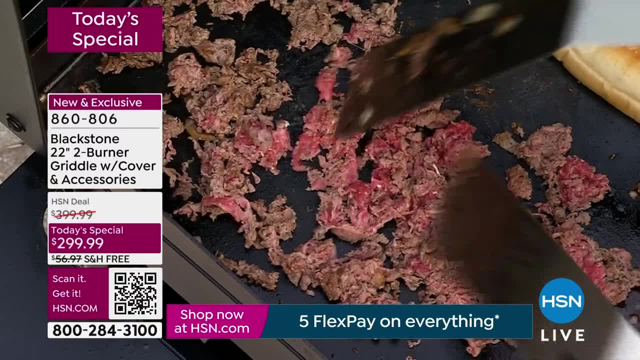 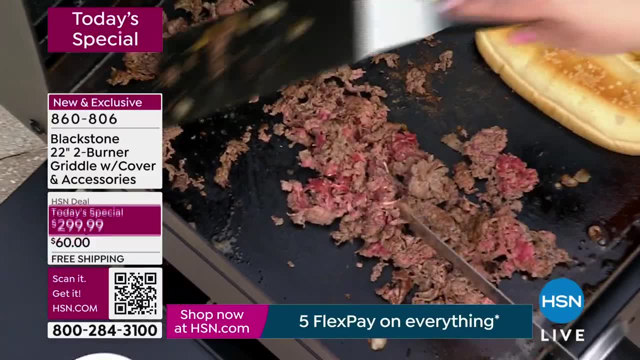 you're doing yep, philly cheesesteak, i just bought some shaved ribeye. if you want to do a little cheat feeding more people and you want to kind of save on your dime, just get shaved roast beef and it tastes amazing. so that's the great thing about this blackstone is you can have fun with your ingredients. 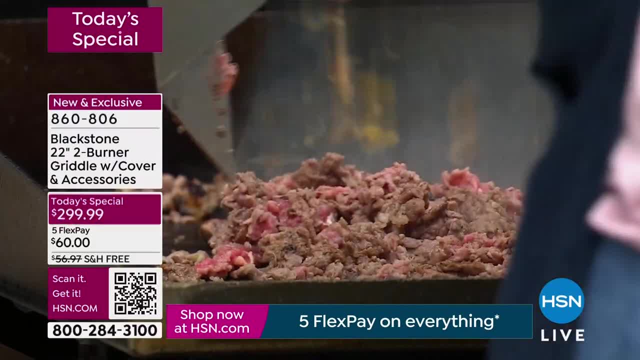 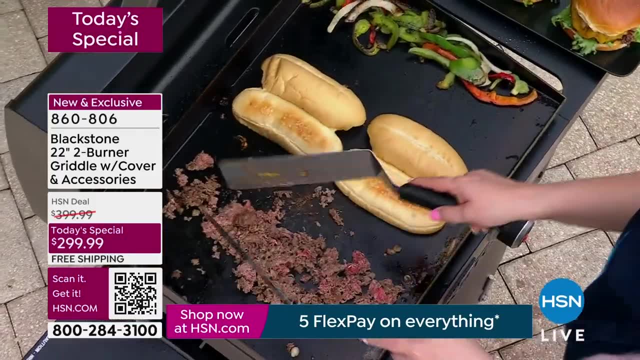 you're using. however, you need to stretch it because it can feed a ton of people. this is 22 inches across, that's right, so it's a really great size. this is not um the size you're going to want. if you have a family of 10 and then you're cooking for 20 plus people, i wouldn't recommend that, okay. 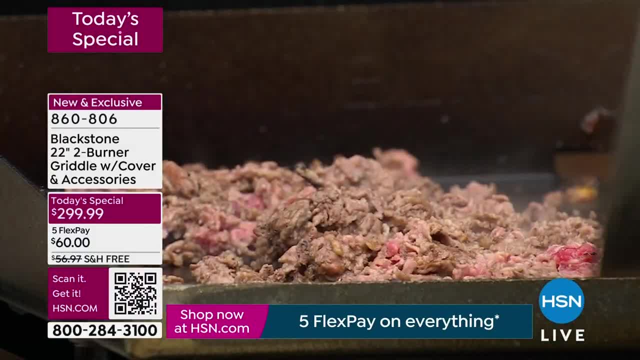 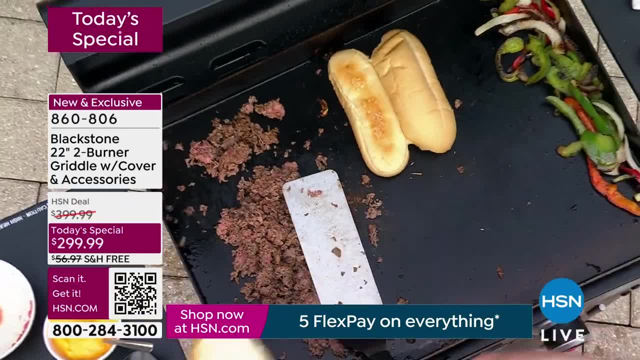 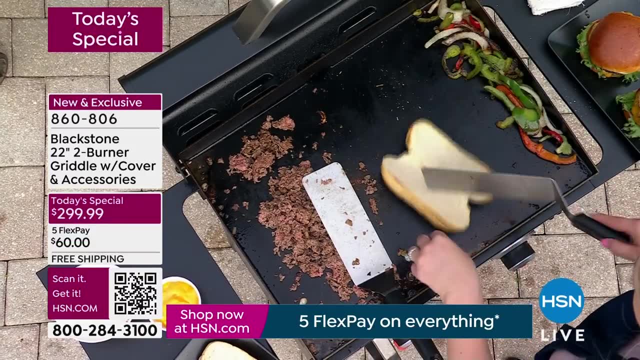 how i'm using it for multiple purposes. i just wanted to toast my buns a little bit. wait a minute. so you didn't have to have a toaster oven to toast the buns- no, ma'am, you didn't have to have a separate grill to do the um, the vegetables. nope, you have it all together. this is it one. 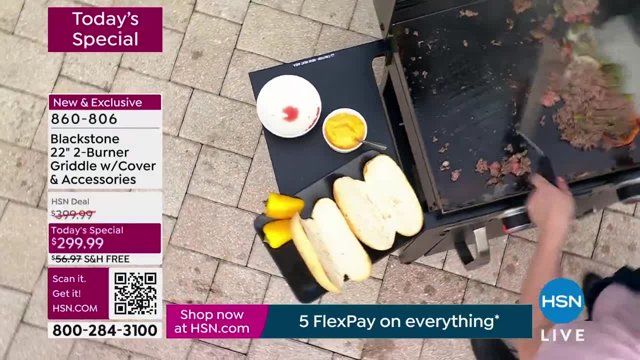 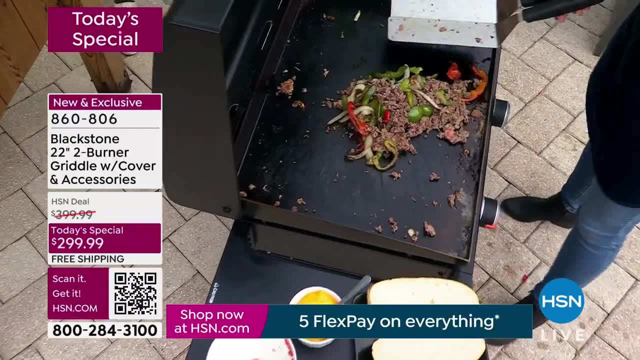 that's it. and then there's your side table, so that you can prep and serve all at the same time. that's why i said it's my bestie, because i don't have to go inside for anything. look, i've got my cheese sauce here. i have my 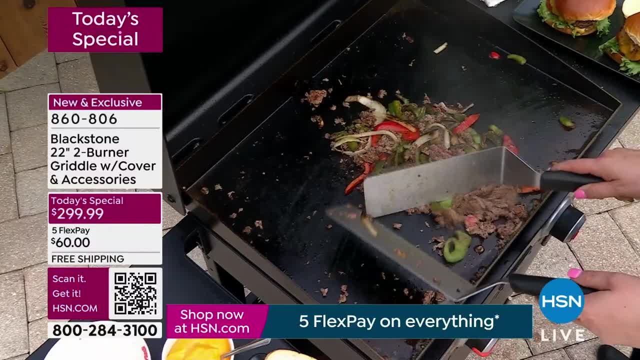 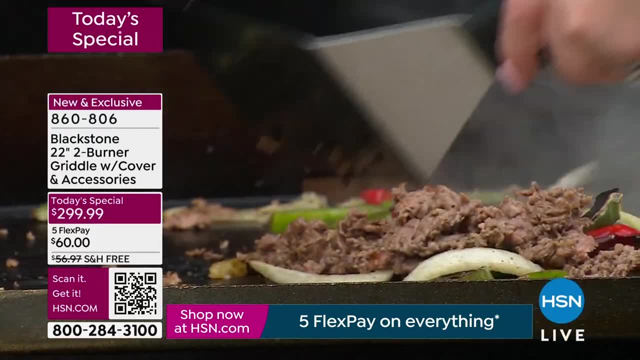 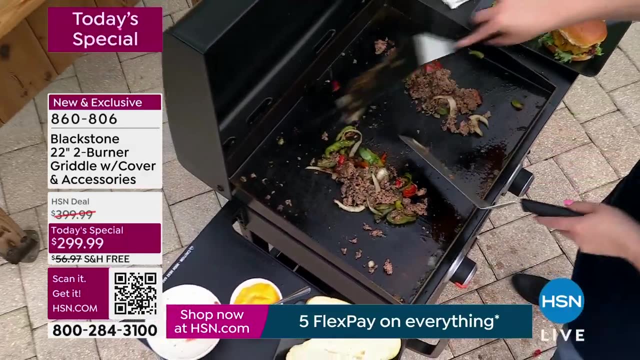 i've had my cheese and my plate prepared, ready to go. um, it's, it's a beauty. i, i love having those arms on the side, so really, really helpful for me. oh, my god, watch me deviate this too. so for me, i love, uh, do you like whiz with or whiz without? have you heard that i have? i, um, i'm, i am not a. 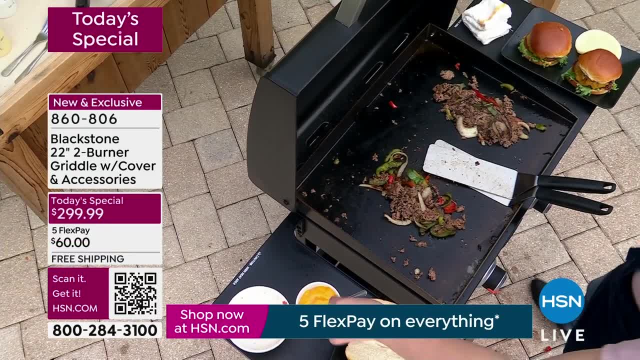 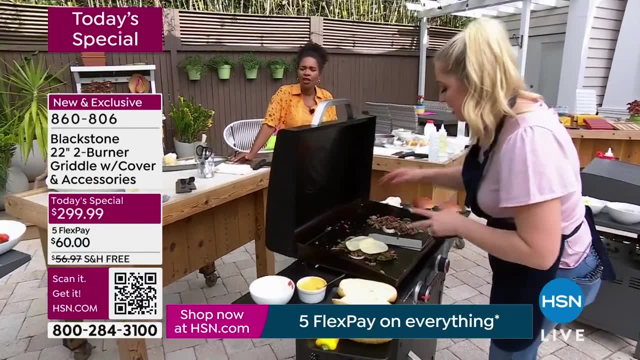 pro in it. okay, i think it's. with that you have the cheese, right cheese. it's whipped cheese like cheese sauce, or you can do provolone cheese, or you don't have to have any dairy on it at all. can you do both you? that's what i do. you're on my level, girl. i know you're on my. 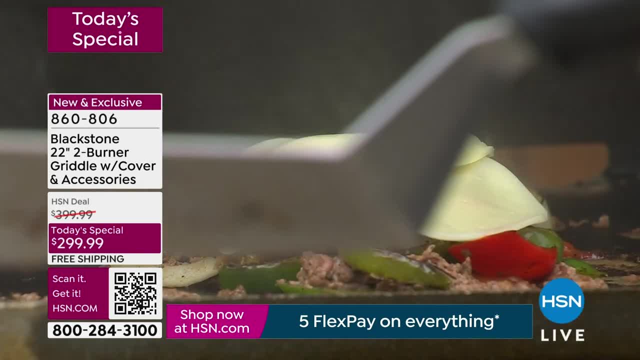 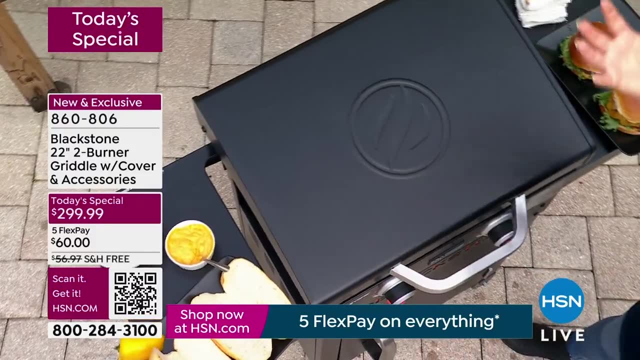 level. that's like too many decisions. i'll just take it all. give me the works. watch this. i put provolone on it. i'm gonna close the lid. remember your. your hood here is acting as your dome. okay, so you're able to melt those cheeses. i could have 15 burgers. i'm cooking on here and melting the. 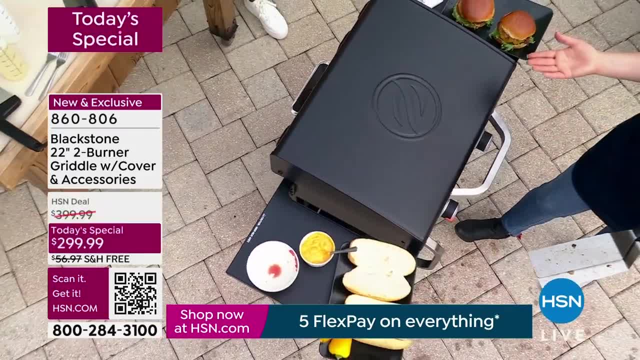 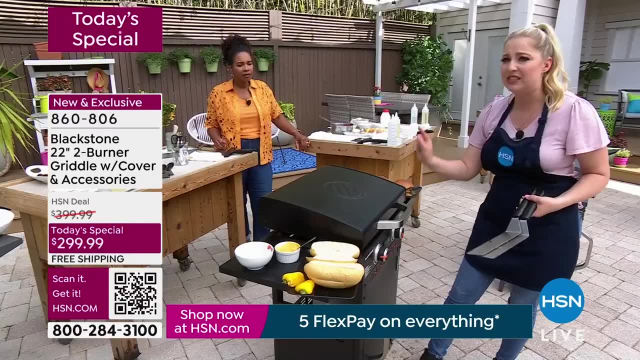 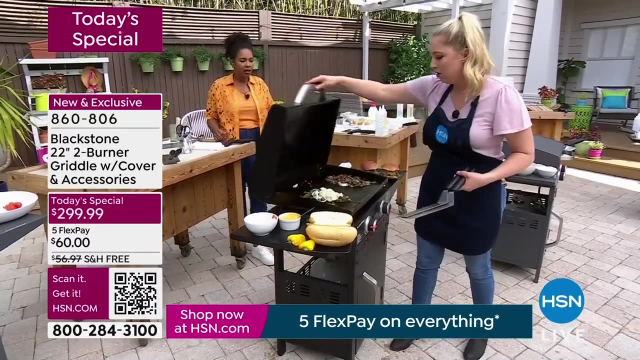 cheese all at once within a couple of seconds. um, you can. you can absolutely cook your veggies, steam them with a matter of minutes by keeping this hood down. this is a wonderful feature. on this specific blackstone i want to mention: not all blackstones have a hood. this is game changer. yes, and look at that changer. this is, you see, do. 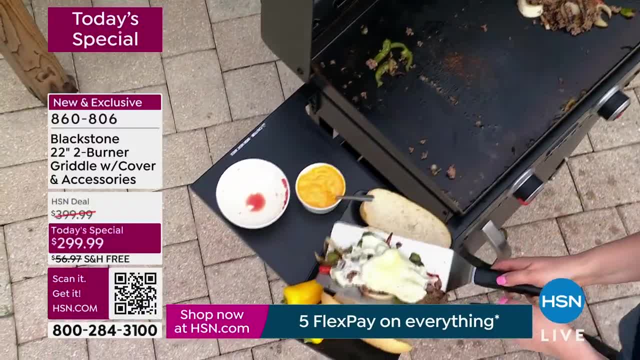 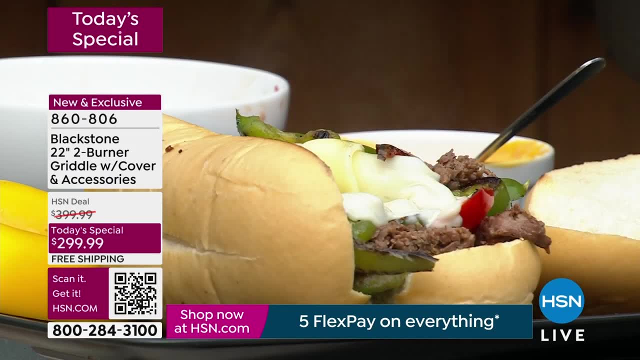 you see how fast the cheese melted. yes, and you're not, you know, going out to a restaurant and paying extra to have the kind of cheese, the amount of cheese, you want, right? you just do it because you're at home, that's right. you do this on it. can you imagine, just on a random tuesday night when you want some philly? 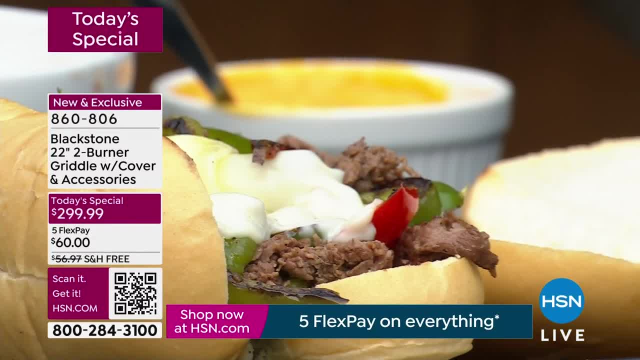 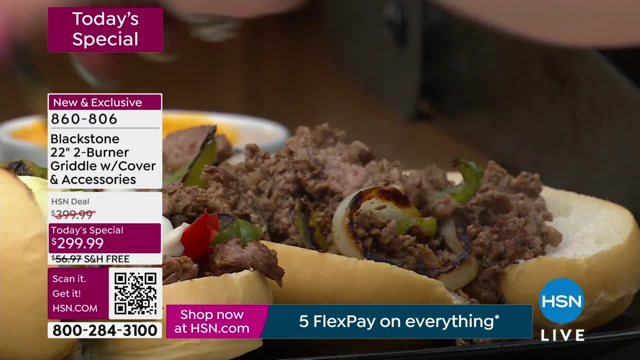 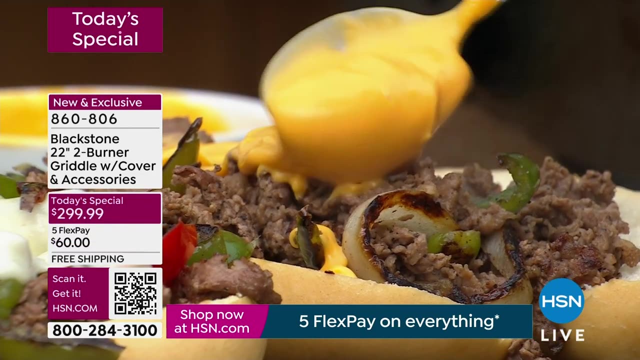 cheesesteak your way. uh, actually last tuesday night- it was a random tuesday night- we had philly cheesesteaks. i'm not even kidding, we sure did. and it was delicious and it was quick and it was simple and it didn't hurt my uh budget, my grocery budget. there's a philly cheesesteak store or a restaurant. 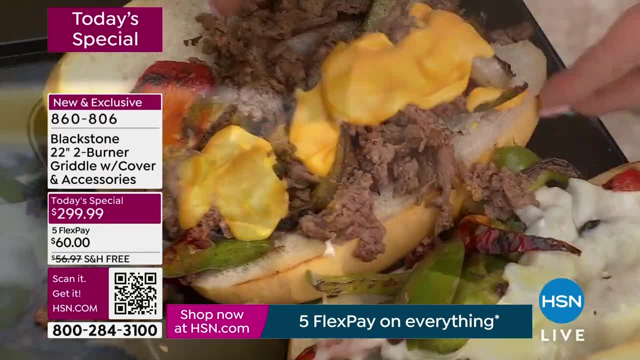 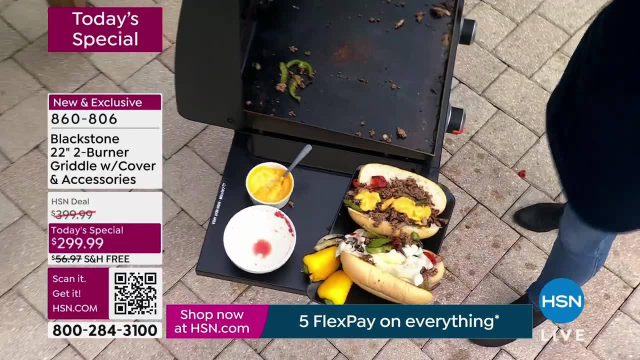 rather right down the street, probably like two miles from my house. yeah, um, fifteen dollars for just the sandwich, no fries or anything included, serious? so i said absolutely not. i'm not doing that every time i want a philly cheesesteak. i'm gonna learn how to do. 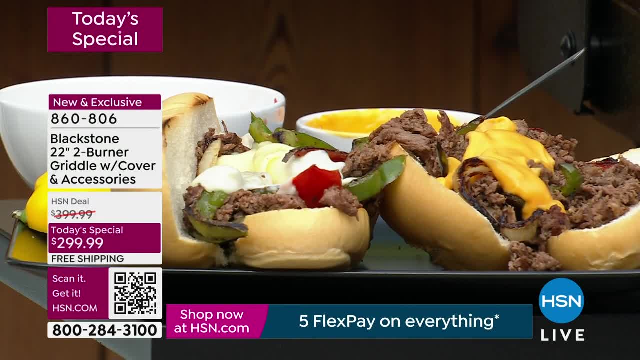 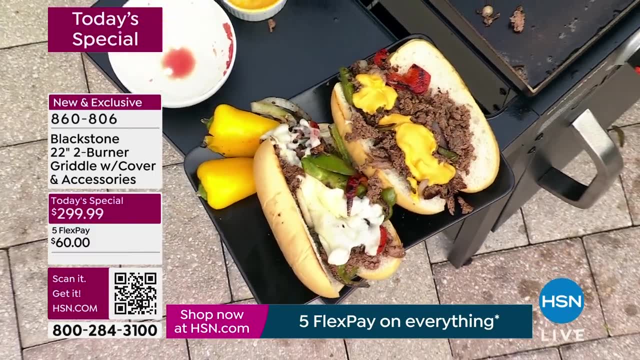 it. yeah, and look at this, i have learned how to do it. whether you are watching your diet, maybe you don't want the hoagie, maybe you want to make a wrap out of it. maybe you want a philly cheesesteak salad. if you've never had a philly cheesesteak salad, no buckle up. oh my, because i'm telling you. 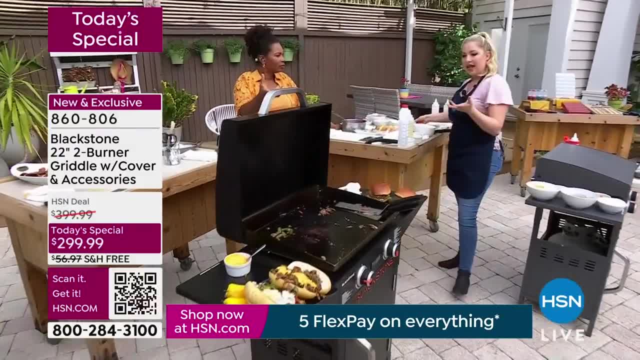 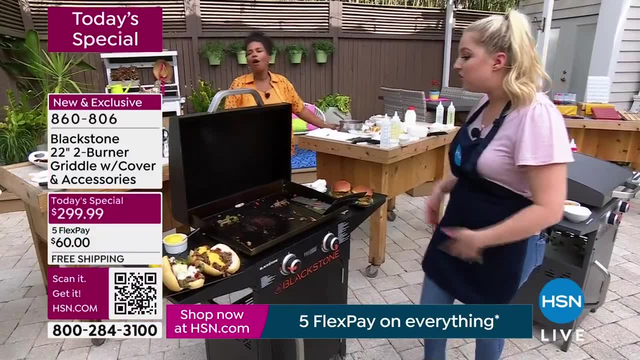 it is absolutely divine. so all of that on a bed of lettuce. on a bed of lettuce you can add whatever other veggies you want underneath. i love thousand island with it. yeah, you can do oil and vinegar if you wanted to, but just you know, make it to your own creation what works for. 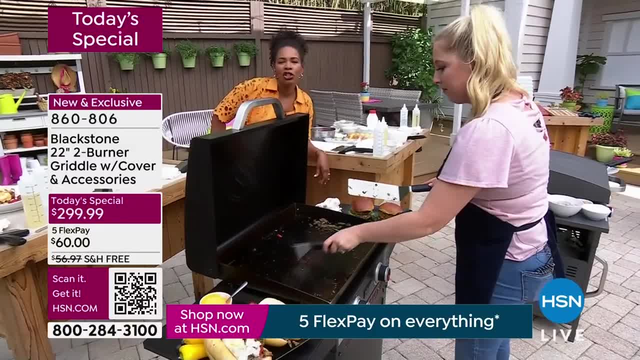 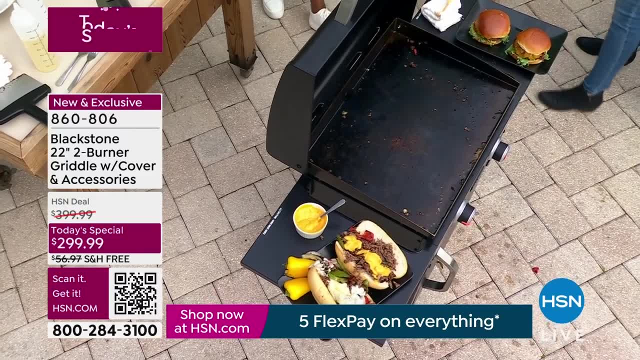 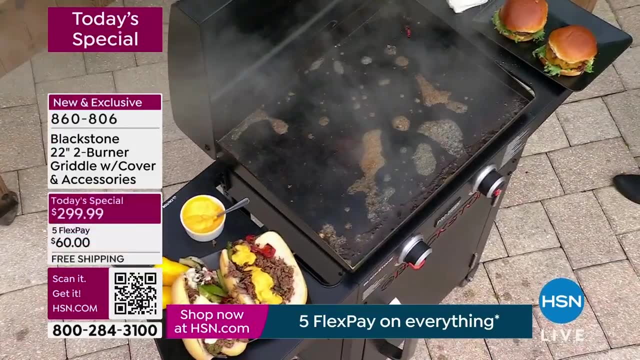 you in your family and guess what? no washing pots and pans. you scrape it and you rinse it with water and you walk away and you're ready to go again for dinner or for dessert or the next day. yep, this is the deal. you're seeing it there in black. we've got it for you in the gun metal, which is that. 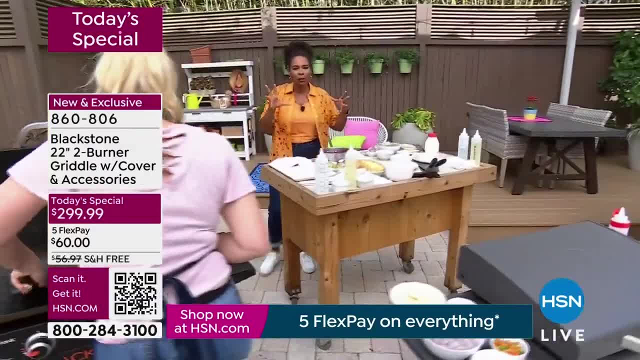 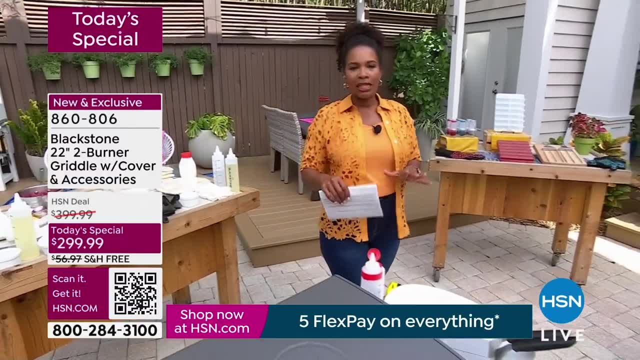 really cool kind of charcoal gray color and we have it in bronze. but in bronze we've got five left and then we say goodbye to the bronze. this blackstone griddle is only going to be a today special today and not for the rest of the year, not for the rest of 2024. so we want to make sure. 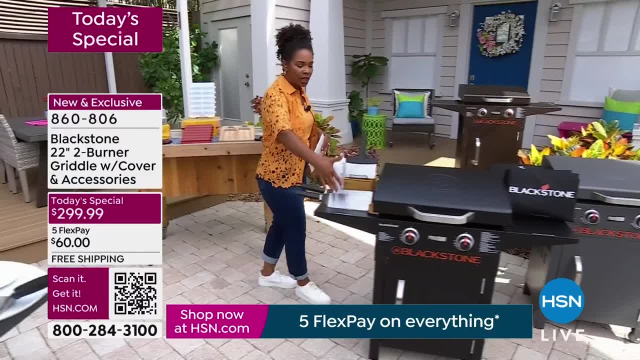 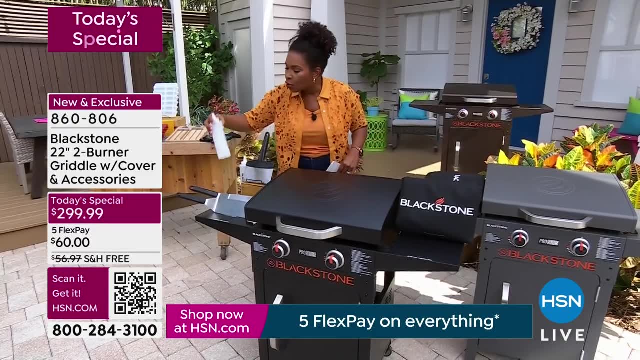 that you get yours. you're getting everything that you see right here, including the two stainless steel spatulas, the stainless steel scraper that's to clean it. so no washing dishes. you're going to get two of the squeeze bottles. you're gonna have just plain water in one. so when you're done, 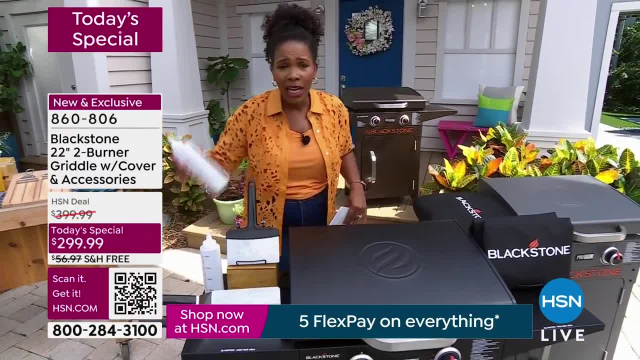 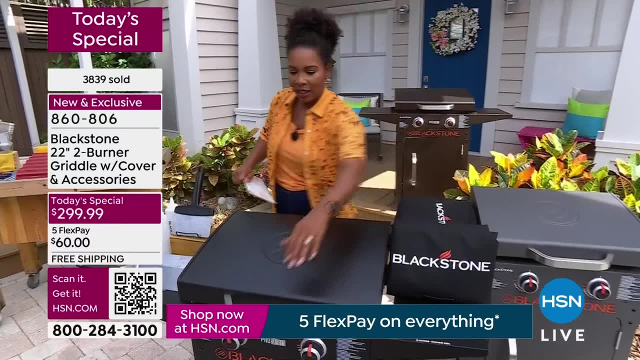 cooking. you wet down the grill, you scrape it, you can have your oil and vinegar and you're going to get the other. it's completely up to you. you're going to get the cover so that when you're not using it it stays nice and covered. you've got this nice 22 inches of space that you can cook. 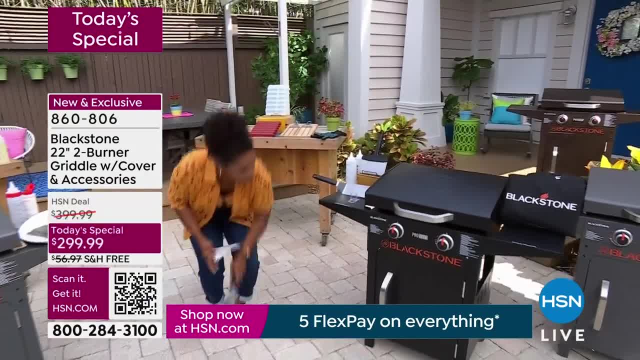 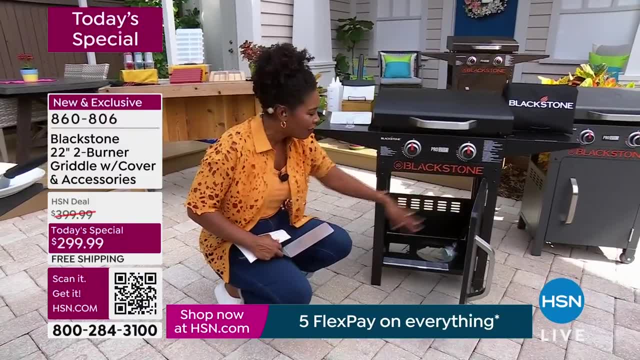 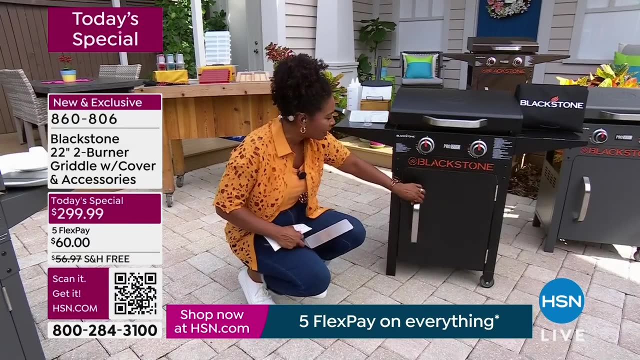 on. I'm gonna come around the front, oops, because you also are gonna get the ability to house your propane tank on the inside of this door. and then, when you're not, when you're you know, when you've got it in there, you just close it up and this door is. there's a magnet, magnet, so it's not gonna. 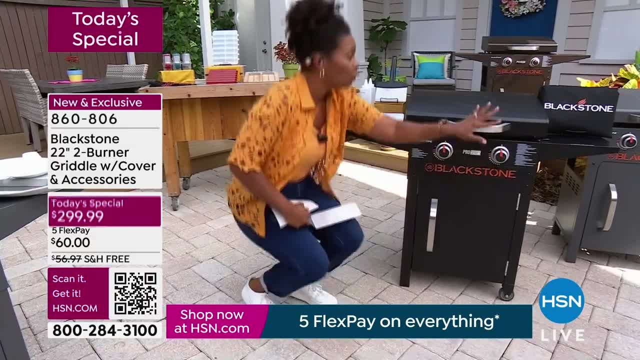 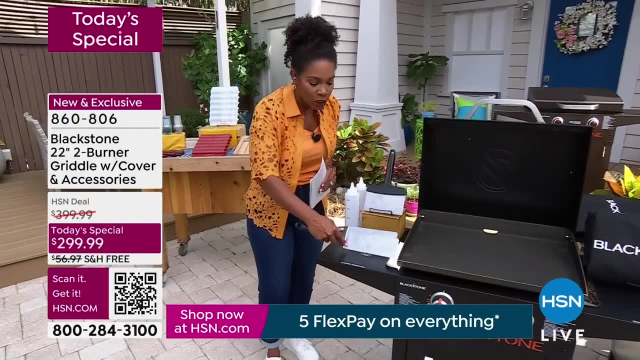 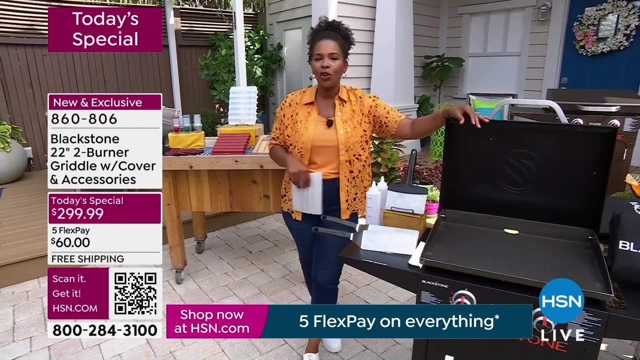 fly open. you even have two separate controls for two different sides of your griddle. this is your today's special. we took $100 off. it's free shipping and the food is divine when you get it home and cook for yourself and for your family. go ahead and pick yours up. you can shop on hsncom. 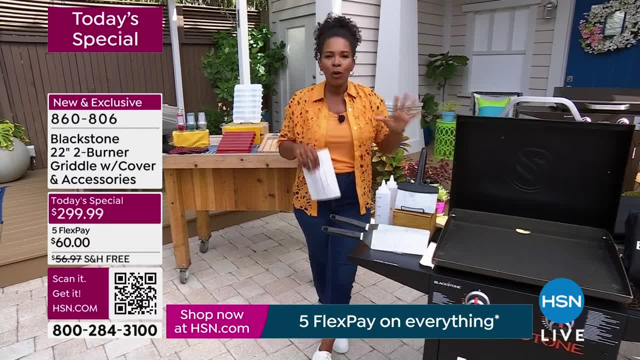 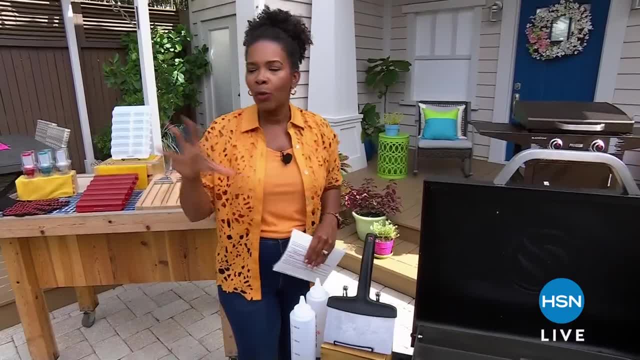 or the HSN app, or use that QR code. we're gonna take a quick break and give you a chance to place your order, and if you want the bronze, now is the time to get it. we've got more food. what? during the day, we're gonna be eating those Philly cheesesteaks, believe that- and we'll see you in just a little. 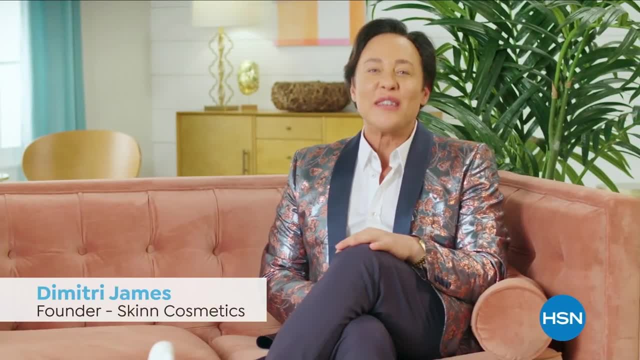 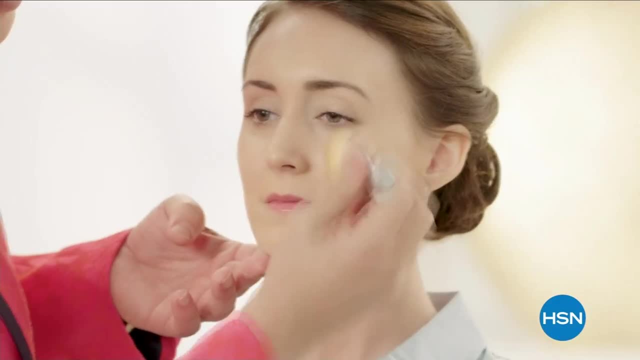 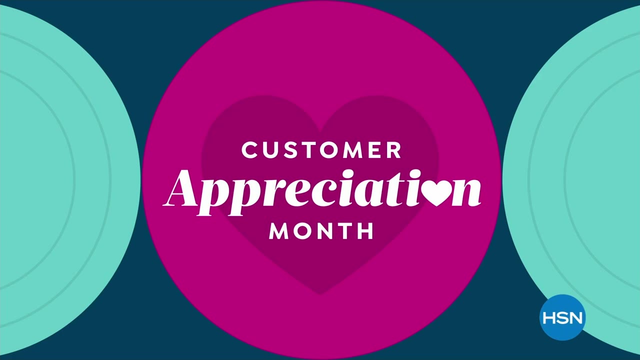 bit. we understand every woman's skin is unique. we offer real beauty solutions, empowering women to achieve healthy, radiant looking skin. genuine beauty begins with skin. it's customer appreciation month and it's all about you. for the entire month of April, we're showing the love to our 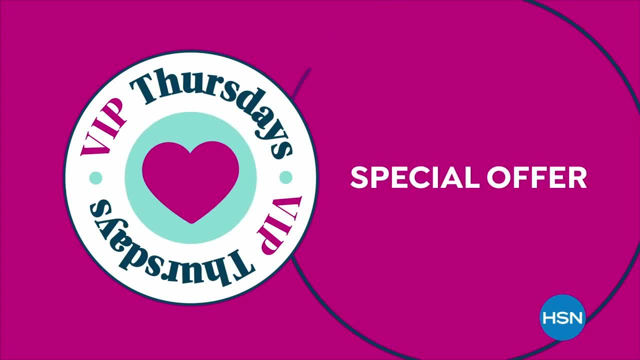 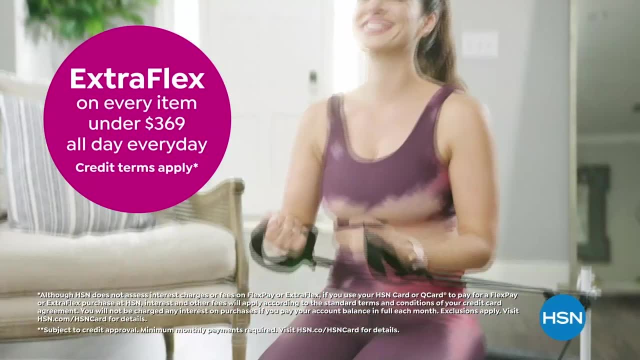 HSN card VIPs with exclusive perks, like VIP Thursdays, get a special offer every Thursday in April, plus extra flex on every item under $369 all day, every day, or VIP financing on so many items, not a card member. apply now and instantly get $40 off when. 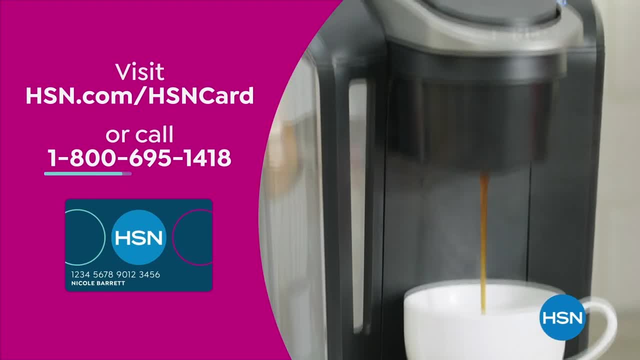 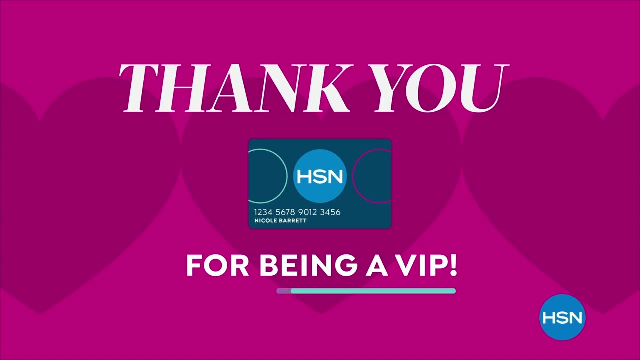 you're approved, visit hsncom, slash HSN card or call 1-800-695-1418 for details on our exclusive VIP offers. thank you for being an HSN card. VIP attention: all crafters. get ready for an exclusive 24-hour event just for you. 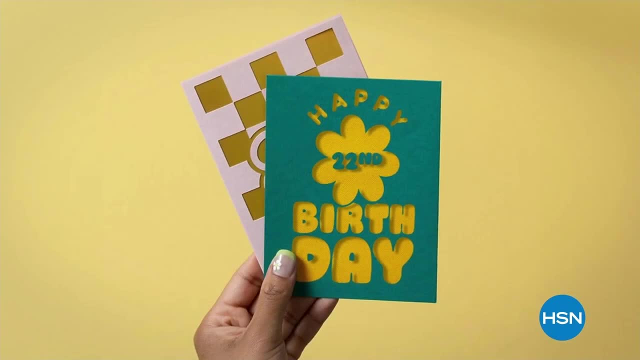 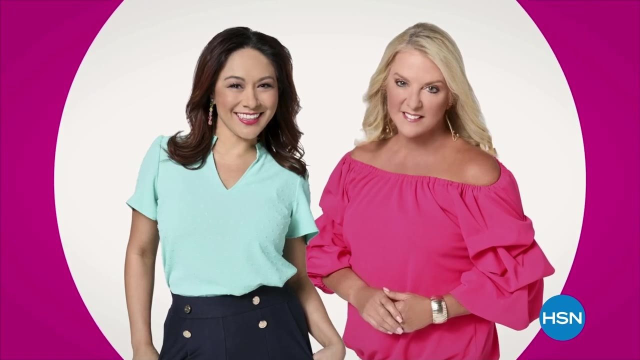 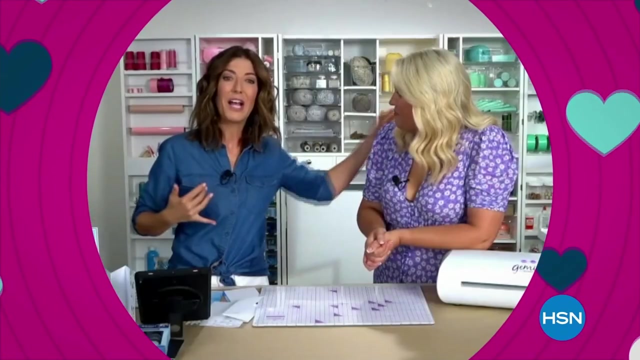 it's HSN's crafters appreciation sale- from scrapbooking to paper crafting and even home decor- and it's all on sale. plus, join HSN's craftinistas Tina and Suzanne for the premiere of up close and crafting. live our first ever hands-on crafting event with your favorite crafting experts. 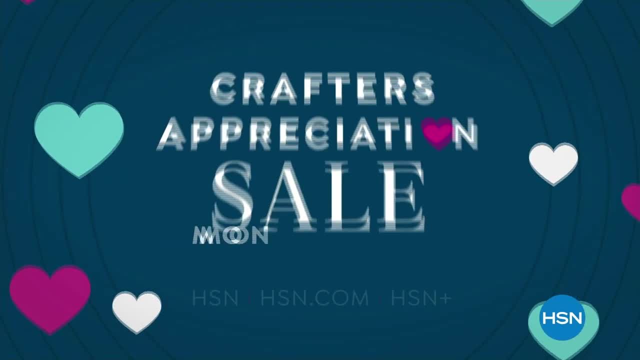 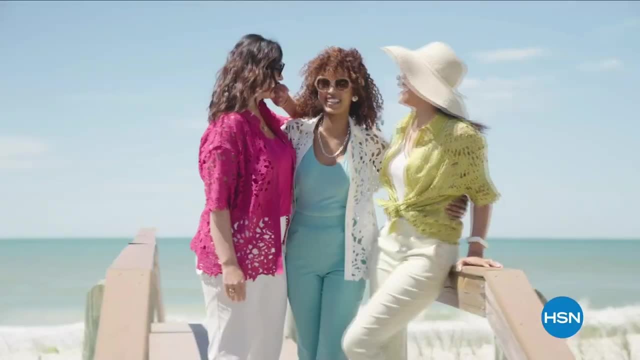 and lovers like you. it's a 24-hour crafting extravaganza only on HSN. get ready for sunshine and style. join HSN for an exclusive 24-hour event dedicated to you, to making your transition from spring to summer effortlessly fabulous. preview next season's. 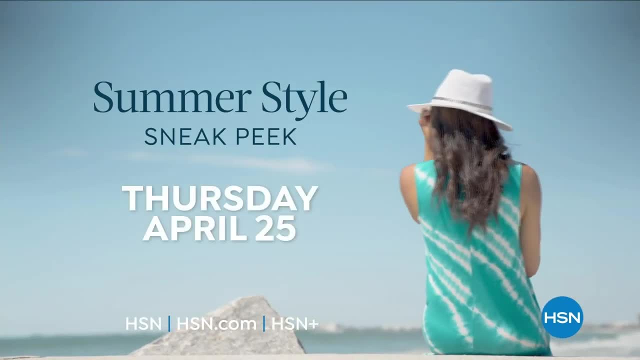 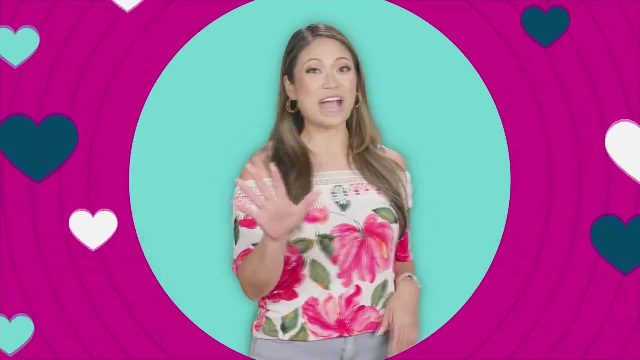 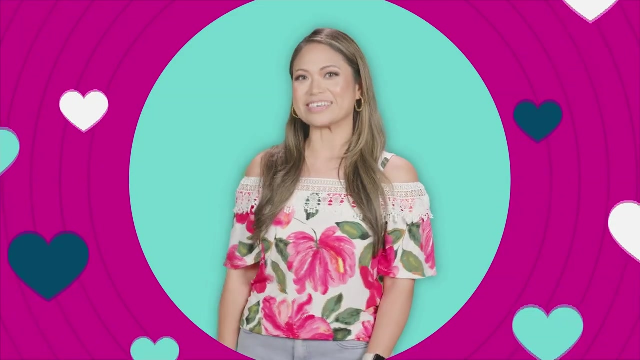 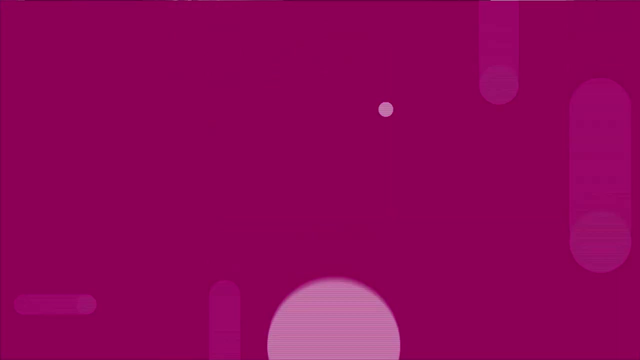 freshest looks during our summer style sneak peek. Thursday, April 25th, Saturday and Sunday: take it all home all weekend long. for less, it's five flex weekend- and for even more super amazing savings. come back for mystery Monday to reveal your mystery deal. it's time to get started, as Mediterranea is here. it's time for the safety, and he won't. 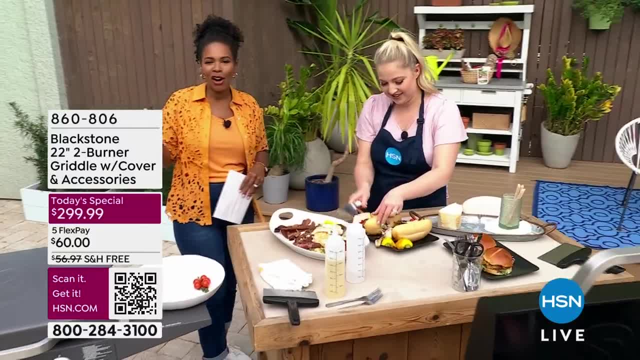 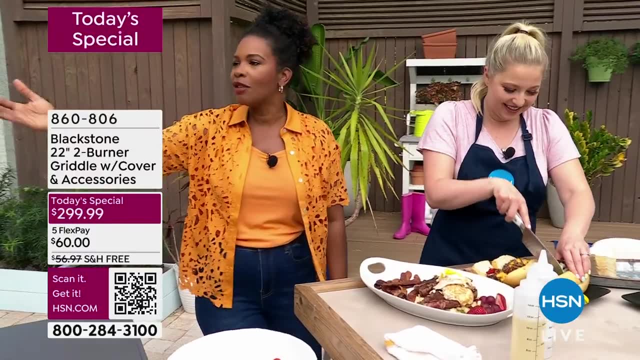 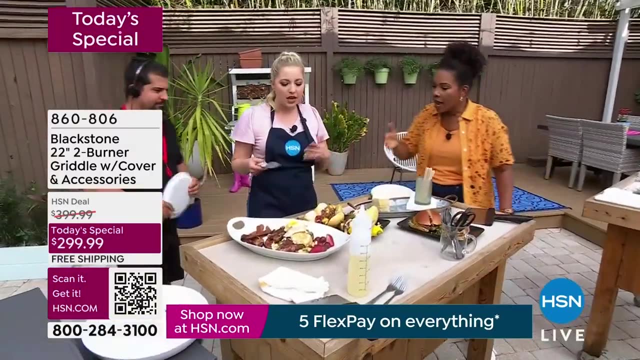 like this chance. so I'm gonna join JAMI and I'm your, certainly I want you. I'm gonna invite the crew to come on and the got their play to the food are really get a non. they've got your play to the food ook. so amazing, radar old fainted, you've able to keep those simple. I know this is really it could. 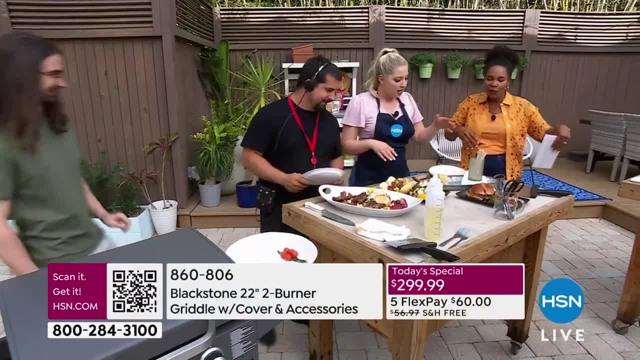 You could feed a drone of people. Come on, Don't be shy. There's a lot of food out here. There's little plates and forks here- Forks. I went ahead and this is the cool thing is, I love to be able to cut things. 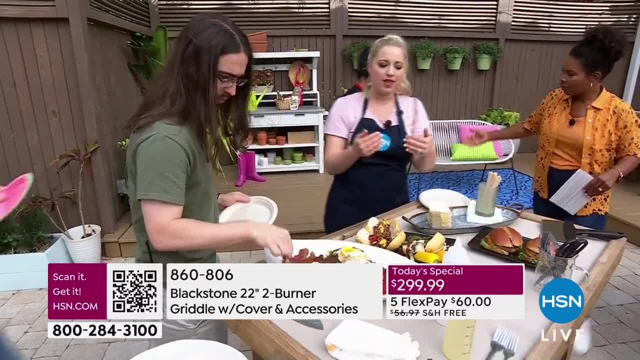 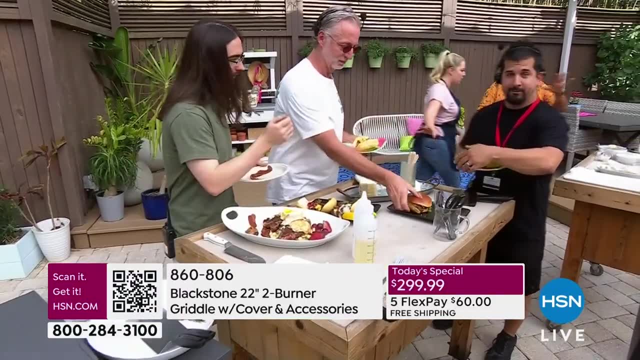 like: cut your burgers, cut your Philly cheesesteaks, so when your company's over they can have a little bit of both. And you've made both things for them to taste For sure. How fun is that? Something for everybody. 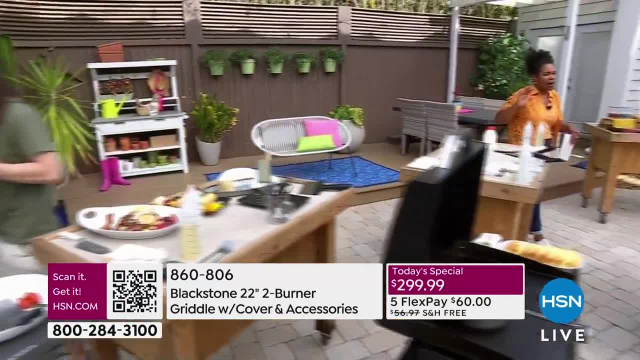 Come on around, I'm going to show you If you're just tuning in and you're saying, wait a minute, it looks like a party. It does. I love it. This could be every day at your house. Look at that food. 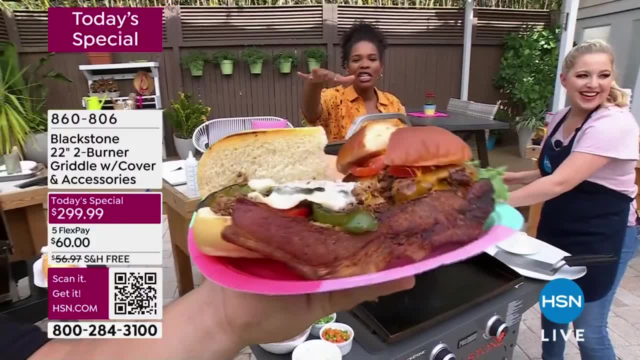 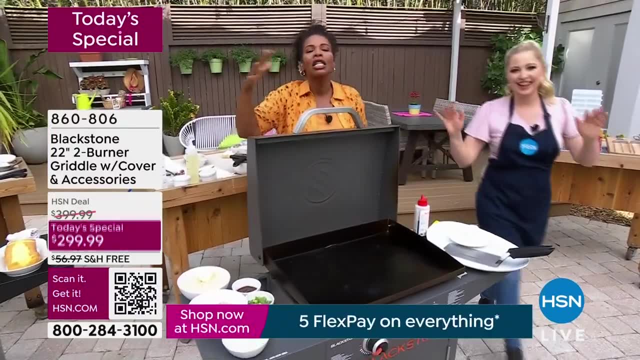 Look at that plate. Oh my gosh, Oh my goodness. All you need now is a cold drink and it's a party. That's it, girl. That's it. Sign me up For sure. Taylor Mock is here cooking for us on the Blackstone griddle. 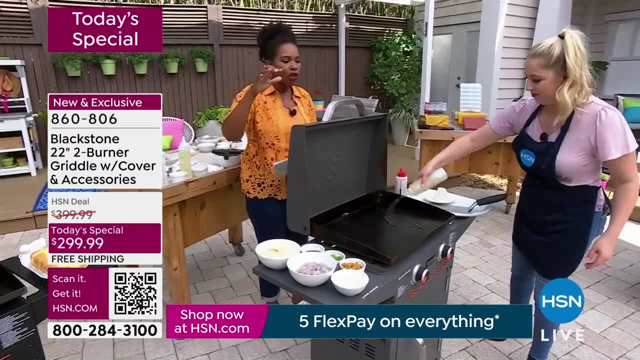 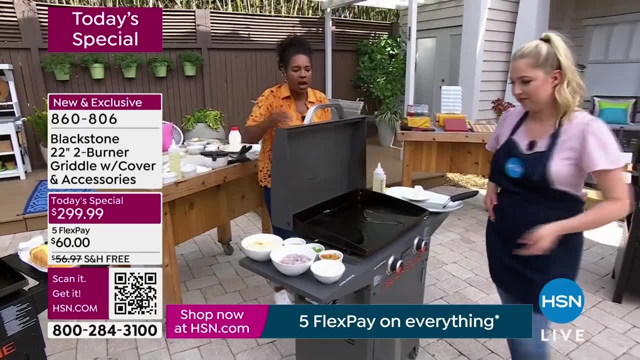 22 inches of cooking space. You're going to get that griddle that when you're cooking, whether things you know. it could be a nice big juicy porterhouse or it could be something as small as shrimp or chopped onions or rice. 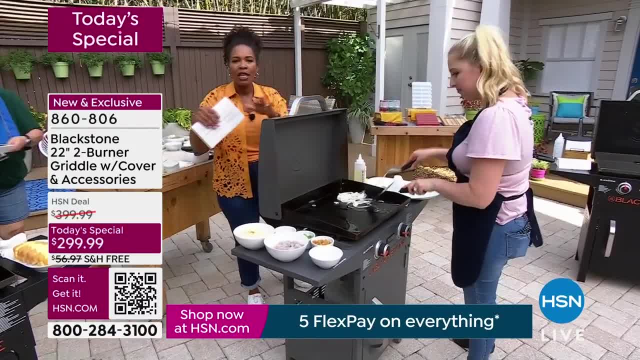 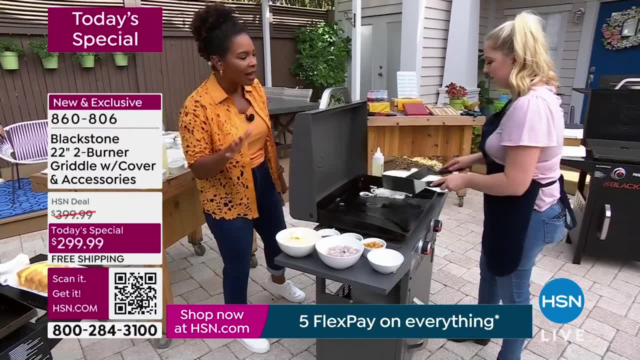 even Absolutely Nothing's going to fall through, because it's not like the open grill. This is your griddle. It's restaurant-style cooking and restaurant-quality eating. Every time you cook with this, you're going to get the two stainless steel. 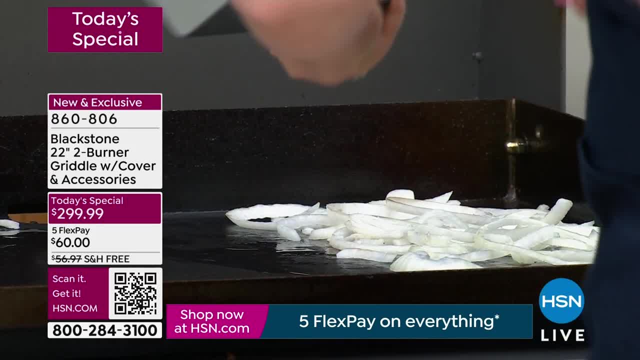 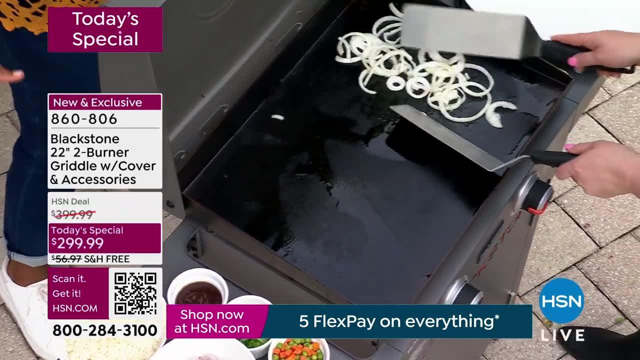 spatulas that Taylor's using. You're going to get the stainless steel scraper for when you're done. I love that. You're going to get the side tables as well, so that this is where you prep. This is where you serve. You're going to get the cover for the grill when you're not using it. 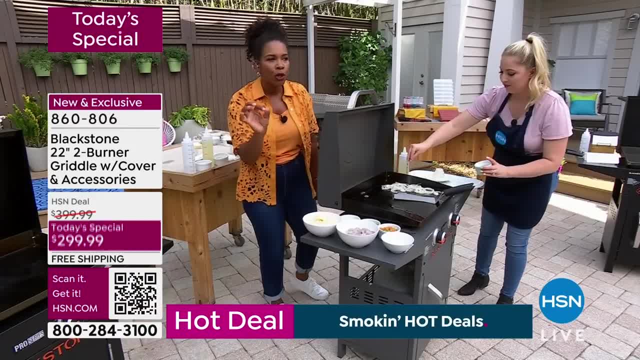 And on the front of each grill there's a little door. That's where you put your propane tank. So it's not on the ground, It's raised up, It's covered up, Yes, And you can hide these in there too. 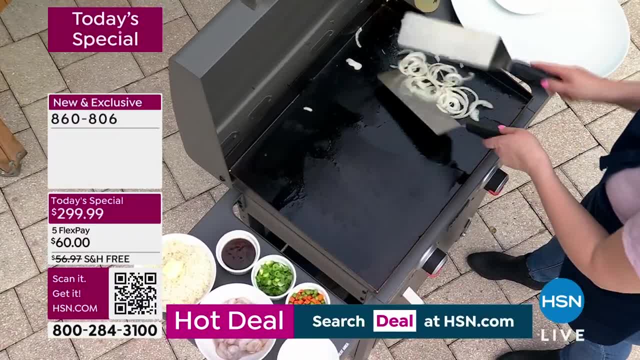 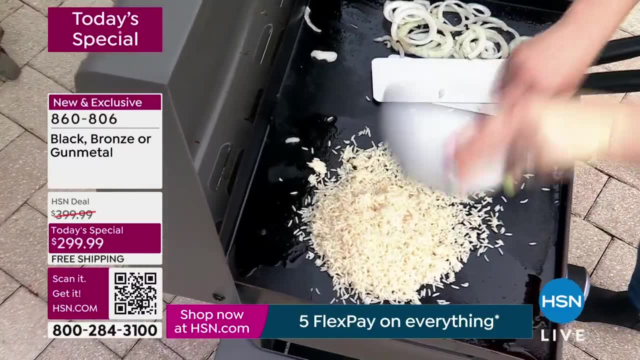 Oh good, So everything's there? Yes, And then you're also going to notice there are two separate heating elements and heating controls. So if something needs to be really hot, something not so much, you've got the ability to do that. 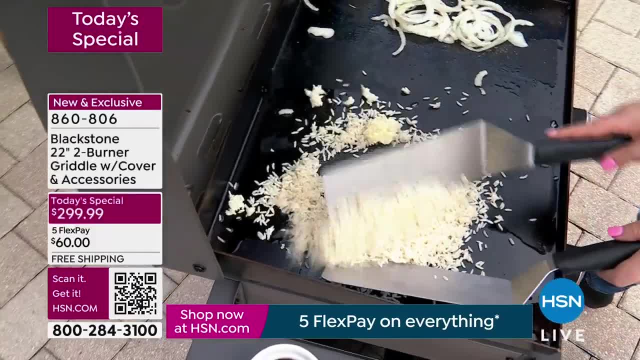 You're seeing it here in the gunmetal color. We have it in black And we have a handful left in the bronze color. Oh, we already know that's going to sell out. And then we say goodbye to that. Yes, You know what, Taylor. 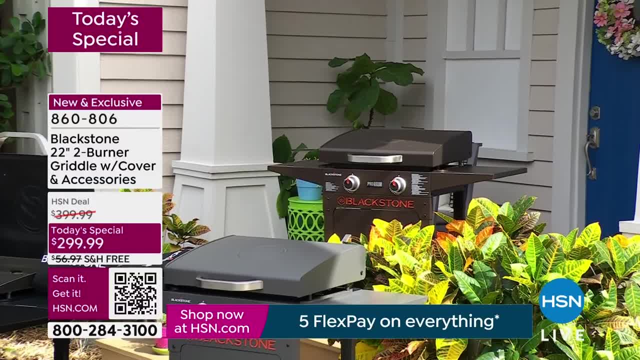 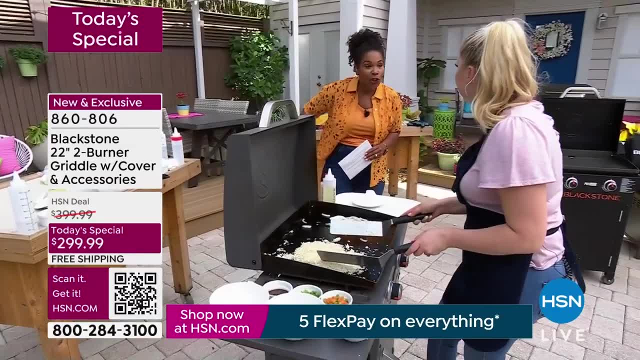 This reminds me of my little six-year-old girl. Yeah, She's getting big, She's sweet. Her new favorite restaurant is a hibachi grill restaurant that we took her to. We took her to And she loves it. She wants to go all the time. 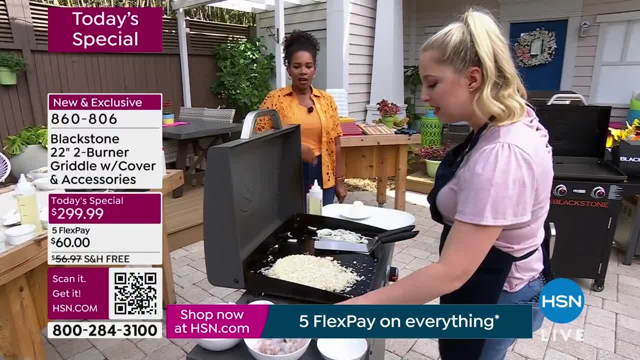 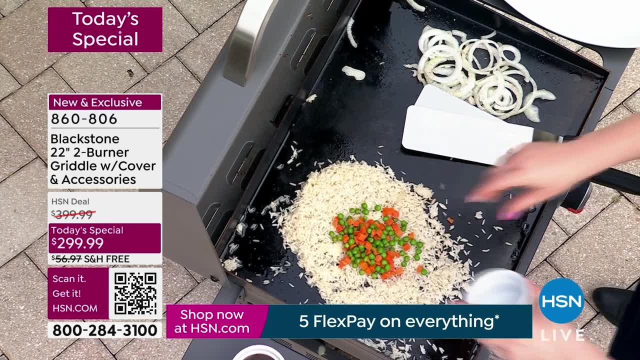 But it's triple digits every time the three of us go. I know It's expensive And you know when you start to add those numbers up every time you're craving it or you decide you know it's maybe not best this week that we go. 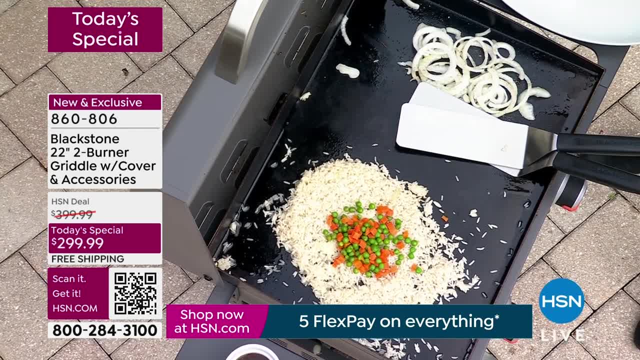 Maybe we'll save it for our birthday, et cetera. Then you start thinking, man, I need to save it for my birthday. I need to save it for my birthday. I need to learn how to do this, because it's not hard. 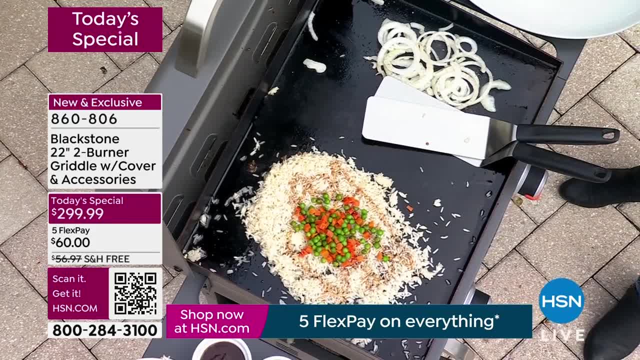 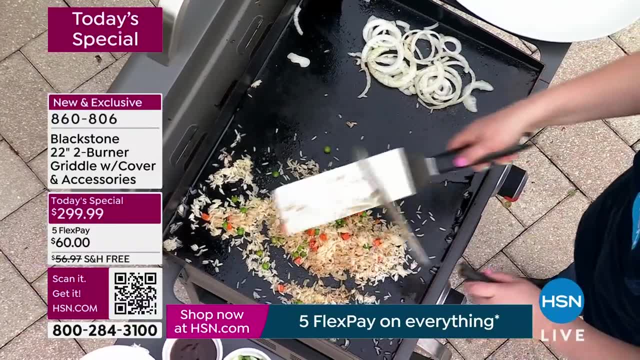 Putting this on your blackstone. I am telling you: you want to impress your family and friends. This is where it's at. You want this hibachi and you want it down pat. Yes, Here's what I do. I cook day-old rice. 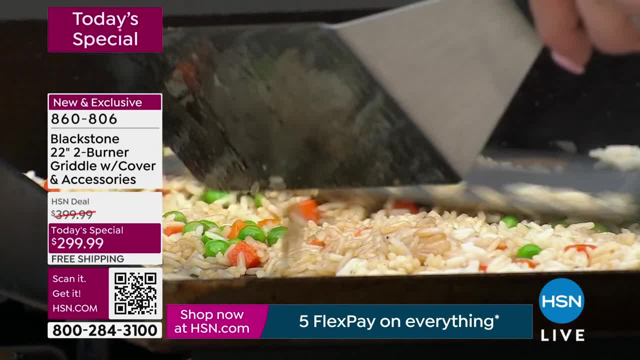 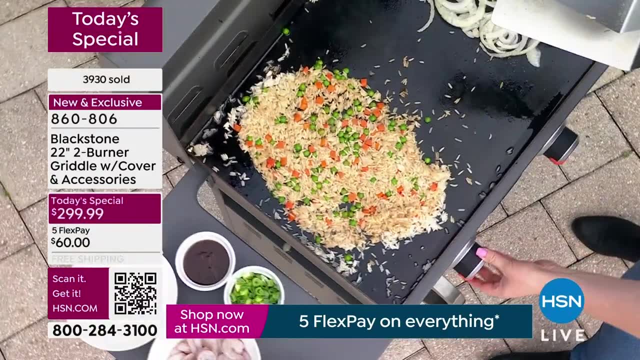 Okay, If you have leftover rice, you can even use microwavable rice and then put it on here when it's done, because you're basically steaming it, You're frying it. That's what you're doing. Yeah, By the way, I have this on high. 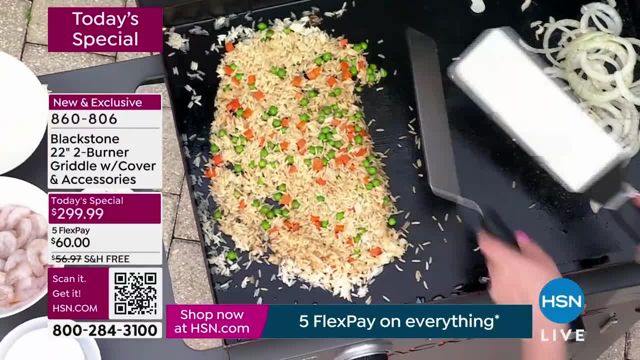 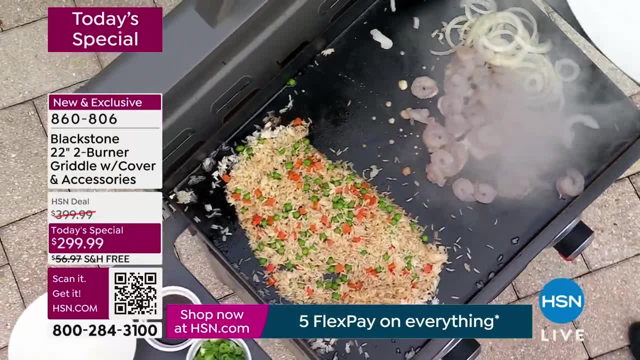 Okay, I have this on medium-low, I'm sauteing it. I'm sauteing some onions in the middle here. Get this, because we've got two units. Yeah, I'm going to work on my shrimp. Okay, So any protein you want. right, you can do chicken, you can do steak. 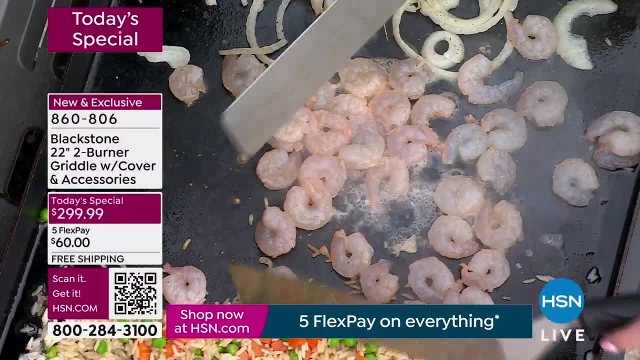 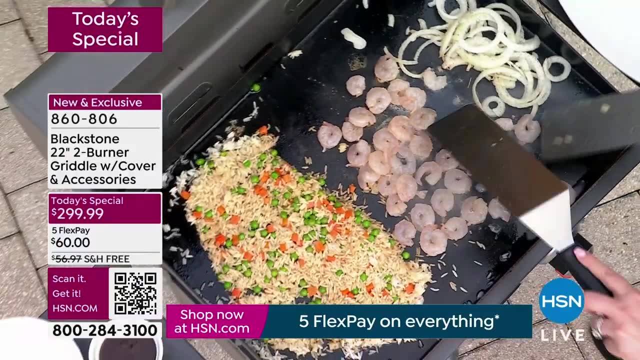 you can do both. Look at that sizzle. Yeah, you've got to love this And you're in control of what's going in your food. I want to mention: yes, we love those hibachi places. Listen, I go every year for my birthday, most of the time because I crave it. 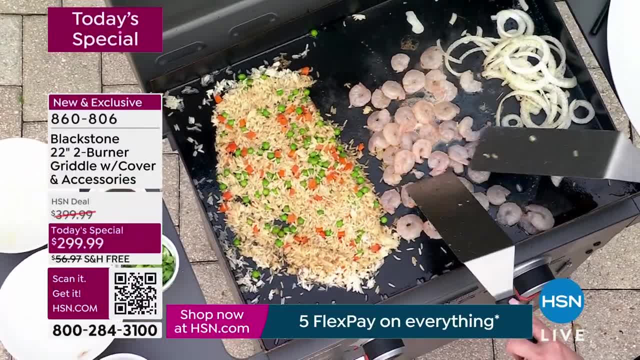 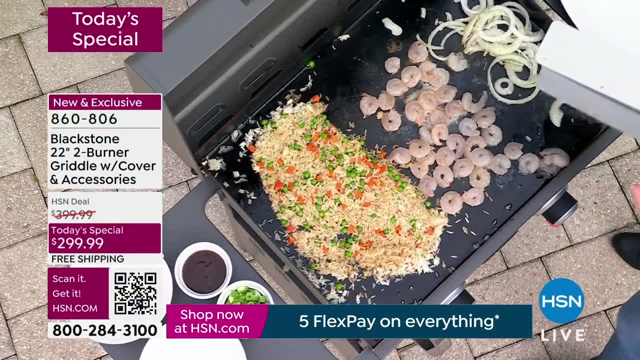 But then, now that I've learned to do it, times have changed. Yes, When you look at the sodium content, Oh, It's like 3,000 milligrams of sodium you're intaking per dinner, And that's just one meal. 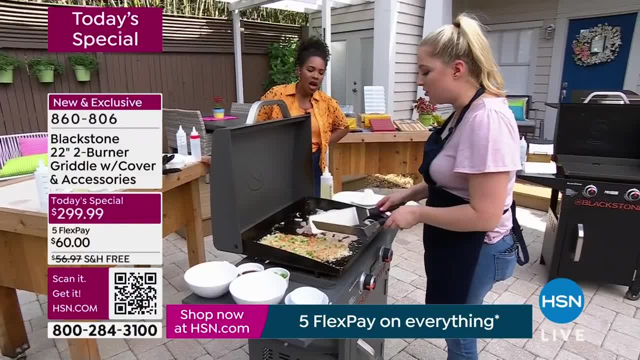 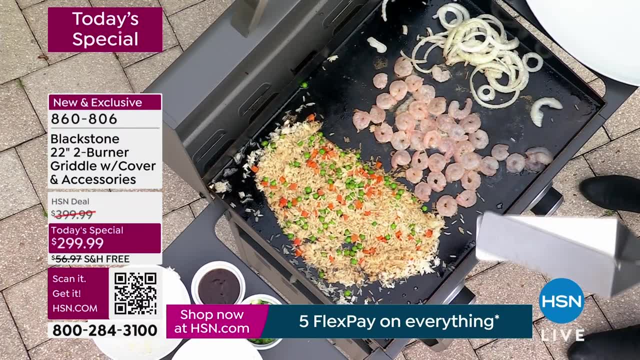 And that's on the low side. I've seen it as high as 6,000 grams of sodium, I believe it. So with this I'm in control of my sauces. I'm using a more low-sodium sauce, no-sugar sauces you can grab. 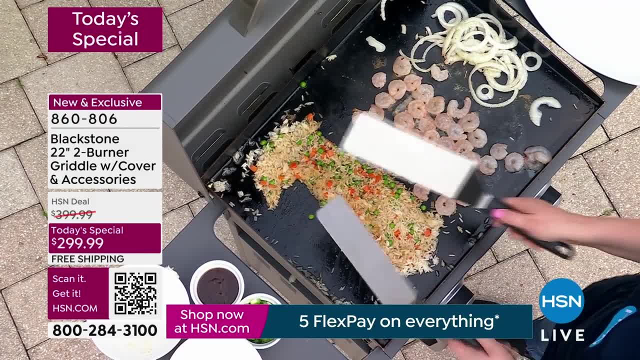 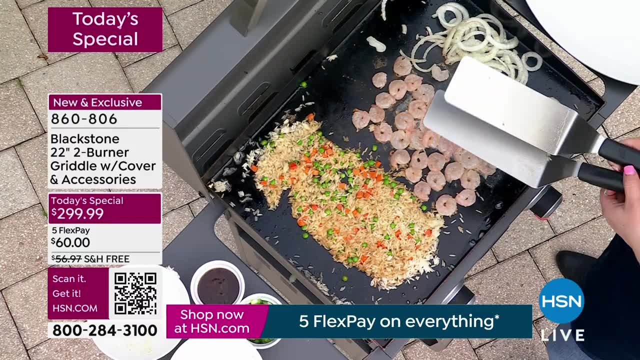 There's teriyaki sauces that have all sorts of, you know, sugar-free, but they have tamarai sauces that are also better for you, like cocoa Aminos, things like that. We've got flying spatulas out here. 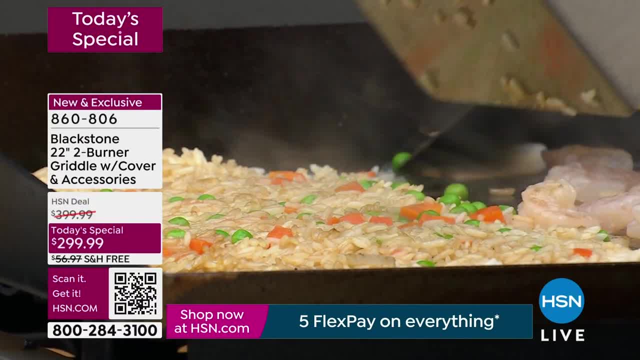 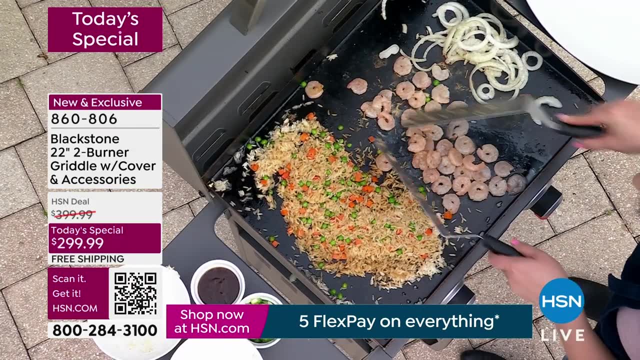 Even the spatula's hungry, I know right, And so that's why I say you're really in control of what you're eating here, but you're still being able to put out those same exact flavors as you would be going to a hibachi place. 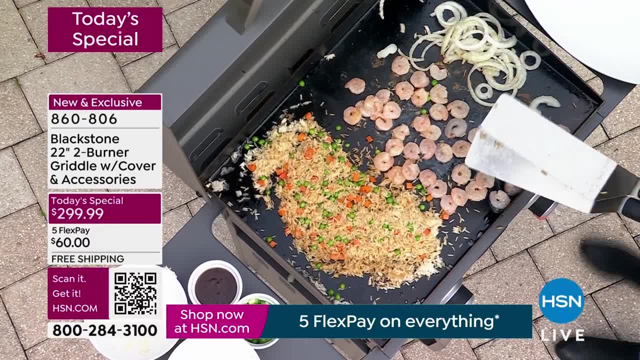 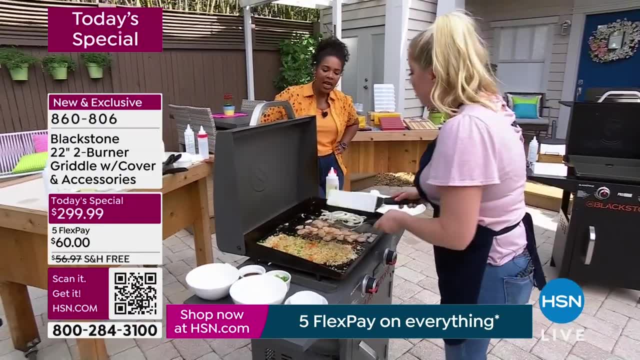 And your daughter. she's going to be like Mom, you are so cool, Yes, Like I cannot believe. you are out here cooking a full hibachi meal, Right, And she can be a part of it, And you don't have to wait for just. 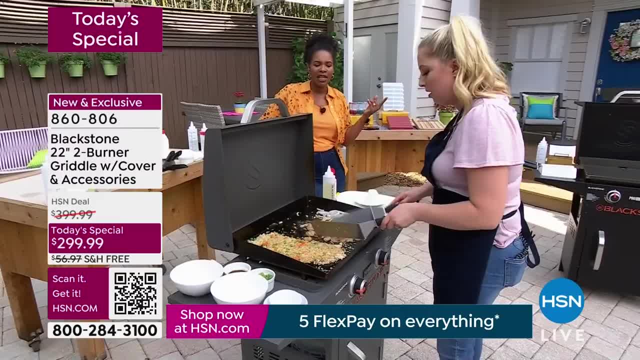 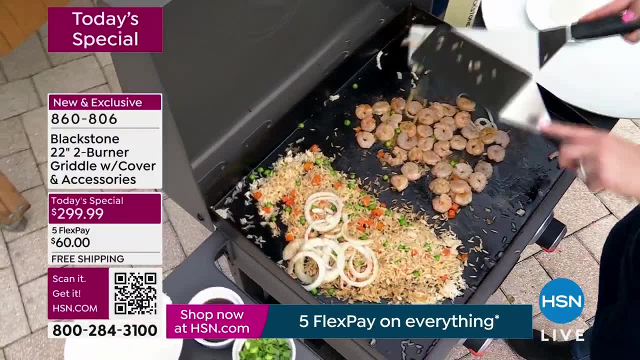 on that one time a year when it's your birthday and you splurge a little bit because we all have our favorite things, but we don't do our favorite. we don't eat our favorite meals nearly enough because they're expensive. We have to go to that one restaurant. 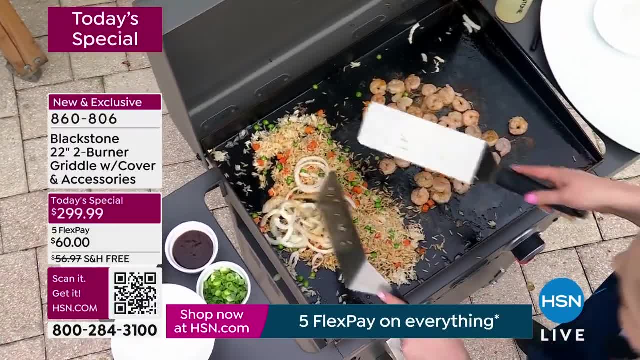 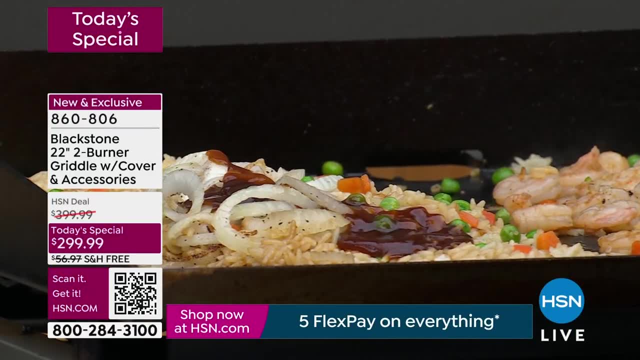 There's always a wait list. Yes, All the things. It's an ordeal. Now I can do it at home on that same random Tuesday- Maybe this is a Wednesday, I can do it any time I crave it, Any time you have day-old rice, you know it. 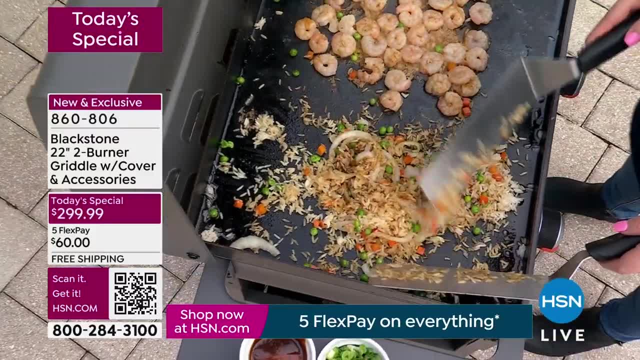 you might say: you know what? I'm taking this out to the griddle. Yep, that's all There is to it. I literally, when I have day-old rice, I have extra and this is what I do. I'm like: all right, I know what I'm going to do with that dinner. 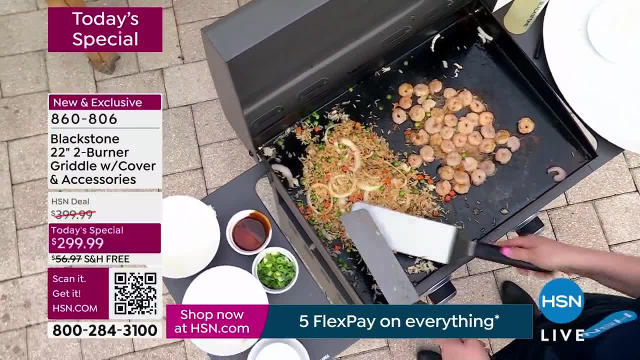 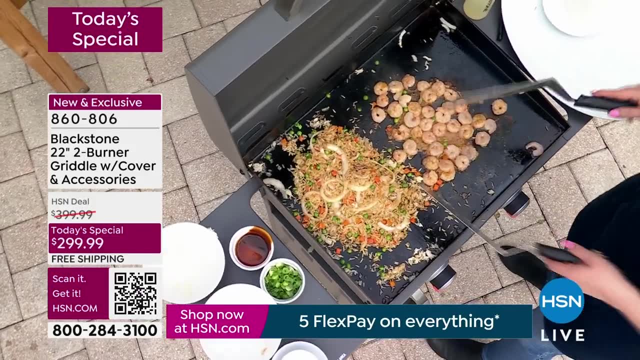 It's my husband and I eating, Yeah, But if you're feeding a drone of people and you're looking for a cheaper, budgeting way to do it, but impressive to impress your guests, here's where it's at. You want to do something like this because it feeds a lot of people. 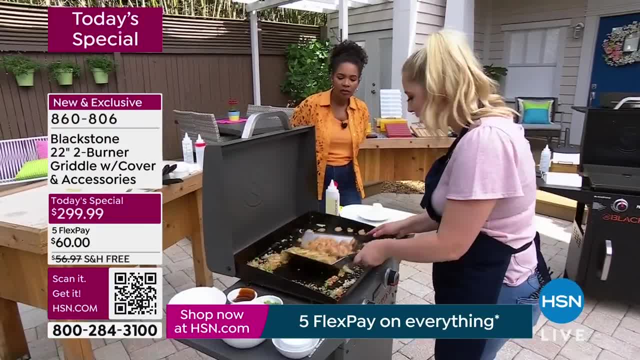 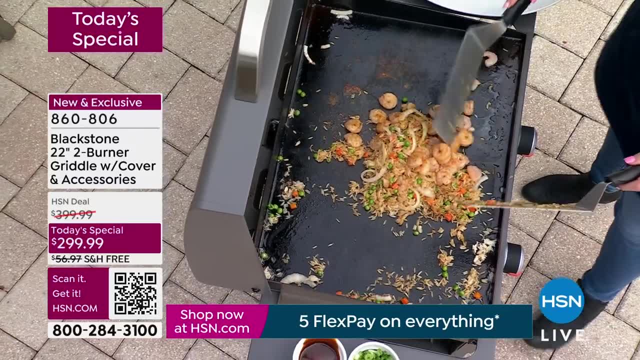 It's impressive, like I said, but most importantly it's quick. Watch this: I'm just going to mix everything up. It takes a matter of minutes for shrimp to cook, which I love. It's just a quick protein, especially when I've got a baby on my hip. 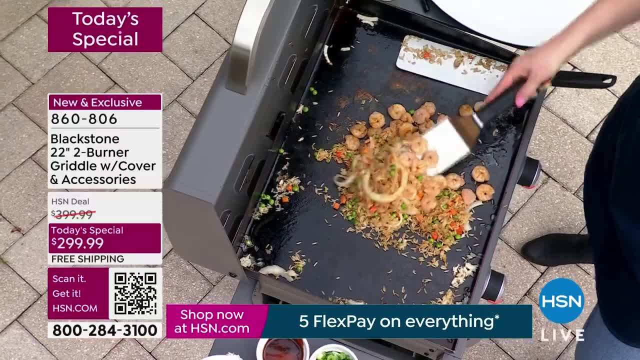 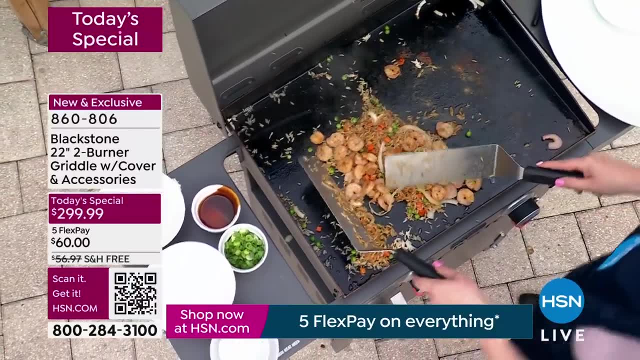 Literally, I'll be like this: I'll be with my baby and I'll be like this right, So it's for anybody, and I promise you- I know it can be intimidating at first to try something new Tamara and I were talking about in the hallway, how you know. 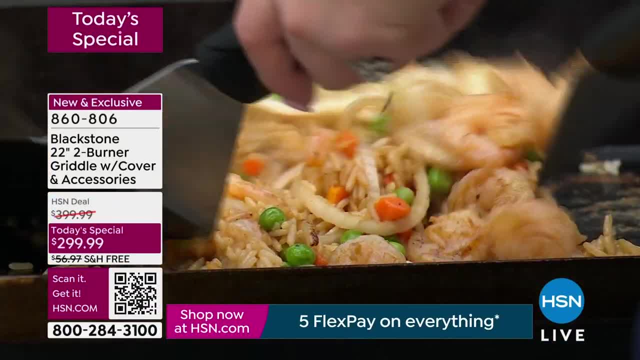 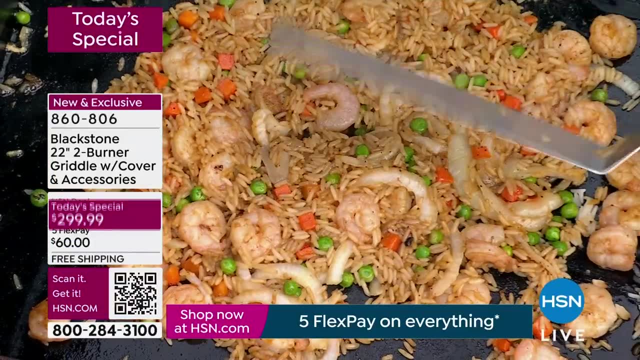 there's some people who are. of course, it's normal to be nervous about a new cooking product, right, You're not used to it, Right? But once you get the hang of it first or second time cooking, that's it. 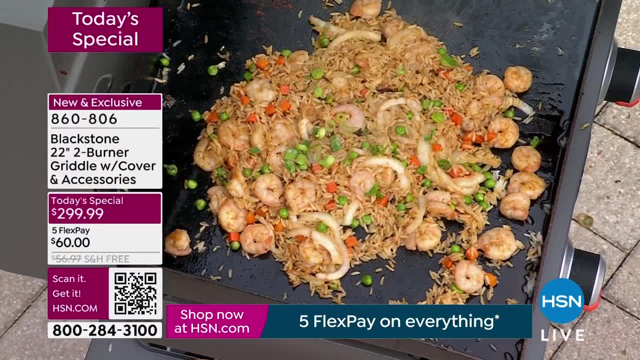 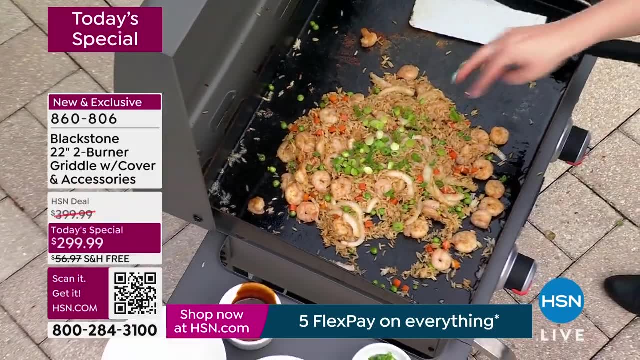 And you are confident, You are comfortable. You're never going to want to go back cooking in the kitchen because when you realize there's no cleanup, there's no splatter everywhere- Yes, That's the name of the game- right there, The whole house doesn't smell like shrimp in this case. 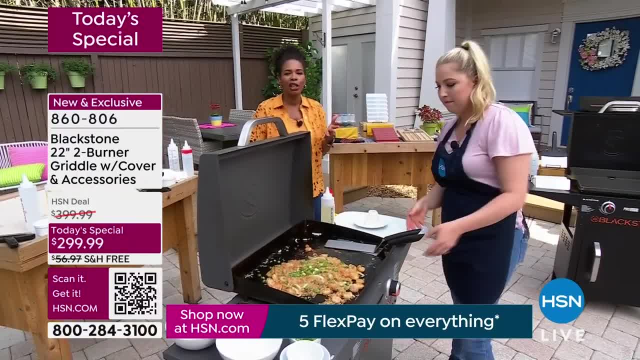 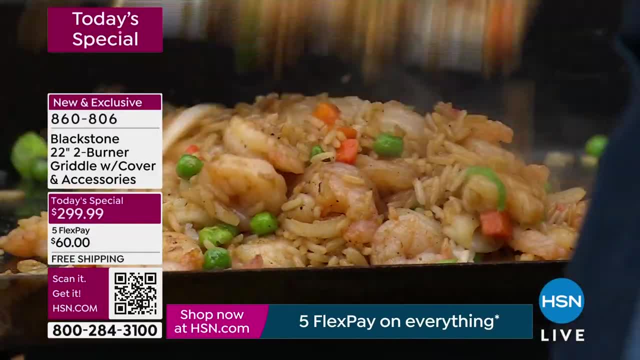 You're not worrying about all the pots and pans, because it's always the person who does the cleanup who can't relax and eat like everybody else, because you're thinking: with every bite you eat, you're thinking: I still have to go do the dishes now. 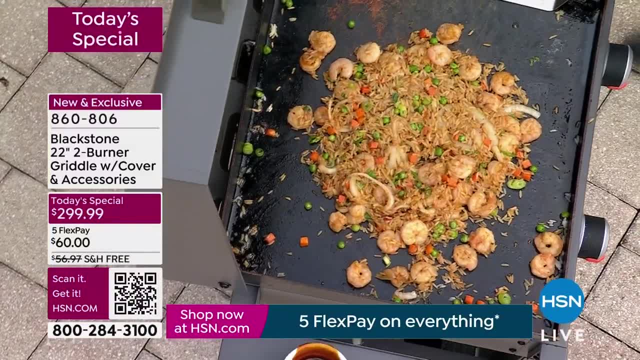 Yeah, and it's piling up. You're full, You're tired, You just want to relax and you're like, oh my gosh, Yes, Everybody's going to leave, I'm going to be stuck cleaning up the dishes. 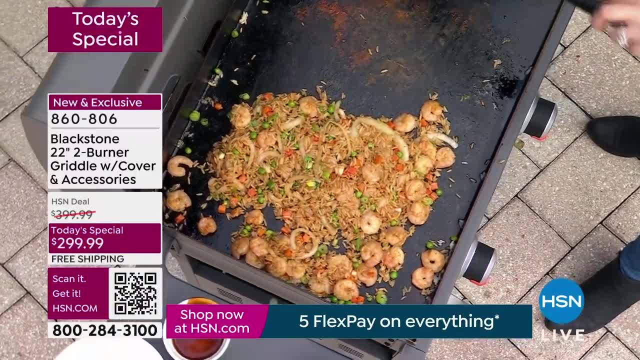 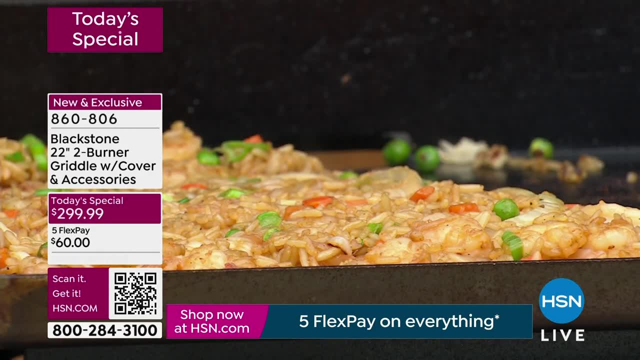 No, I've been saying this a lot because it's so true. but my husband, he always tells me: honey, this food was wonderful, It was so delicious, but now I got to do dishes. Yes, And I say that's the name of the game. 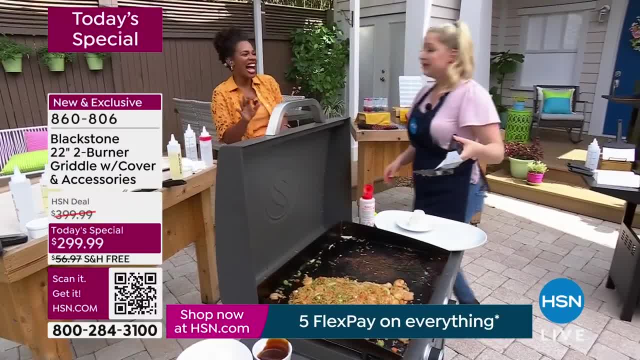 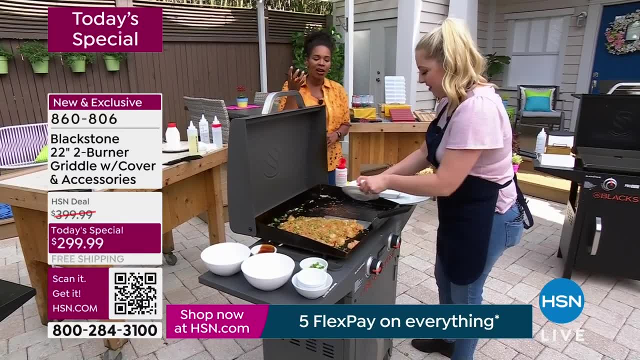 And now he goes: are you cooking on the Blackstone tonight? Because he knows there's not going to be any dishes. That means it's an easy night. All the food's done together. All the food is done again. We talk about restaurant quality. 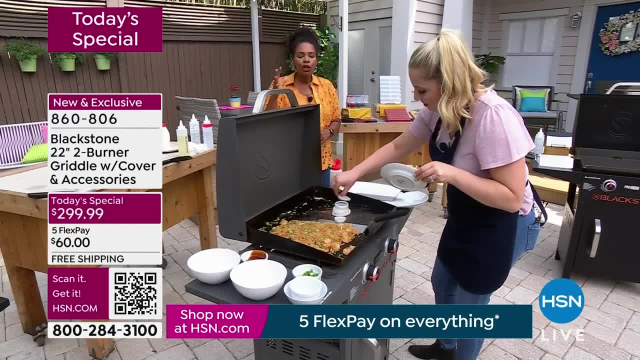 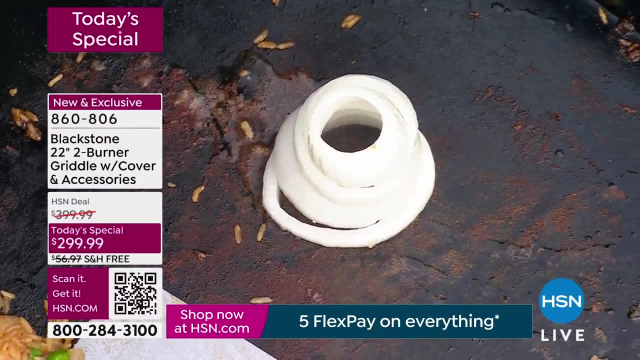 We talk about ease of use. And to Taylor's point, you might look at her now and say, oh gosh, she's really good. She can just easily flip those around, But you will be able to as well. It doesn't take a long time to get comfortable with your Blackstone. 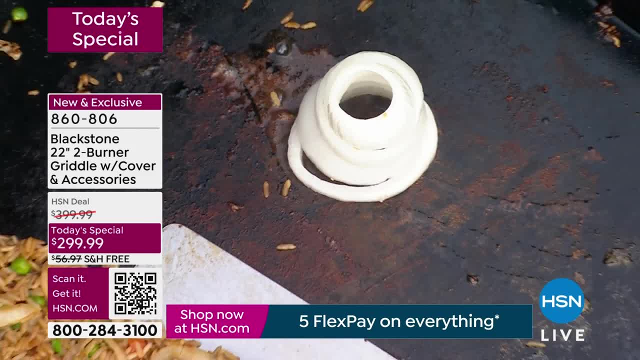 And that's what I really want to impress upon you. There is no open flame, No open flame, except for this. I'm about to do an open flame. I had to warn you, girl, This is just like at the restaurant. 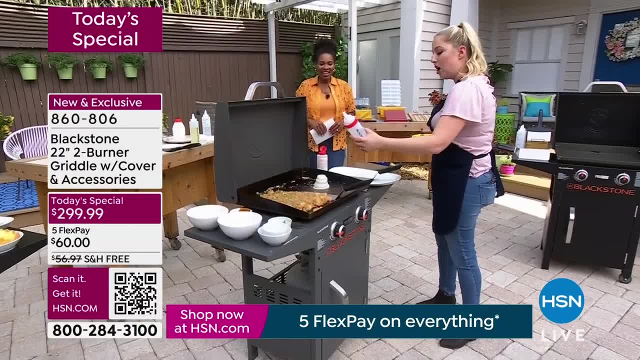 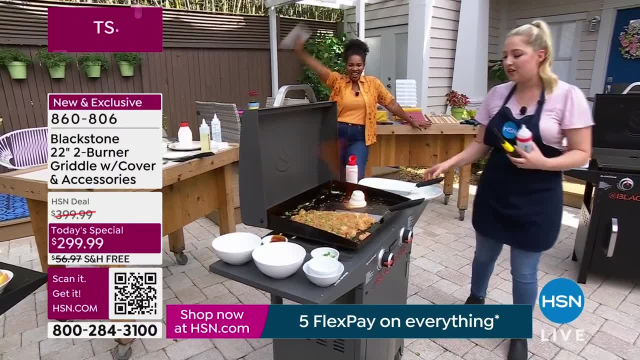 So if you go and you do the volcano, the stacked volcano, they use 100%, They use 100 proof alcohol. Oh, is that what they use? I'm going to do a little bit more Ready, Okay, And just like that. it's such a cool thing to do for the kiddos, for the grandbabies. 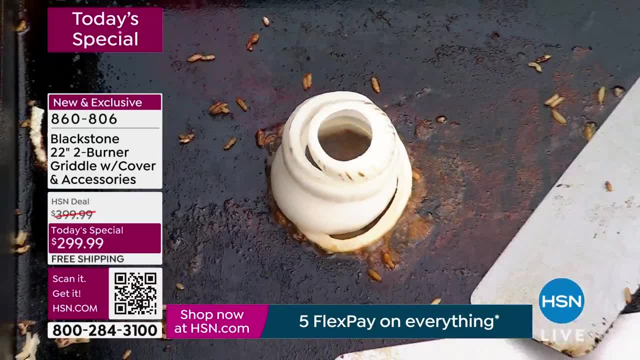 They do the choo-choo-choo And they do like the. you know what I mean. Yes, And then, if you want to put it out and be safe, just add a little bit of water and that's it. 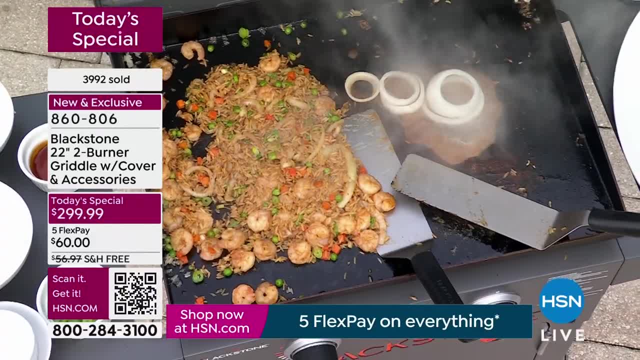 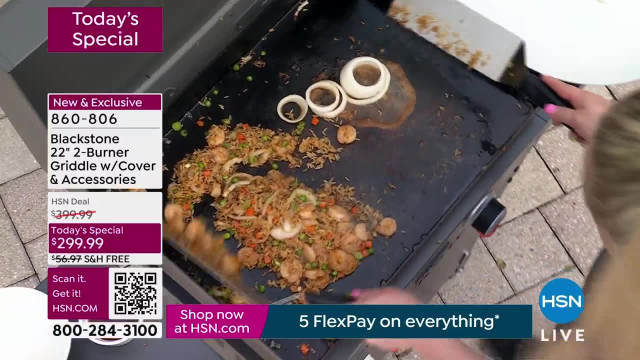 That's simple. It's that simple And we pay a lot of money for that. We pay probably $10 for that experience on top of the meal. They added it. You know. they added it When you know you can do it. 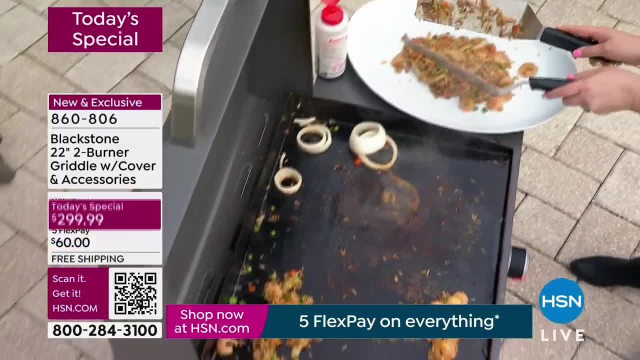 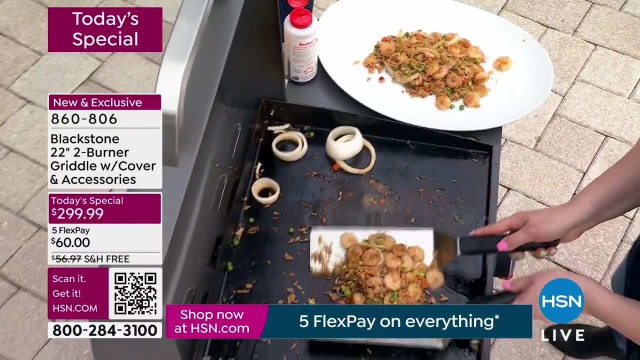 So this is the deal. We've got it for you as our today's special. I'm glad that so many of you have already said you know what. this is what I've been looking for. Even if you have a grill like a traditional grill, I think you're very likely going to use this one even more. 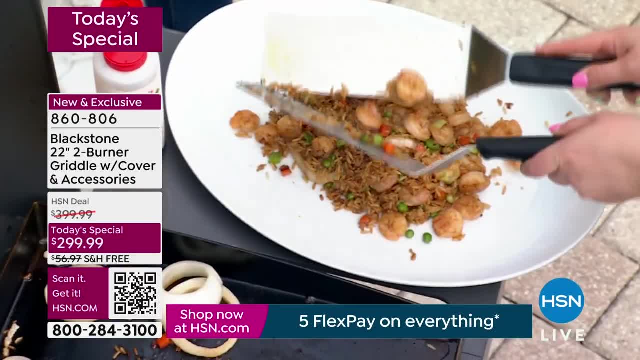 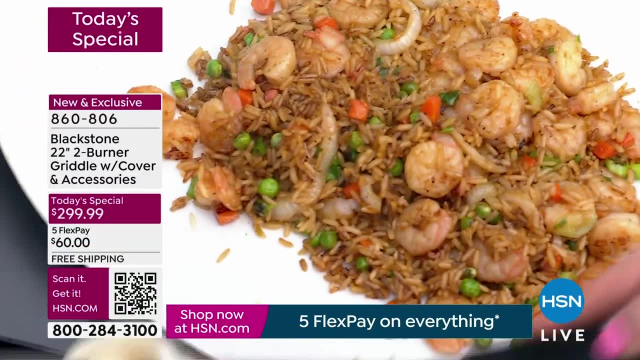 You're going to use your griddle even more And they can live right next to each other if you choose to, But because you can do more of your meal. usually for the regular grill, which we love, it's just the protein. 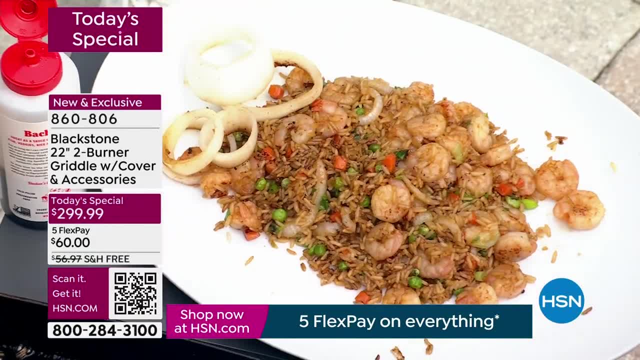 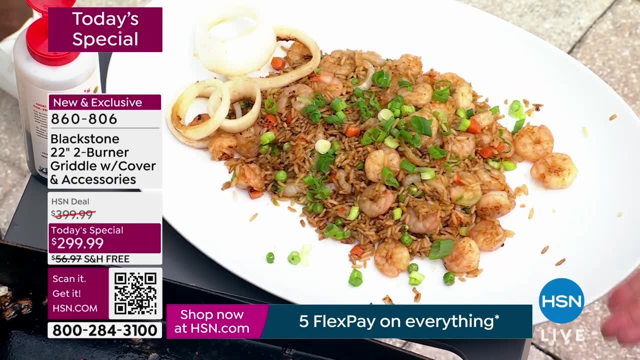 Yeah, This is the entire meal And that you did right here, right in front of us, Yep, And you don't have to wash a single pot or pan, Nope, Just my spatulas. And, honestly, I just usually wipe them off with a nice cloth. 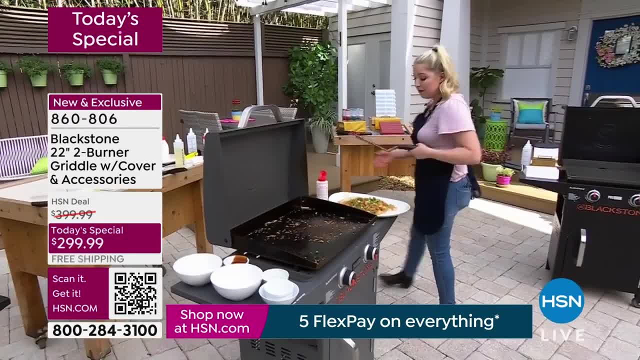 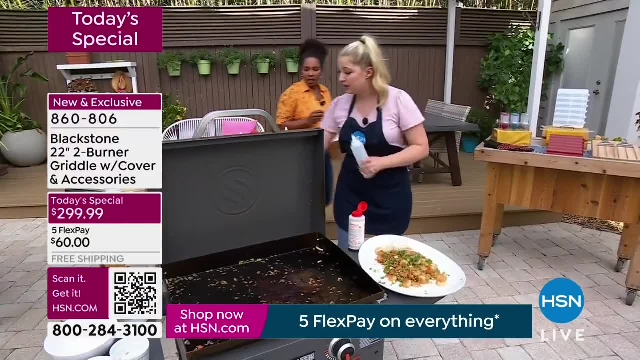 And that's it. Let me get a fork. Get a fork And this can feed easily. I could triple this recipe and feed up to 15 people. I've done it plenty of times. Yes, It is such a statement piece. 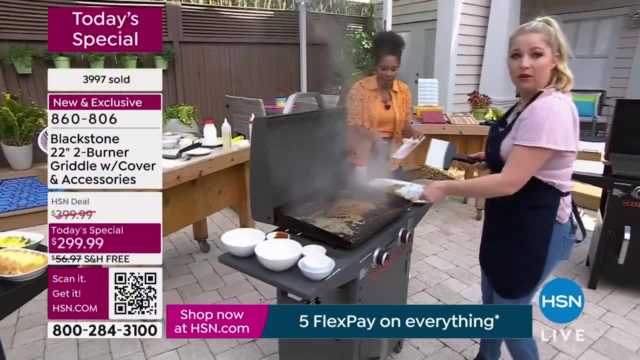 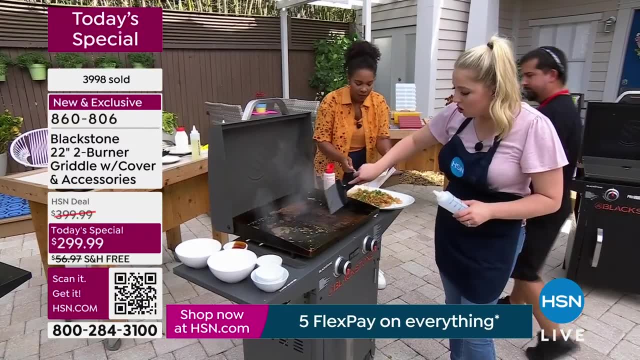 It is such an entertaining piece You want to come on in. Yeah, You guys, go ahead and taste it. But here's the beauty, It's the cleanup. Do you see all this stuff? These are what's called sugar reductions. Okay, 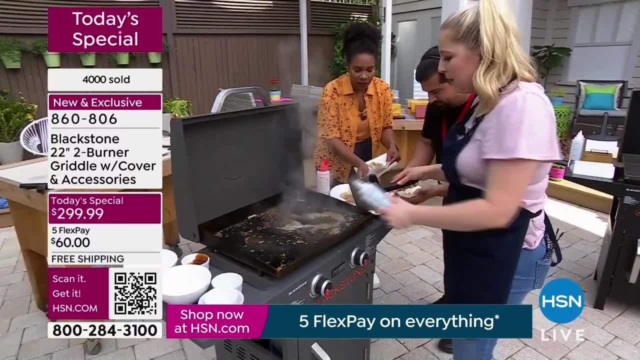 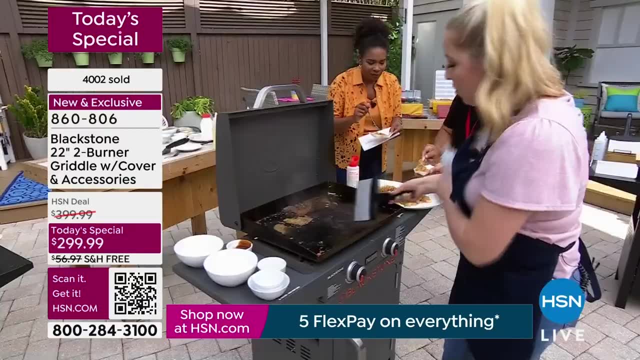 So this is what we want to get off the griddle. Add a little bit of water And it just scrapes away, And so you're going to do that until everything is all clean here. You want to make sure your griddle is more on high. 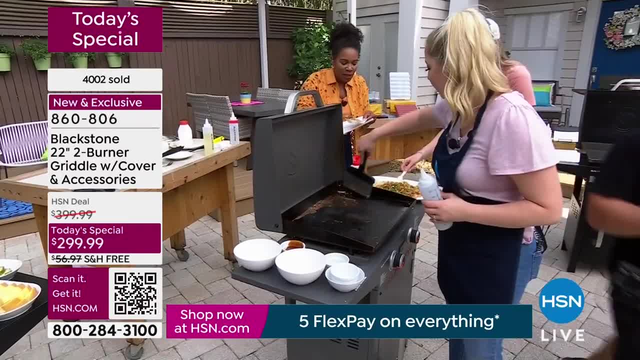 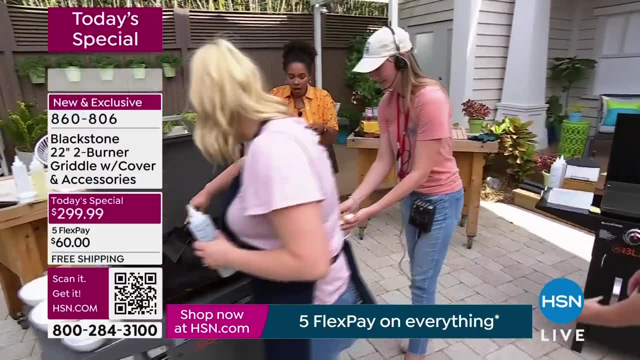 Yes, And that makes it easier to clean. How is it We're about to dive right in? Okay, Let me know. Let me know If you're at my house, It's so good. Would you be impressed? And it's so good. 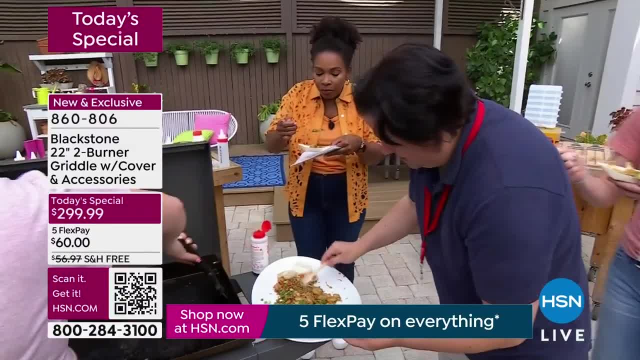 Thank you. I'm glad you enjoyed it And it was fast And we watched you do it. I know That's the thing You watch the whole time. It's entertaining. You're over here drinking your wine And I'm over here entertaining you. 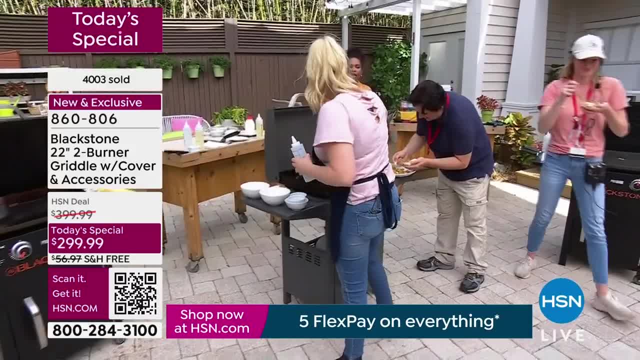 This is fantastic. You know what the funny thing is At home when you're cooking, when you have family over? Uh-huh, Everybody's in the kitchen anyway, aren't they? Oh, exactly, And they're all like bumping into you. 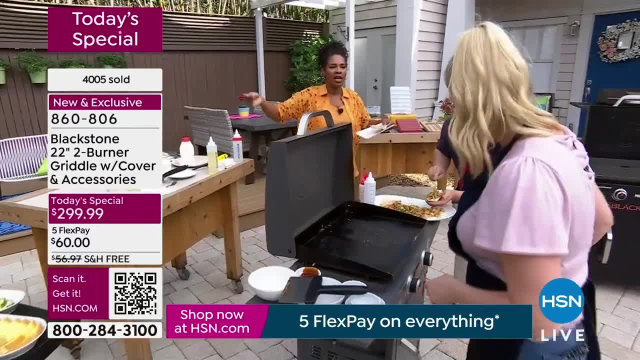 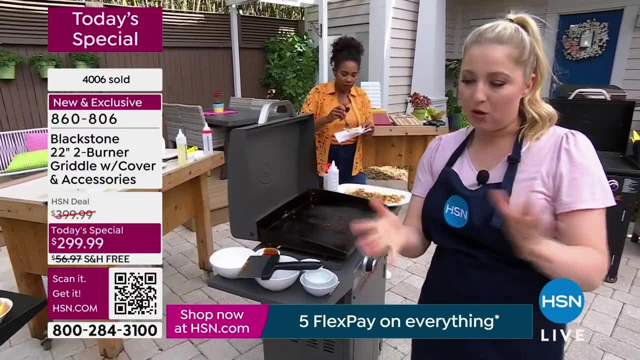 They're kind of in the way, But when you're outside, you welcome it Absolutely. It's an experience together which I absolutely love. That's what makes the Blackstone journey so incredible. And hey, I don't know if you know, but I actually have my own cook show for Blackstone. 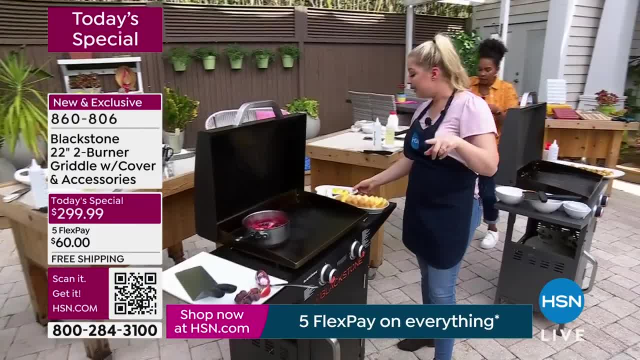 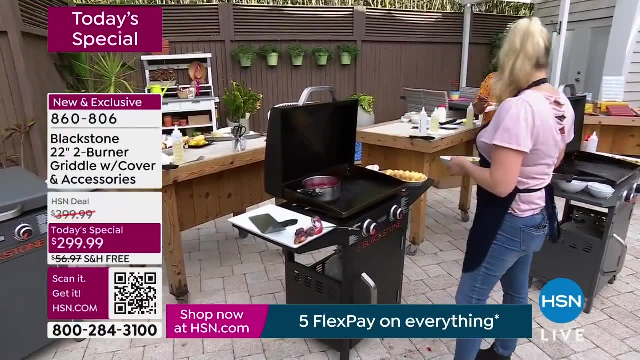 If you're looking for new recipes, I've got you. It's called Easy Weeknight Meals with Taylor Mock. You can find hundreds of recipes on there, But I'm going to kick you off a little dessert. Oh wow, Now you had some. 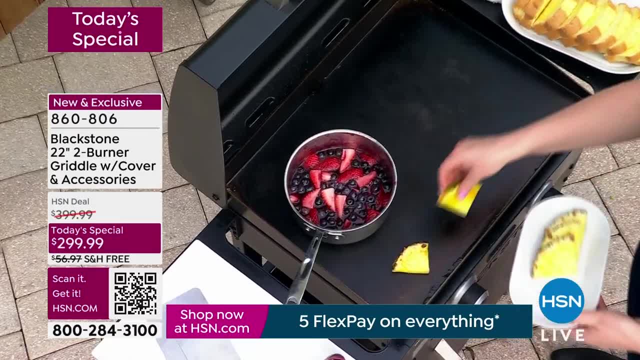 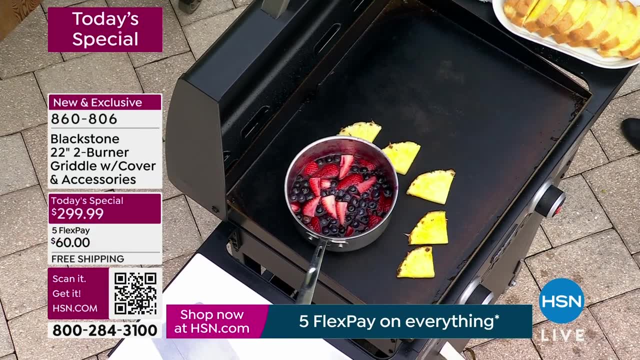 Wait, let me tell you real quick. I'm sorry She's like I'm enjoying this stir fry hibachi. I'm all about the dessert, But let me tell you bronze is now spoken for. okay. I'm so glad for all of you who were able to get bronze. 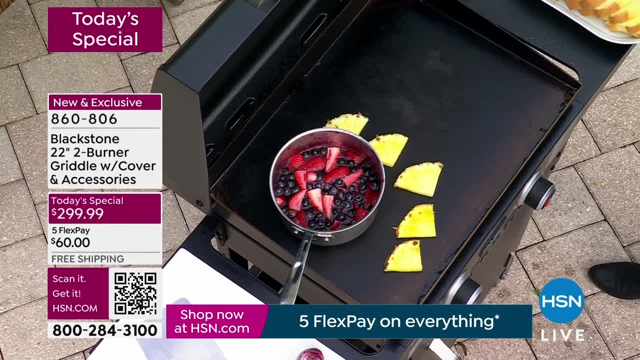 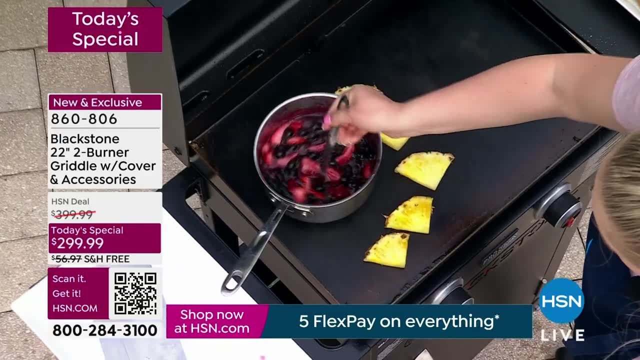 We still have black- and that's the one you see right there Taylor using- And we still have the gunmetal color. They all cook exactly the same. So if you missed out on getting bronze, then choose one of the other two, because you can still get all of the convenience that this is giving you. 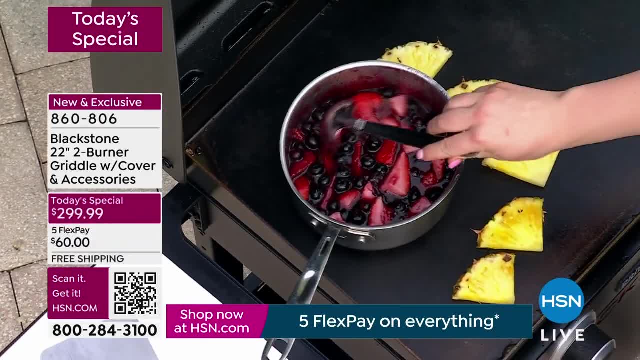 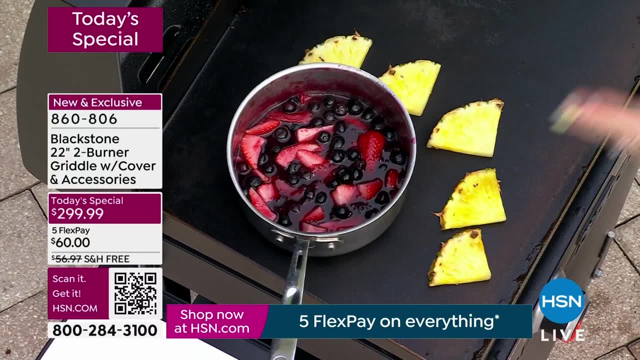 I'm telling you: this food is so good, I'm so glad you're enjoying it. You could charge us and I would pay. Oh, I love you. Let me think about this, That's right. Okay, so we've got to think about not only. 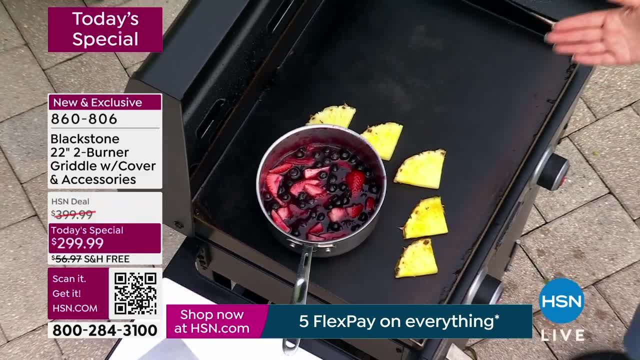 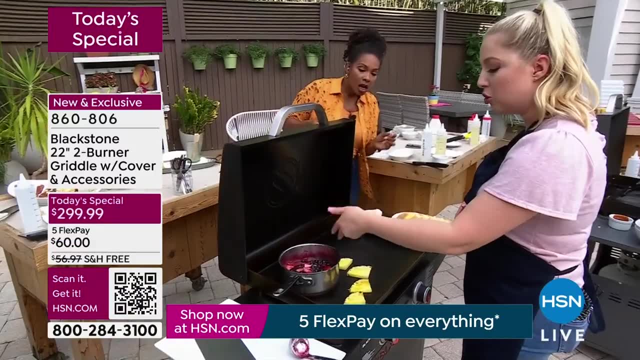 is it a flat-top griddle, but it's also it's your stovetop, okay. So if you want to do a sauce, whether it is a strawberry, blueberry, raspberry compote, I have some jelly, some sugar, some blueberries, some strawberries in here and that's it. 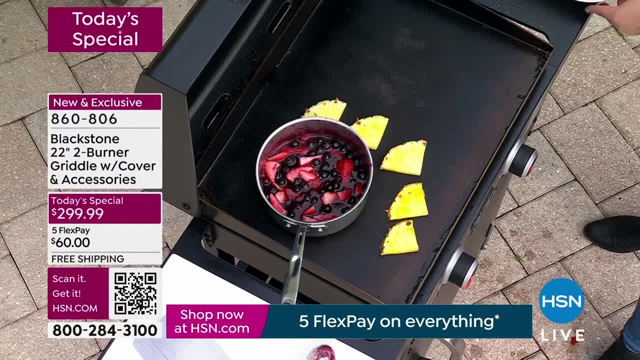 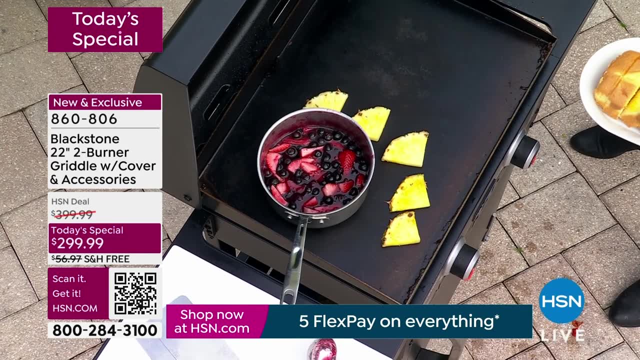 Because this is the season for those now. Yep, I bought- pre-store bought already sliced, because mama don't got time- pound cake, And so all I'm doing is I'm simply toasting the pound cake and I'm adding that reduction on the side. 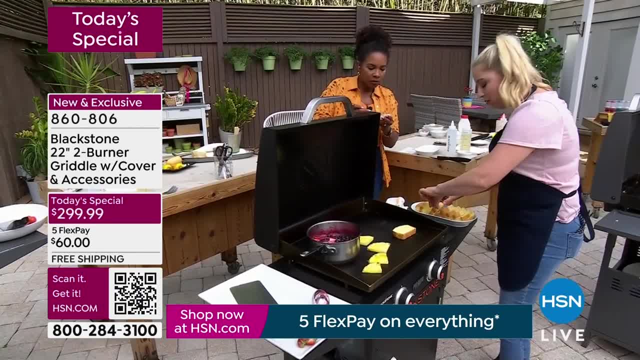 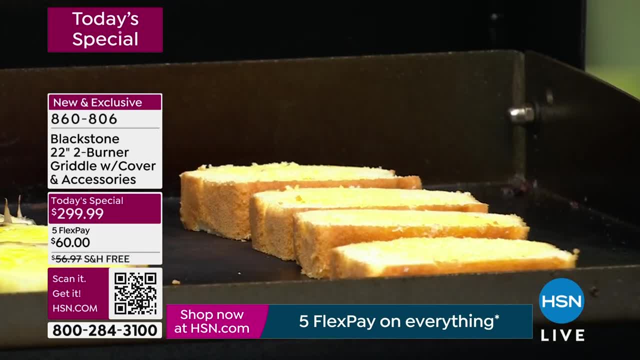 So I'm just going to lay flat. I pre-buttered both sides. Oh my gosh, This is such a good little hack: Butter and pound cake. And your family, your friends, your girlfriends- they can watch you do this. 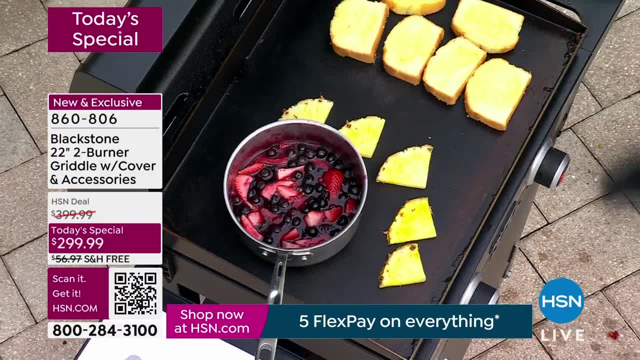 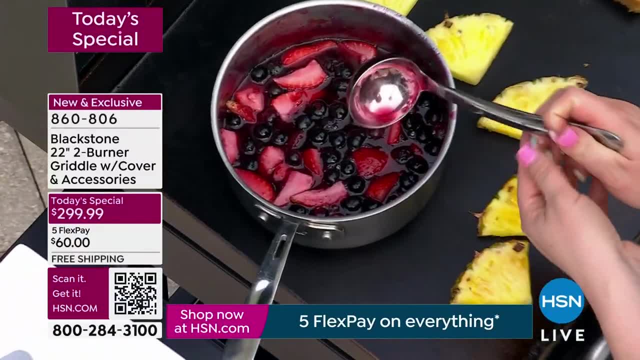 and they'll be like: wait a second, you just did that on the griddle. I'm like: absolutely, And this has been cooking down for about five minutes. So, whether it's chili, I love making hot dogs and then chili on the side. 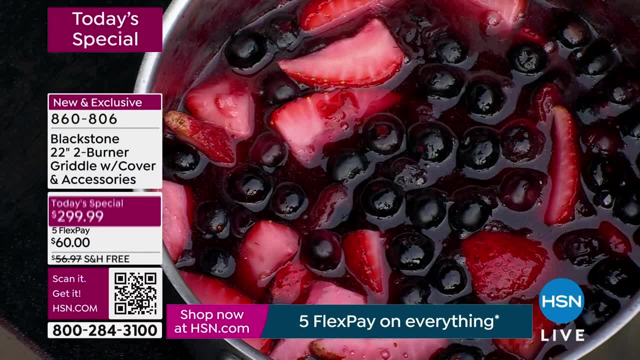 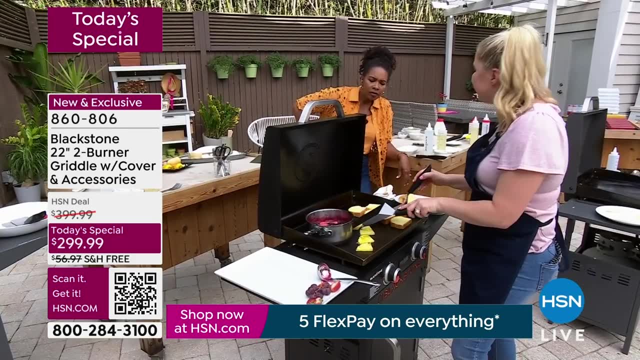 and then I'll have a cute little bar set up. Yeah, With chives and green onions and cheese, and it just makes for such a presentation. Yeah, But again the cleanup is like minute. Yes, I mean, look at all of this. 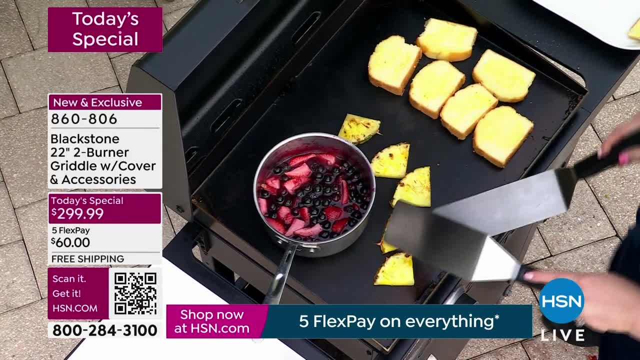 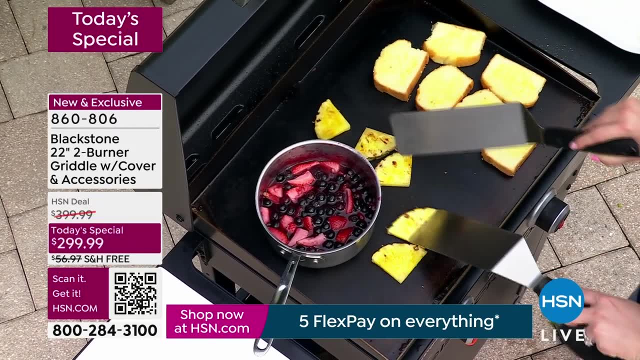 So, if you missed the beginning of the presentation, Taylor did steak and eggs for breakfast. and I'm not talking about just any steak. These were those big, thick Curtis Stone steaks, Yep, ribeyes, Ribeyes with over easy eggs with maple bacon. 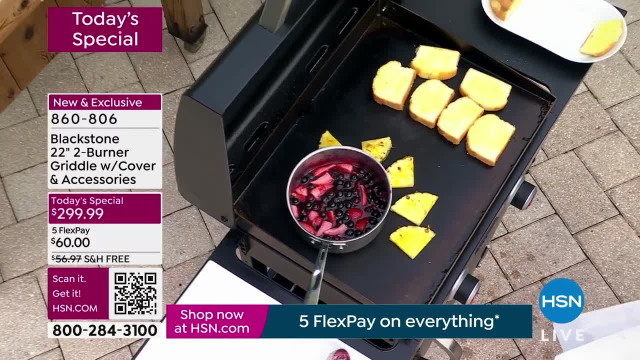 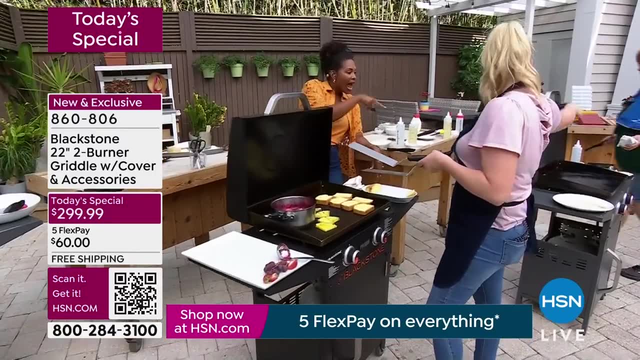 All on the same griddle. And then she scraped it off, Yep. And then she made smash burgers and Philly cheesesteaks and sausage- I mean peppers, Yeah- and then the hibachi. And then you did your hibachi. 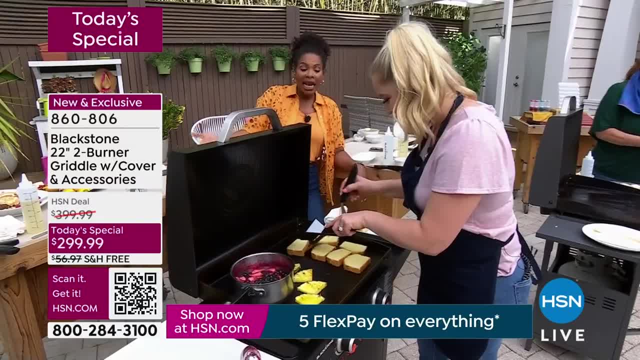 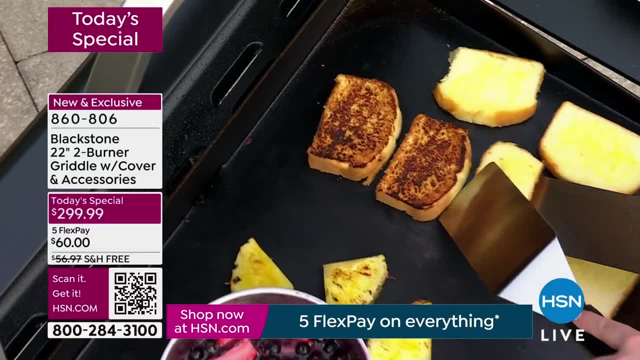 And now I'm doing dessert. I mean all on the griddle, I know, And she does not have to wash a single dish when she's done. Nope, And all of the food is delicious And you're controlling the temperature. 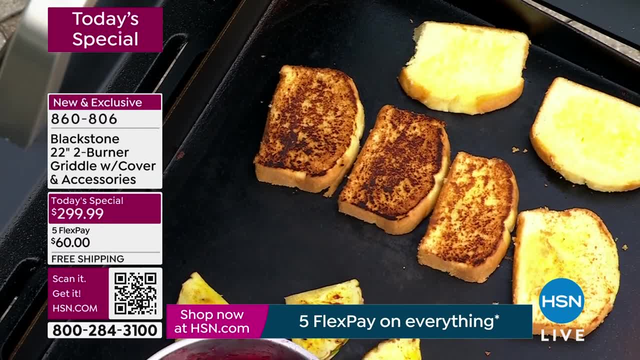 That's right. It's not just fire. So a great point. I have this on low Yep, Because I'm simply, I'm simply just toasting, right, I'm getting these browned up. I don't want them to burn. 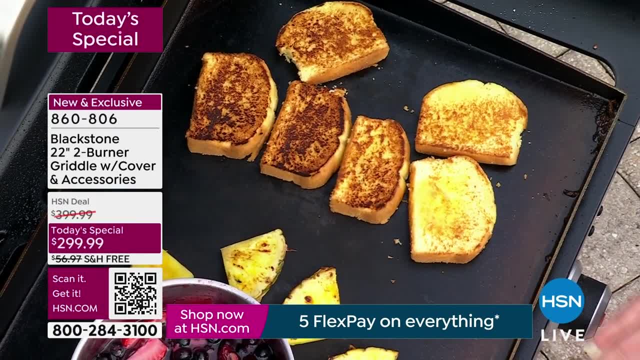 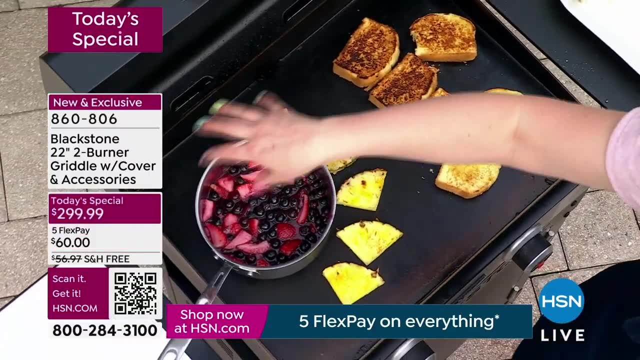 I want them to get nice and crispy toasty. Okay. So I have this on low for this side of my right H burner. On this side, I have this on medium low because I want my compote to continue to boil. Okay, let's plate, because we all know we're all ready for it. okay. 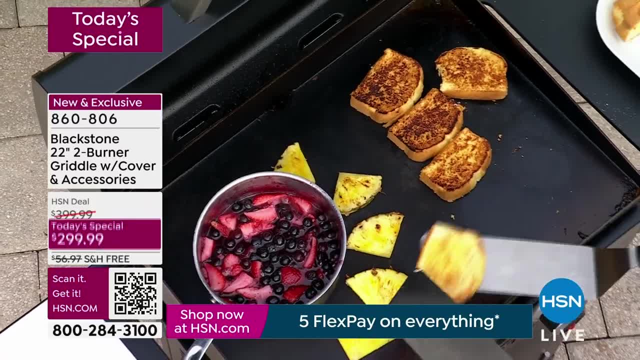 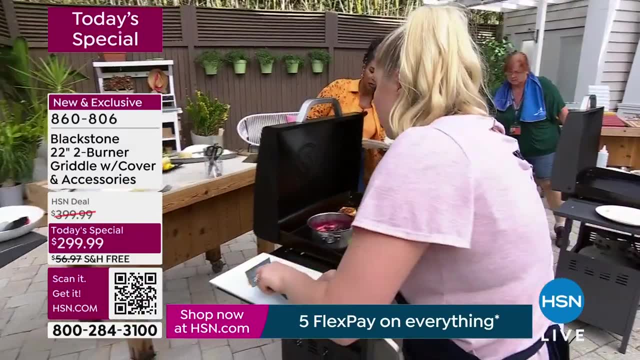 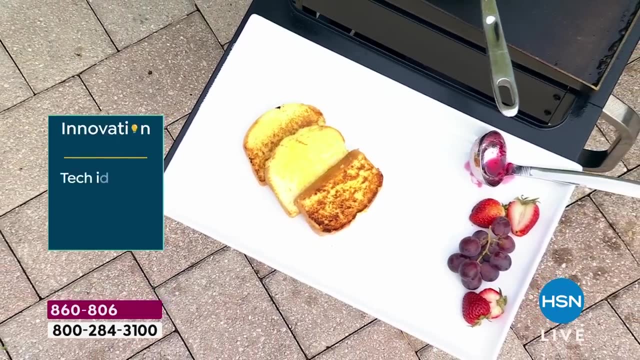 So here's how I display my dessert. My friends are absolutely enjoying their time. They're drinking their cocktails- Maybe it's mimosas. This is for a fun little brunch. This is also great for any kind of neighborhood get-togethers because it's easy. 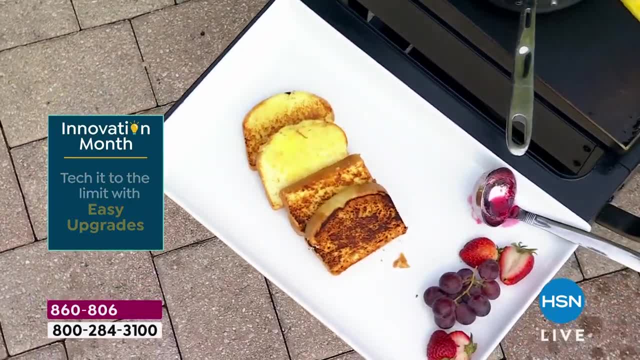 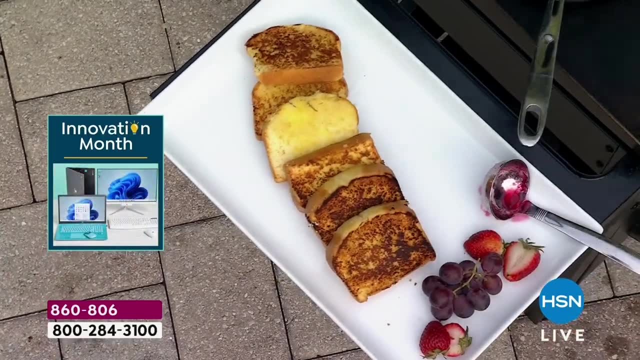 There's really no thought to it, You're just, you know, easily stacking on a beautiful platter here. I love being able to add those colors to showcase of that compote, with those colorful strawberries and blueberries, I'm going to add my grilled pineapple. 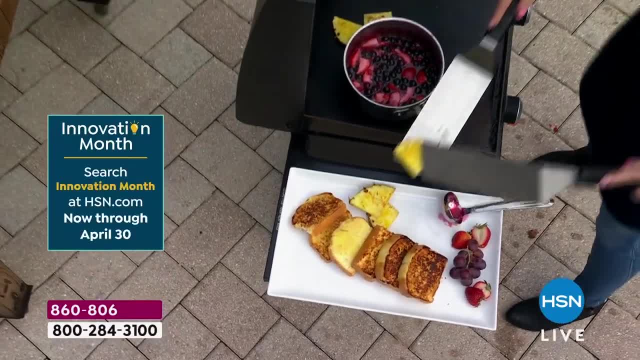 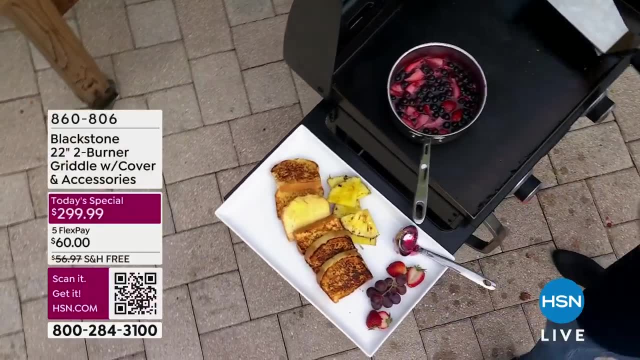 You can do grilled mango. You can do apples. I love doing apples during the fall- Yes, With my pork chops. So I want you to think outside of the box here. This is so easy, y'all Okay, Anybody can do this. 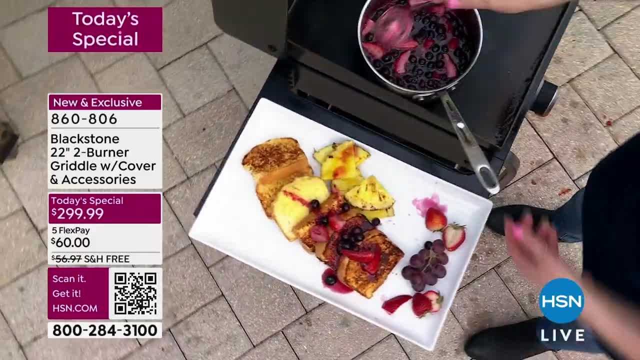 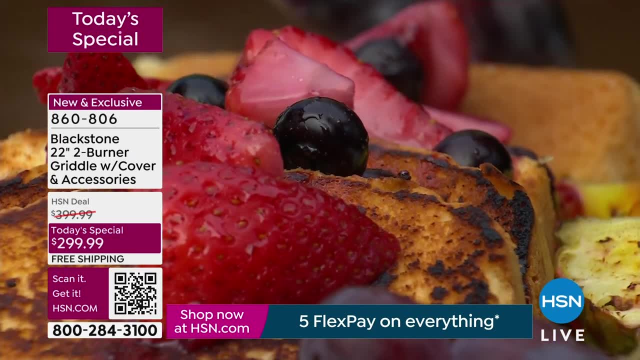 You just have to say, yes, I can. Here you go, And that is it. You add your compote right on top here. You can add it on the pineapples if you wanted to. Yes, And this just makes for such a neat presentation. 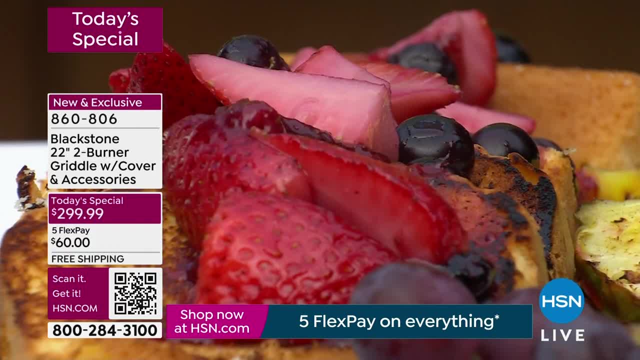 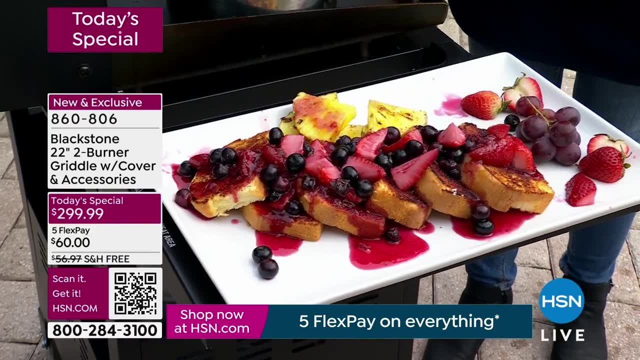 Like I said, listen, I love me some Martha Stewart, and this is her thing. She says it's all about presentation. Yes, it is. Of course it's about the taste, But you can put a Band-Aid on a lot of things. 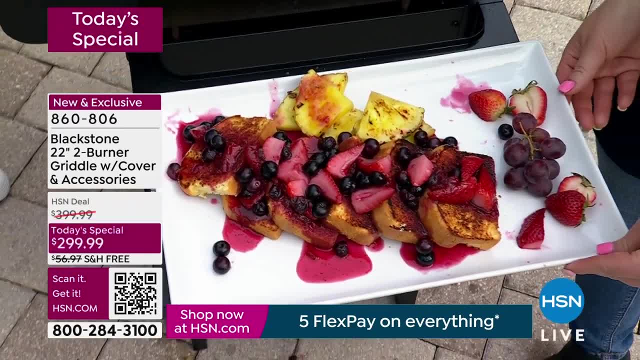 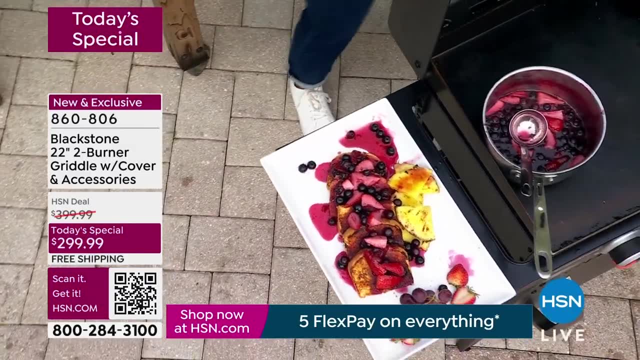 Yes, And that is a dessert right here that I always feel confident serving. Did somebody say about the taste? I'll just take this little one right here. Well, how about you tell me and you let me know what you think, because you know I haven't. 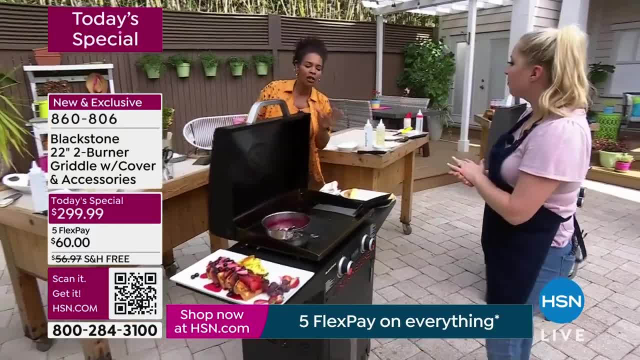 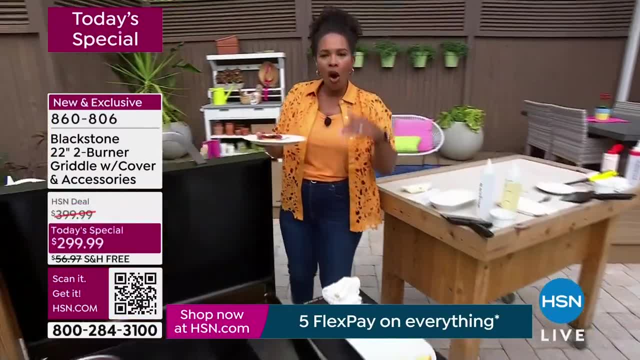 tried that one today, yet that I've made it, Your family's going to say, oh, you didn't have to go through all the trouble and truly in your mind you're like this was so easy, like it was actually easier to prepare this. 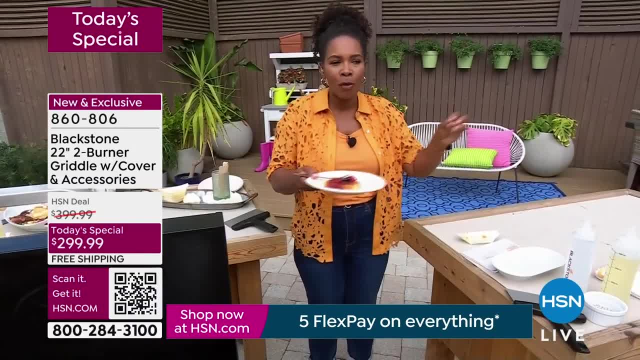 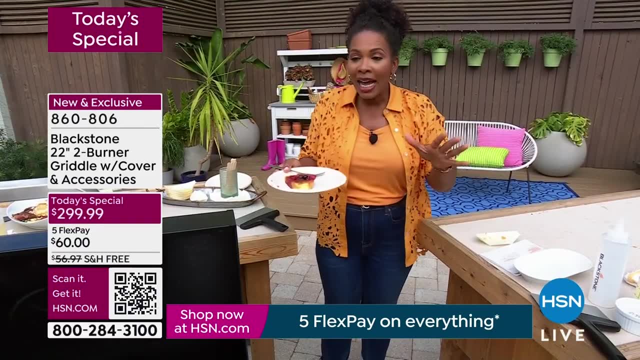 on your Blackstone griddle. Uh-huh, It would have been if you tried to pull out pots, and pans and different things and turn on the oven and have the toaster oven going in the kitchen. It was that, It was easy, And you're not smelling up the whole house. 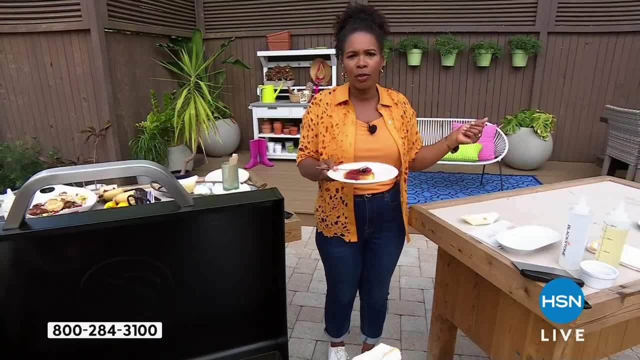 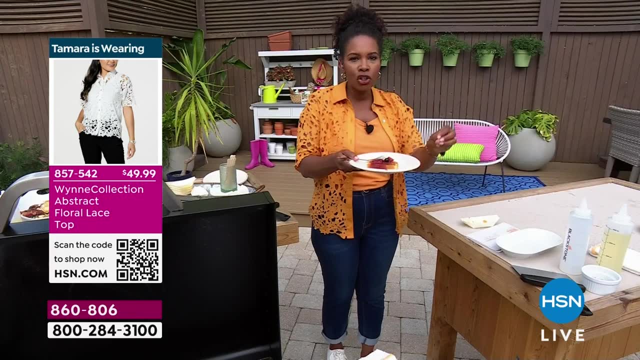 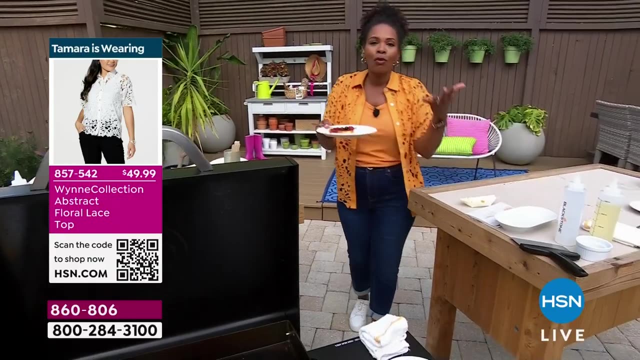 Let's say you actually burned something. Let's say, you know, oh, I cooked it a little bit too long. You're not right. You don't have that burn smell in your house because you're outside grilling and from breakfast to lunch, to dinner, to dessert, to snacks, to football games, to you know all the things. 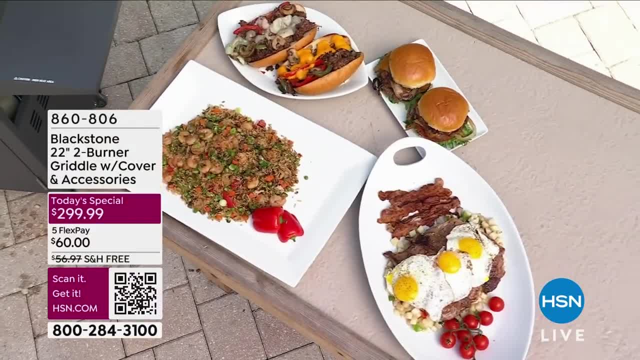 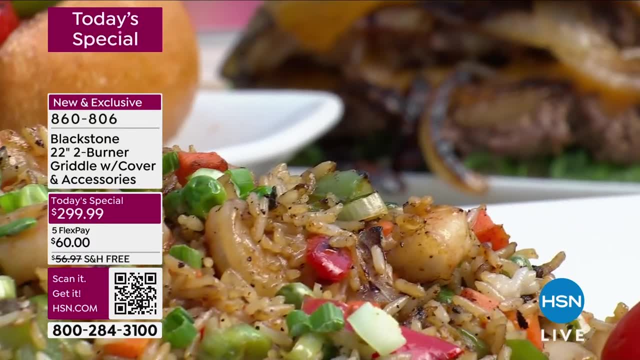 that we do All the things that are coming up. it all revolves around food And in some way, for the person who has to feed the family they have the brunt of. how am I going to do this so that I can have fun at the same time? 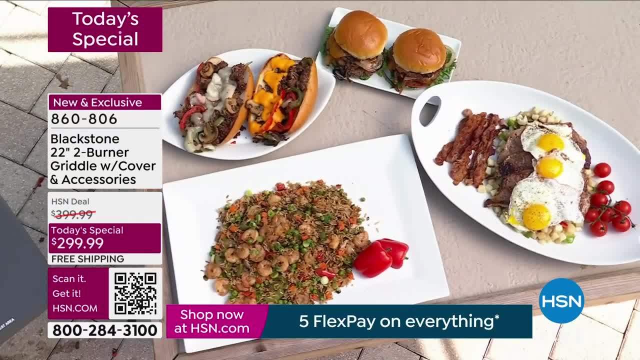 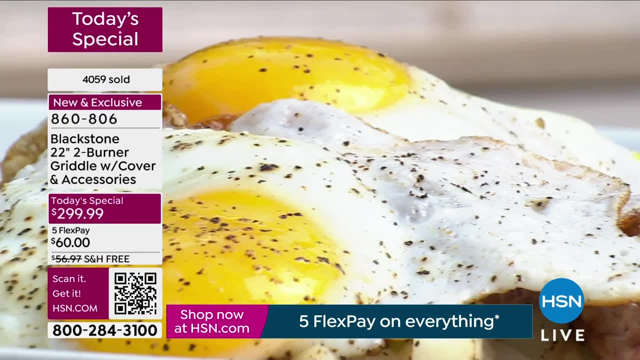 Oh, fun's all about it. This is how you do it. Yep, This is all about it. And I know that a lot of you have already shopped for your Today special, but a lot of you haven't. You're still watching and you're saying: can I do this? 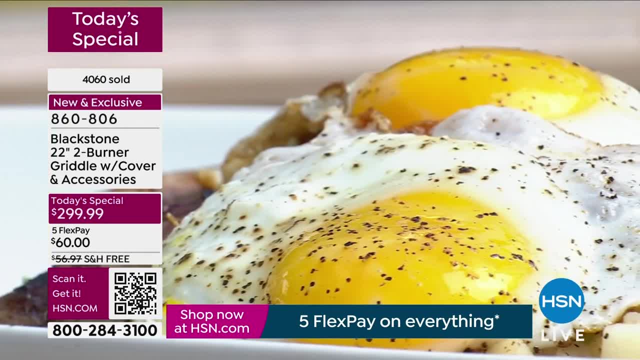 And Taylor said: you know what, If I can do it, you can do it. If I can do it, you can do it. Yeah. And then Tamara said: she's like you're, you're a pro, Right. 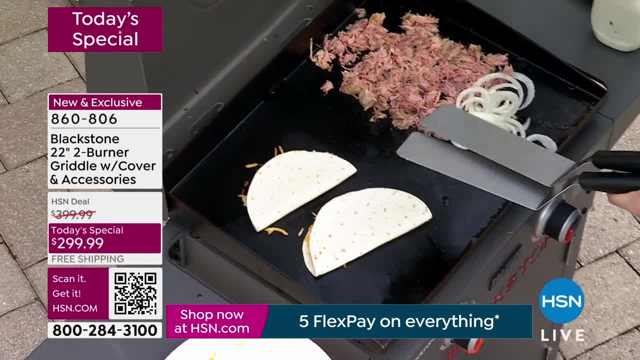 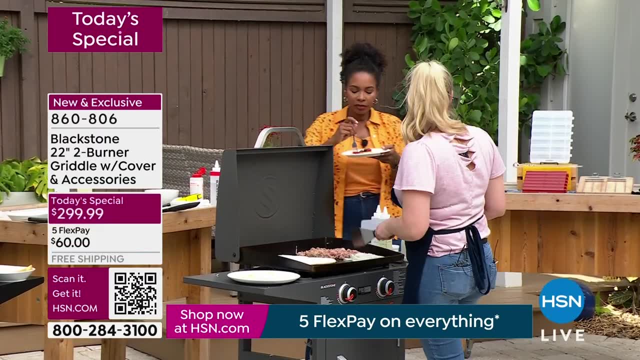 I said: girl, I'm not a pro, I just have learned to have fun on this. I've had this now for two years, So I was able. I was so confident in myself that Blackstone said: you know what? You need your own cooking show, because I became what was just a novice home cook. you know. 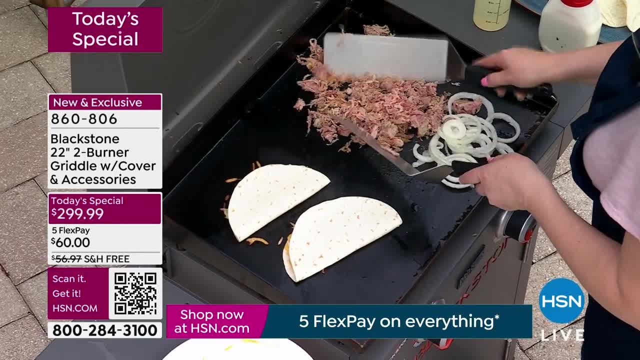 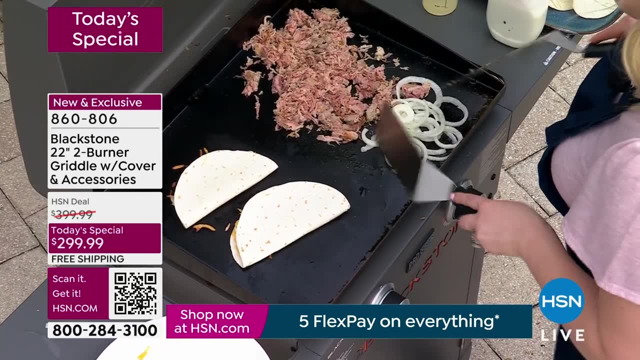 putting food on the, on the plates for my family, to me feeling so confident, to cooking really whatever I wanted, but this is my baby. My Blackstone is my baby. Yes, I can do anything and everything on my time, Most importantly on my dime. 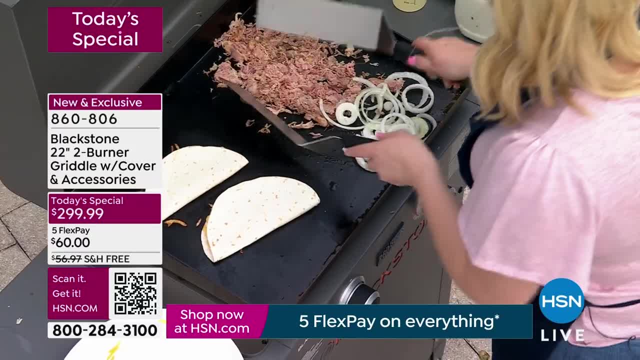 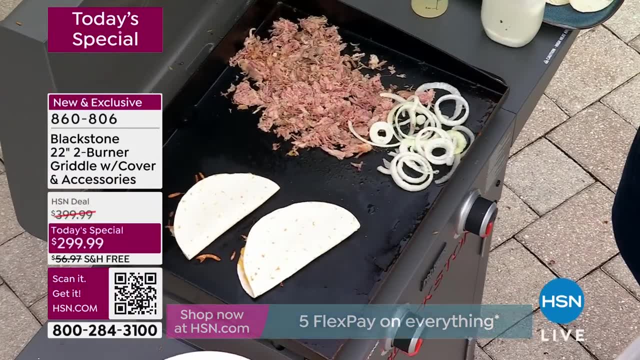 Yes, I love meal prepping, So if you are looking to meal prep for your week, the great thing about a Blackstone here is it's got this 22 inch griddle top So you could be making two pounds of diced chicken on one side and on this side you could. 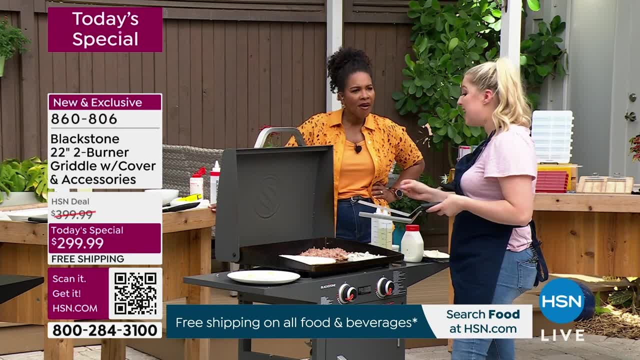 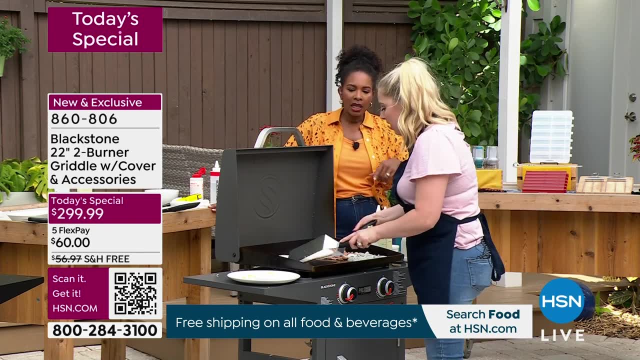 be making your pulled pork. you could be doing any kind of other protein, or your veggies or your rice- Yes, Prepping those meals for the week. So I want you to think outside of the box. I'm glad you're, you're, I mean, and I'm listening, because I need help with meal prepping. 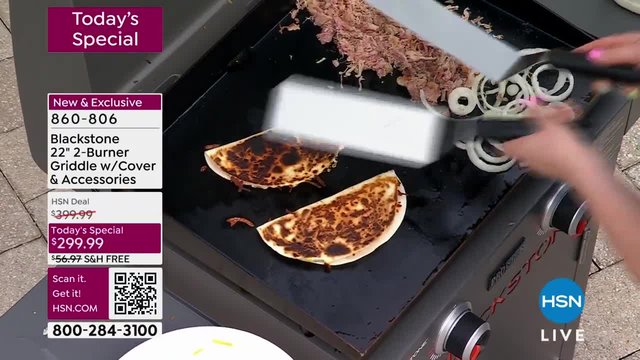 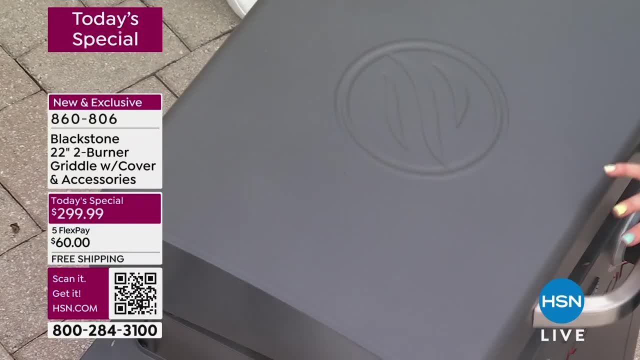 So I love as you're showing us, because you can cook so much at the same time. your meal prep doesn't have to take your entire Sunday afternoon and night, because you can do it so quickly for meals all throughout the week. Yes, Right here. 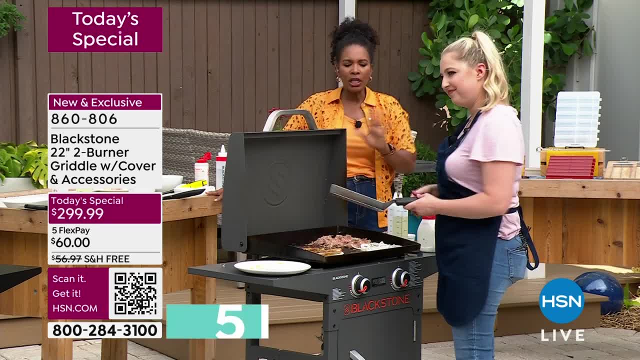 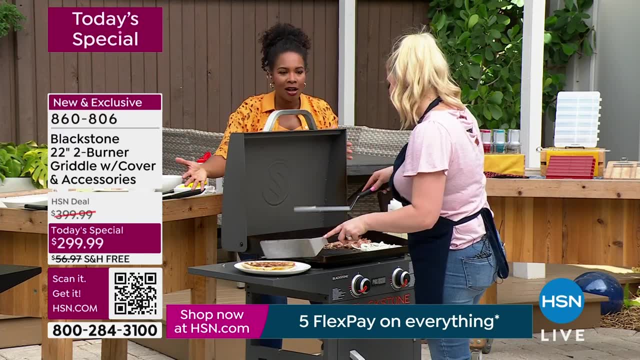 Yes, Um, we took a hundred dollars off the price. We've got free shipping. You're getting. you know, you provide your own food and you provide your own propane tank, but you get everything else. Yep, So you're using the two spatulas that Taylor's using. 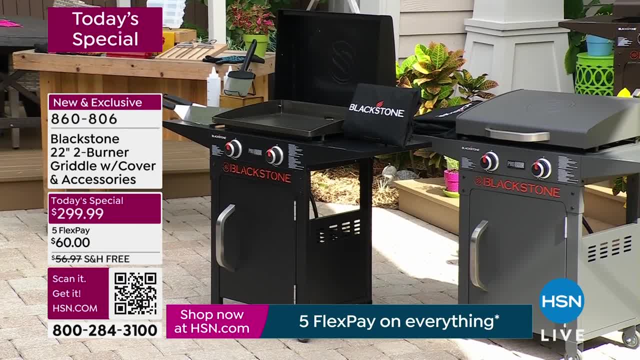 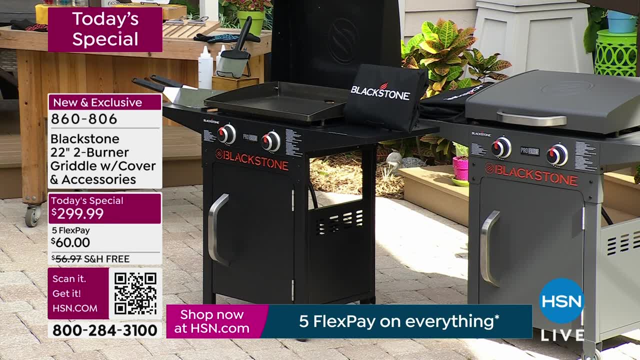 You're going to get the stainless steel scraper- and this is why you don't have to wash a dish- and it's with the help of that scraper you're going to get the two side flanks, the side tables on your griddle, AKA our besties, our best friends, because they are extra hands. 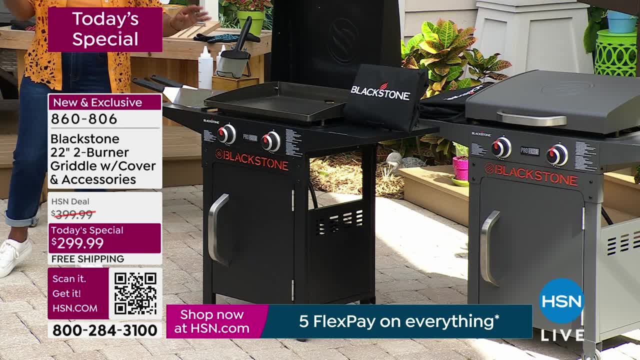 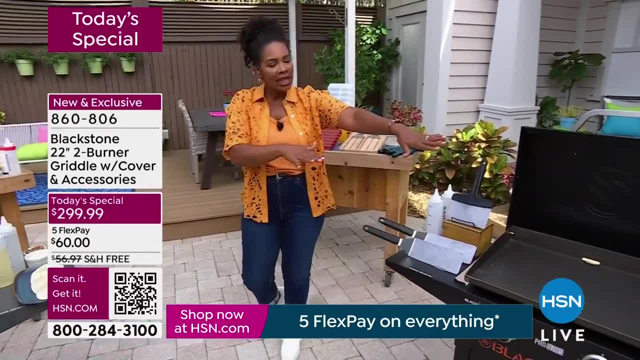 Yep, Um, you're going to get the two squeeze bottles You can have. Taylor has water in one oil and another, and you use them both when you're cooking and when you're prepping the grill. That's right, And you're going to get the cover to the grill as well. 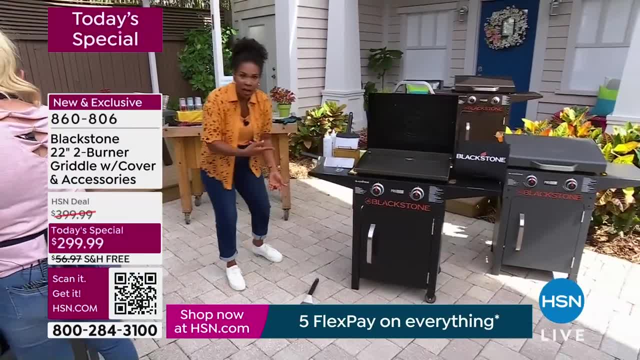 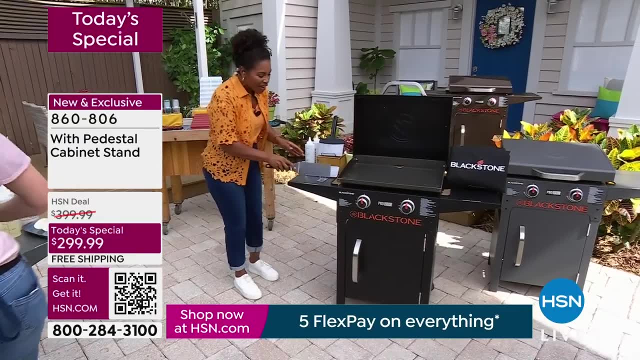 So when you're not using it, you keep it covered up. and then here we go again. I know they're. they're like: get me to the griddle girl. there's a ghost, there's a griddle ghost and you and you're going to get that cover so that when you're not using it, you 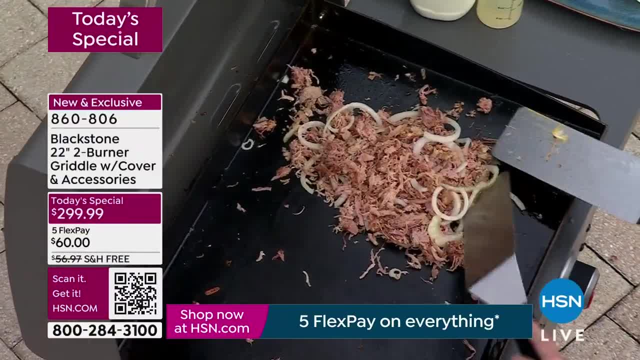 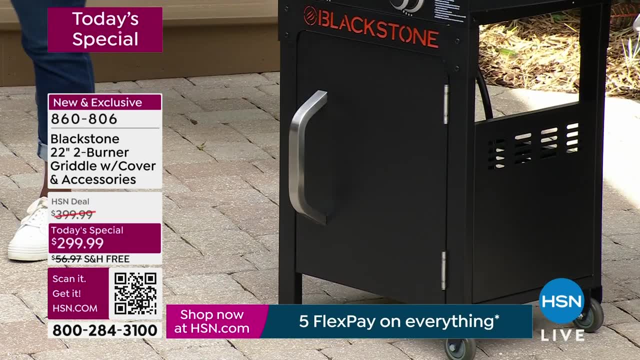 can keep it covered in nice. And then, don't forget, you've got that door up front and that's what's going to house your propane tank. Okay, Okay, I'm just going to hold this one. No, this is what needs to happen. 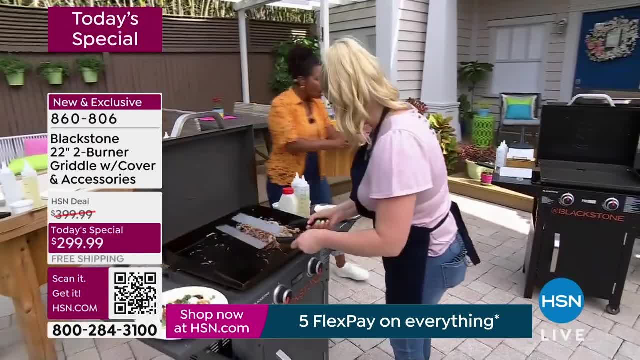 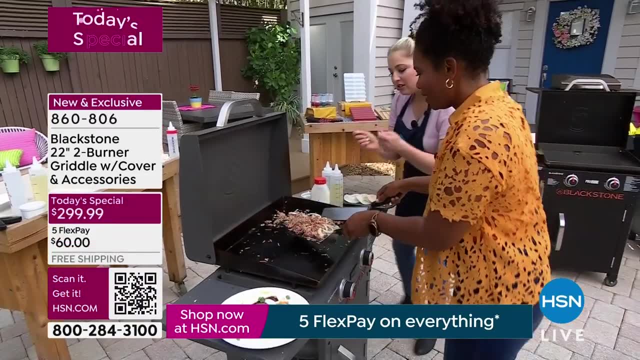 I want you to come over here, Okay, And I want you to hold these, Oh, really Okay, Because I want you to see that any, this is easy lightweight. Anybody can do it, Okay, So grab those and just just toss it around. 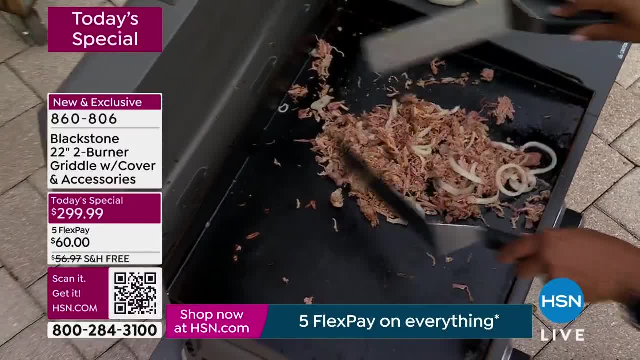 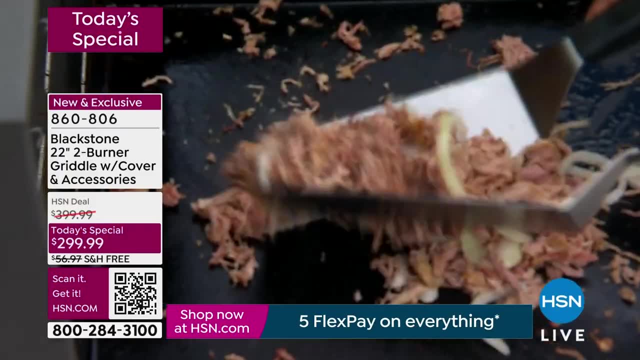 I feel so special. Don't be scared, girl, Just get it up and get it going, Can? I'm telling you, Yeah, just do whatever you want. And I'm going to tell you my first time ever, first time ever on the Black Steel Grill, right. 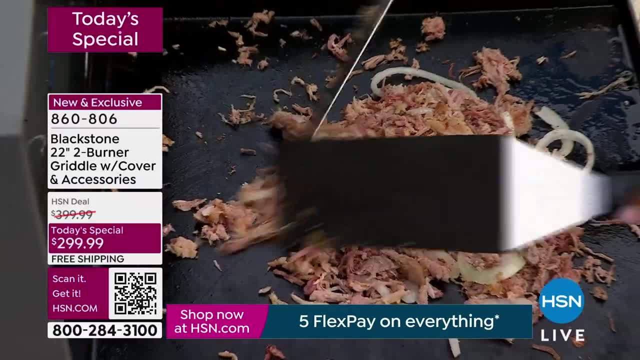 this second And look, she's not a professional. Am I doing it? You're doing it? Do I look like? see You look professional? Okay, This is going to be the example of if I can do it, anybody can do it. 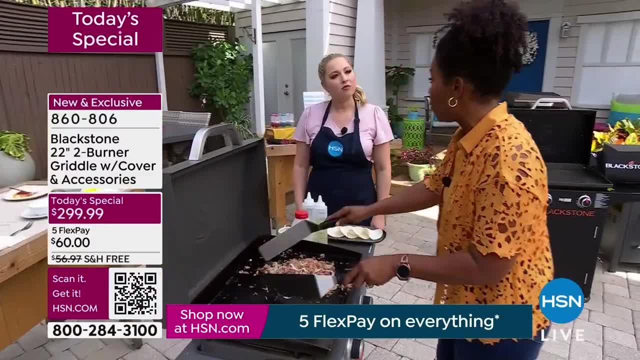 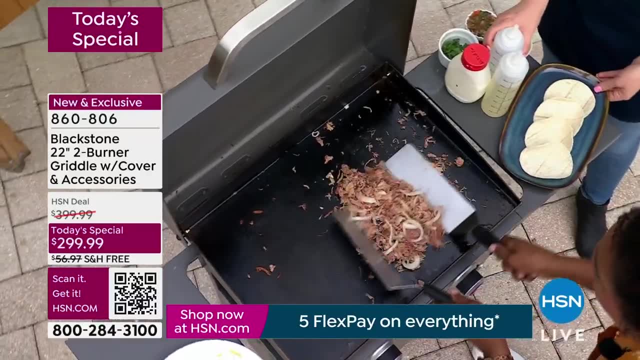 Because, to be honest, Absolutely, I didn't learn how to really cook until I was a grown adult and it and I was slow to the party, you know, and I just did kind of one thing at a time, Yep, So to be able to. 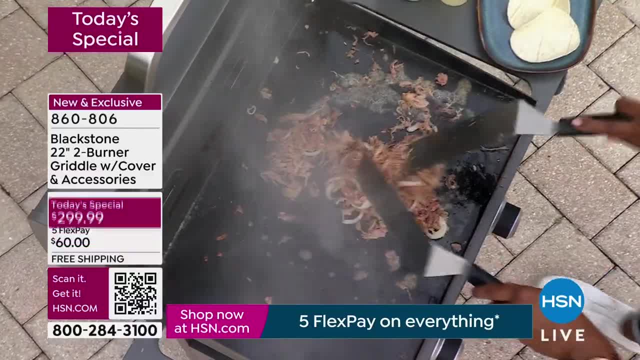 I'm going to add some water for you. Yeah, let's do it. Let's get some steam in there. There you go. Now you really look like a pro here. See, in a minute I'm going to be making the onion volcano. 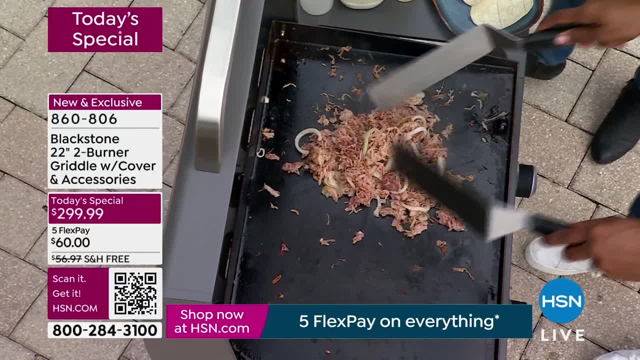 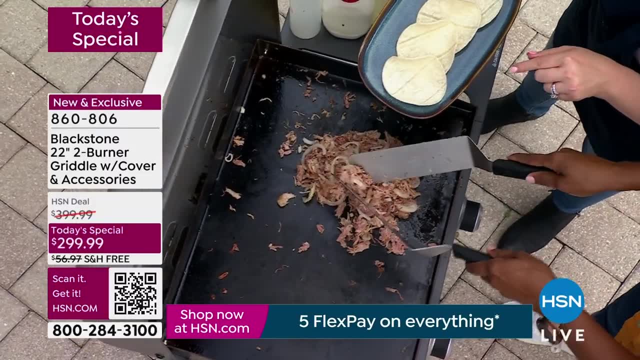 Yeah, I have full confidence in you. Okay, So we're going to make some tacos together, Don't be scared, It's okay. I want you to add a little bit of meat, Just a little bit, Okay, Yep, A little bit like this: 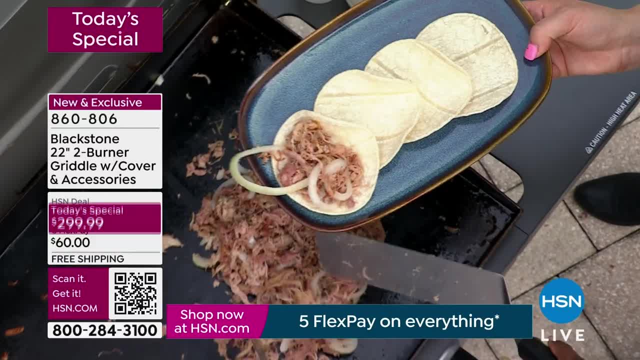 And put it on each. There you go. Okay, Look at that. Now do it, I did it. I'm going to make her do my job for me. Oh my God, Wait, let me get a little bit more here. 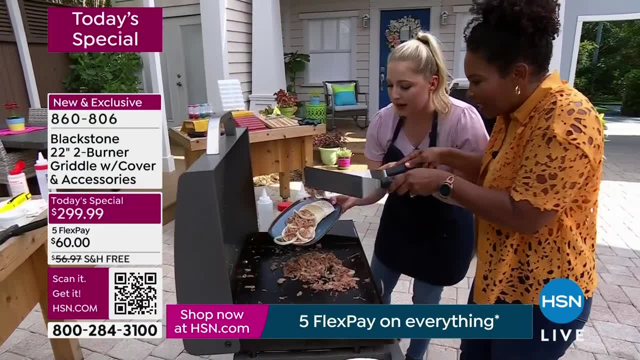 That's perfect Right on top there. Oh, that might be a little bit too much. Hey, it's okay, My husband would prefer that bite. anyway, We'll do a little bit right there, Yep, And a little bit over here. 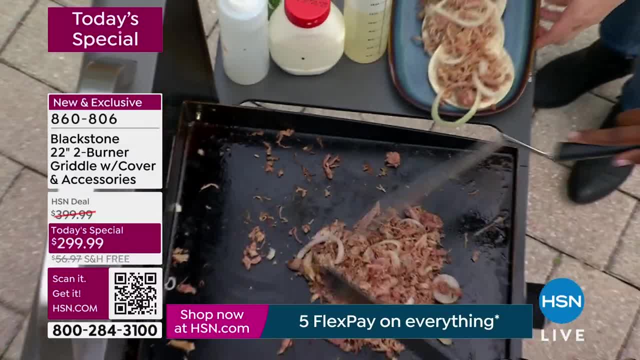 A little bit right here. That's why I said this is, this is so easy, Oh my gosh. Okay. So now we're going to add the garnishes here. I'll do this so your pretty fingers don't get messed up. 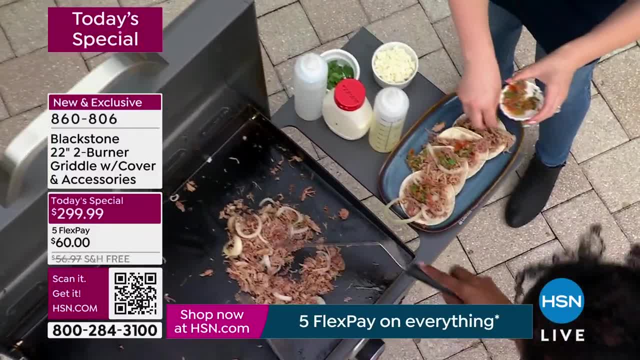 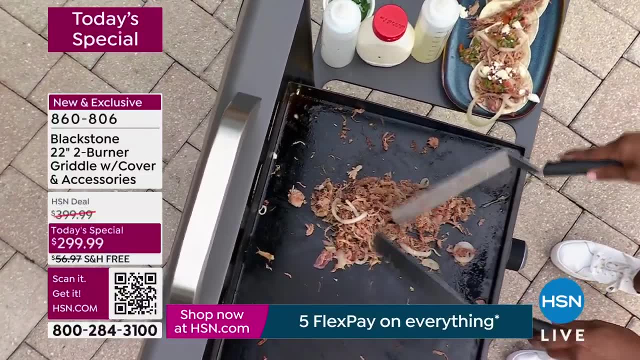 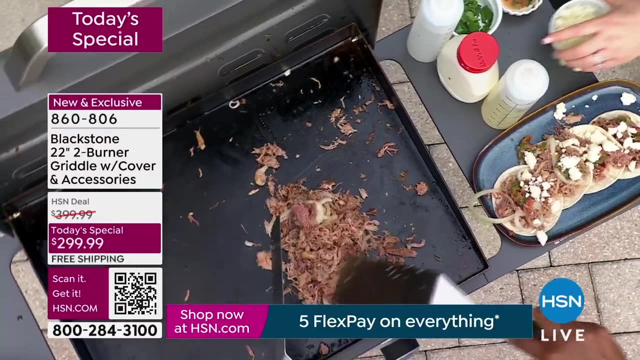 I'm going to add a little bit of my toppings. This is something quick, a weeknight meal, Great recipe that I have on my cooking show as well. You can add that cojita Mexican cheese, mozzarella cheese. My husband is dairy free so I love that I can just use his dairy free cheese. 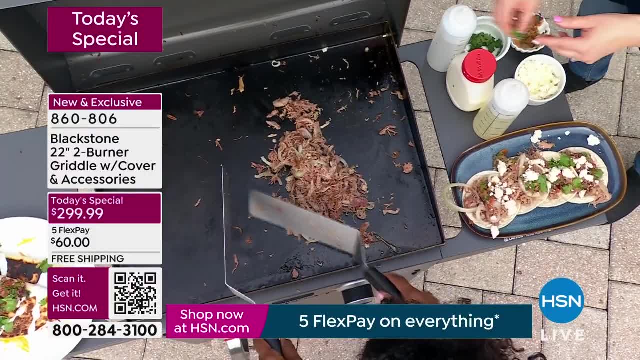 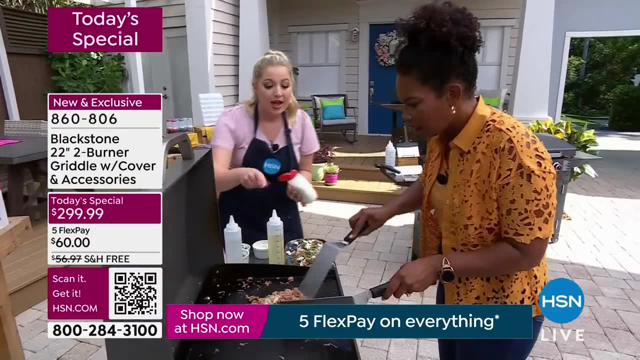 Very nice. Where can we see your cooking show? It's actually it's on Blackstone's YouTube channel and it's called Easy Weeknight Meals with Taylor Mock. Oh, That's simple, That's it. I'm going to add a little bit of crema. 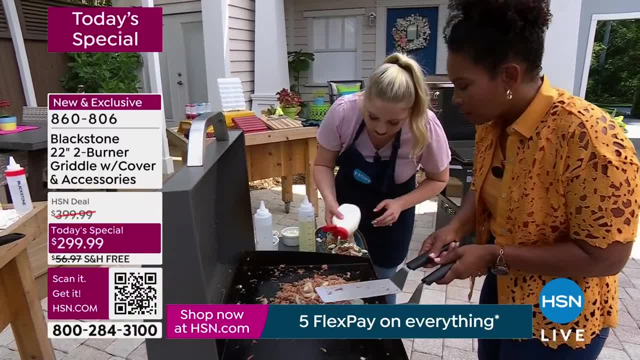 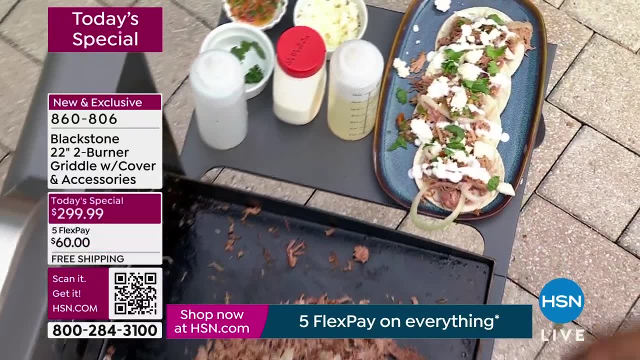 Now you see all that leftovers. Yes, Now with those leftovers, what would you do? Do you have any idea like how you would utilize that? I guess I could put them. It's pork and onions, so I could put them. we like pitas at home, so maybe I could put them in a pita. 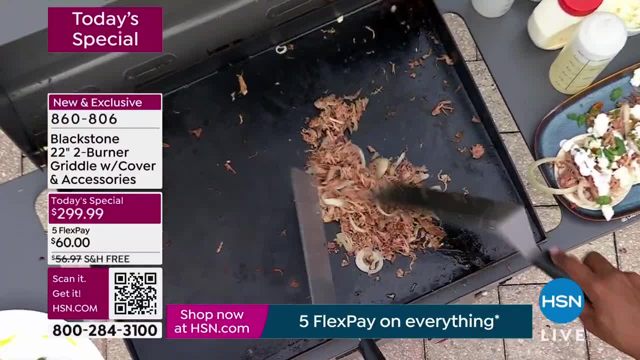 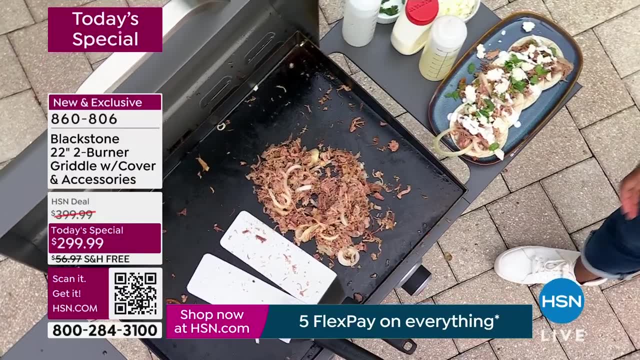 I love that. What about? what about a pulled pork sandwich? Yeah, What about a pulled pork quesadilla? Yeah, Because I made a cheese one. Look at that. So that's it. It's that simple girl. Oh my gosh. 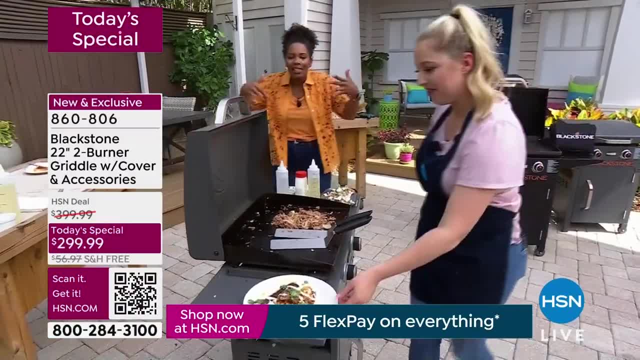 You feel like you can do it now? right, I do, I know, And you know what I feel, like I did something special. Yeah, Because sometimes, to be honest, and you probably agree, cooking can kind of get monotonous. 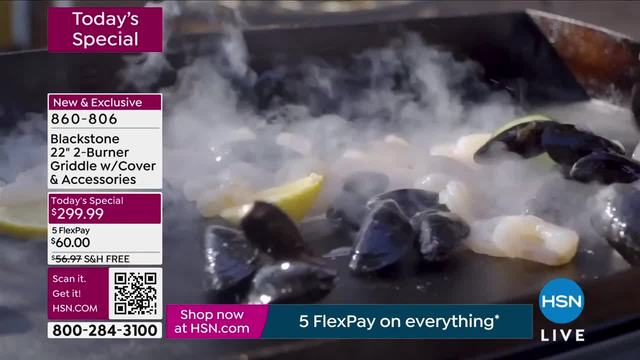 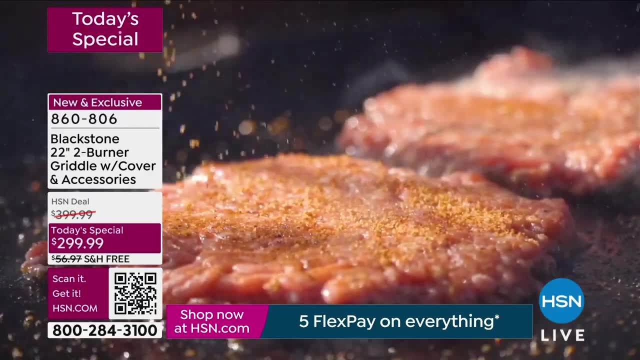 Oh, totally, Because you have to do three meals a day, every day, for the rest of your life, for the entire family, And I get that. And you're thinking: how do I do this in a way that tastes good, is easy, I can count. 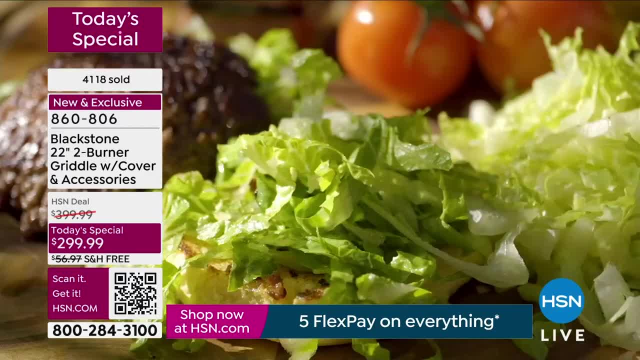 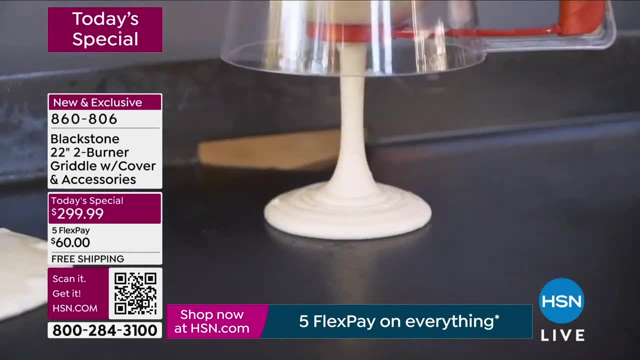 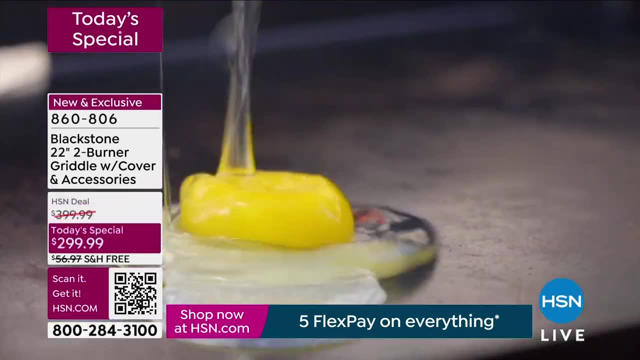 on the, on the outcome, I know it's going to be good. I'm not spending my entire day or afternoon trying to do all of the cooking, Yep, And I know, when I cook for my family at home, we're eating better. we're eating healthier. 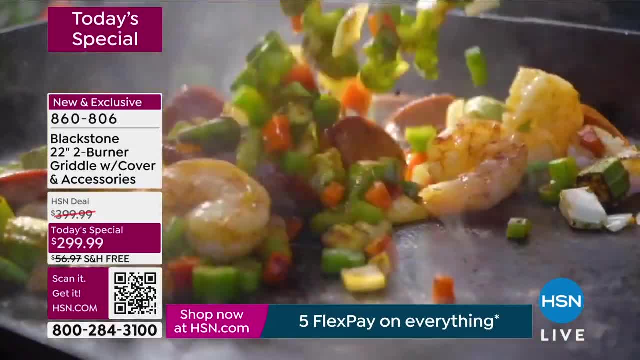 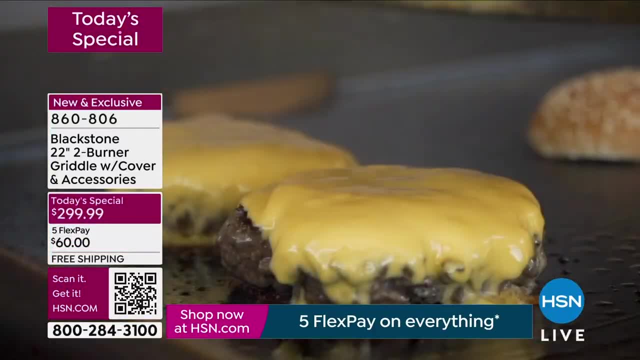 we're not spending as much money. it's just better all around when I can cook at home, Absolutely, And this I would look forward to doing. Yep, And that's the thing is, you want to bring your family into this. 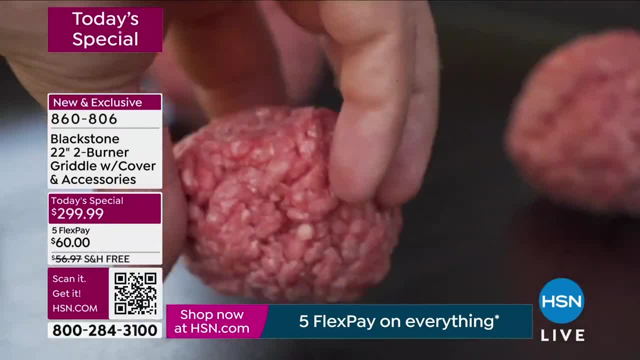 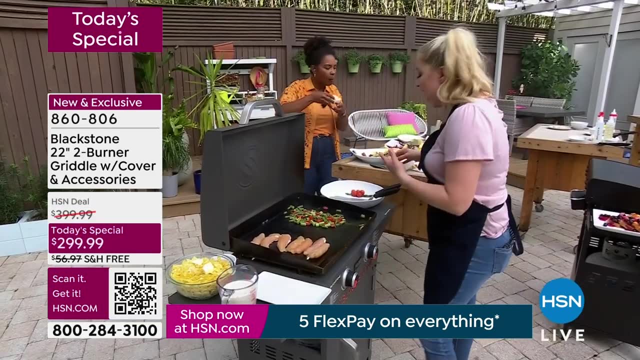 You know I've got my two-year-old baby girl who's when I'm cooking dinner? she's outside running around in the yard playing. my husband's sitting next to me. he's having his afternoon cocktail and I'm just telling him about my day. I'm listening to my baby play in the 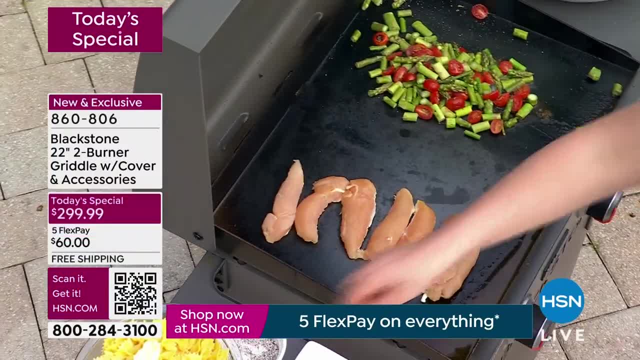 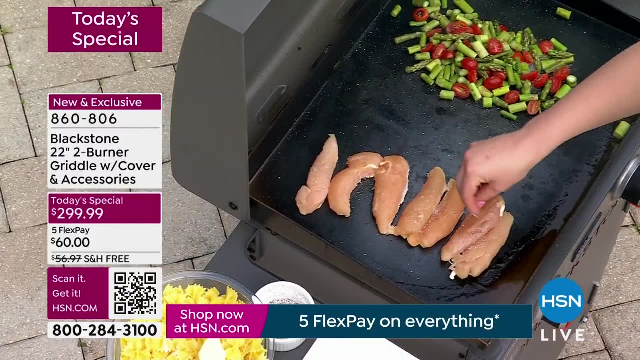 background and just know that we're having that quality family time. Oh, this is good. Usually, what happened before Blackstone came into my life is this is what would happen: I would be in the kitchen, my husband would be with my baby in the living room playing. 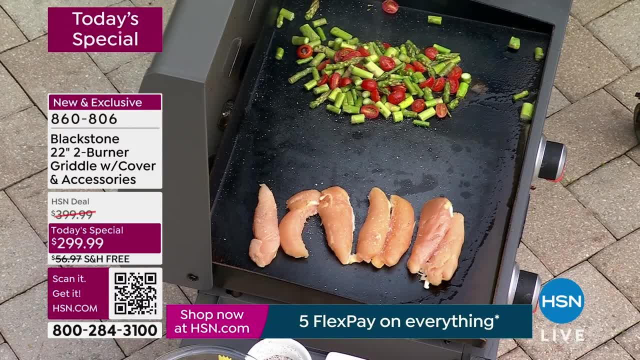 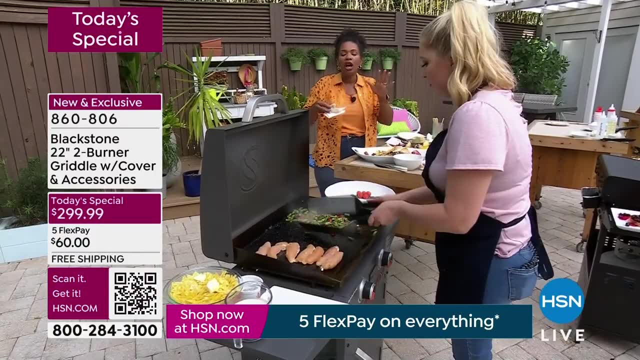 with her and I would be missing out on those moments, and I hated that. Now we're all together. Yeah, You know. Yeah, She's young now. Yeah, She's two, But she'll be learning how to cook. 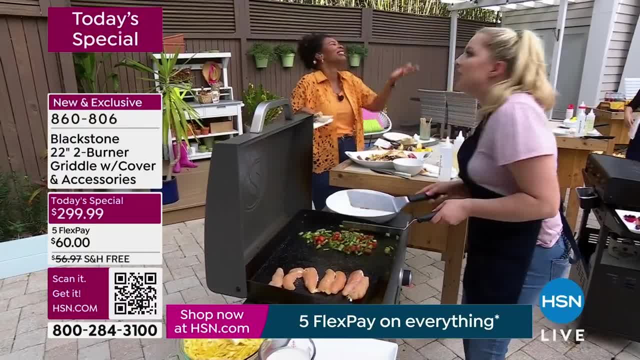 Oh, she will. Like I said, I didn't learn how to cook until I was an adult. She has her own Blackstone. Blackstone has a Blackstone toy out, Oh my gosh. And she is right next to me on her little Blackstone. 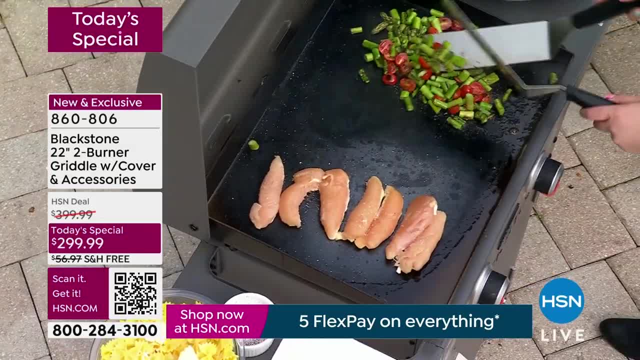 It is the cutest thing. Watch out, Watch out. You're going to have an apprentice in the kitchen very soon. I'm telling you, I'm going to lose my job. She's going to be the next Blackstone girl. She's going to be your sous-chef, you know, by the time she's five. 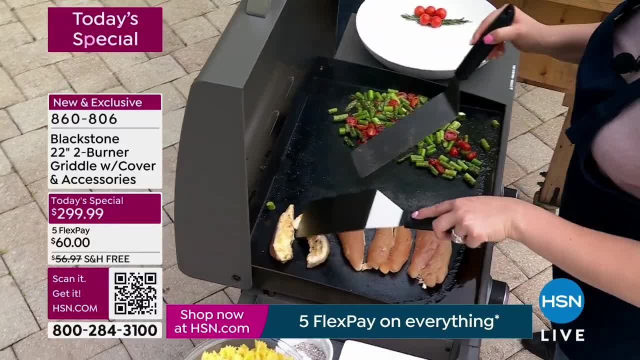 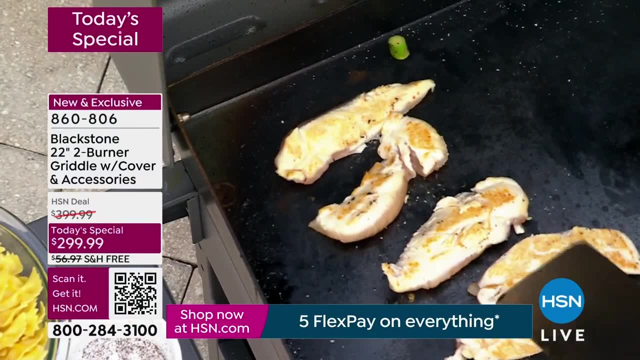 I love it Absolutely And I'm here for it. Listen to our customers over the many years. we've launched, in 2008, our Blackstone journey And we have 10-year-olds here that are cooking on the Blackstone. They're learning for the first time with their parents, with their dad. 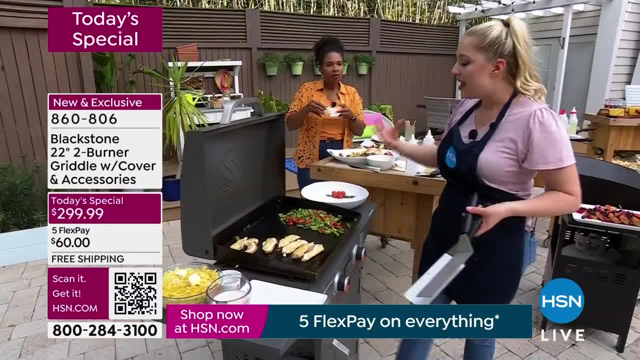 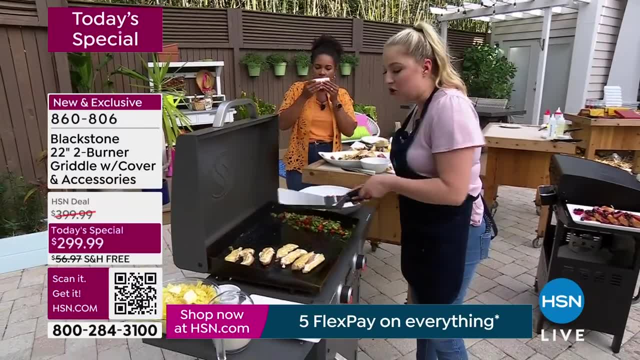 And it's just such a neat experience to watch your kids kind of get out there and learn something new and learn something they're not learning in school, right, And on top of that you're spending that special time with them. Yes, So, whatever it is, whether it is a dinner, a breakfast, 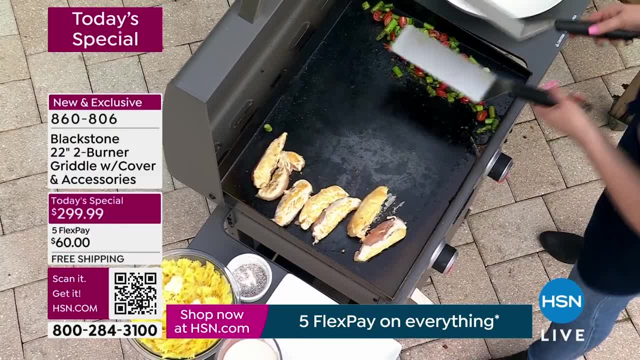 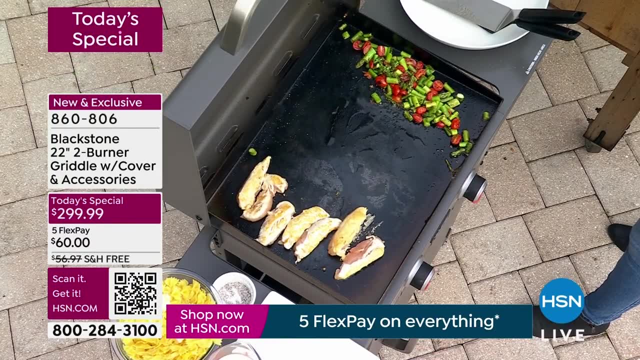 A breakfast, A dessert. I promise you can do it. You can make pasta. That's what I'm doing, by the way. Can you believe it? This is what I wanted to see too: the way you do pasta. You know, what's so interesting is we at my house on the big fire grill. my husband does. 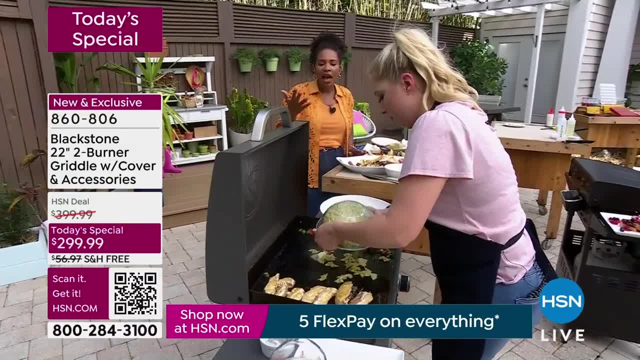 it. Yeah, Oh yeah. I don't do the open flame, But I have to ask him. you know, we want to have steaks, I want to have steaks today. He's like: okay, I can make steaks. 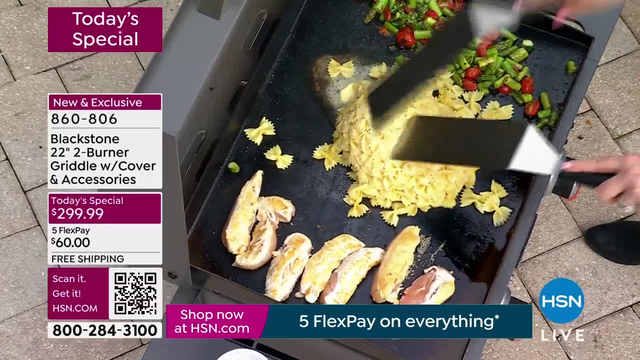 Yeah, You're inside doing the other stuff, I'm inside, But sometimes he doesn't feel like it. Yeah, Sometimes it gets too dark, Sometimes it gets too late, Uh-huh, And so we don't have steaks that day. 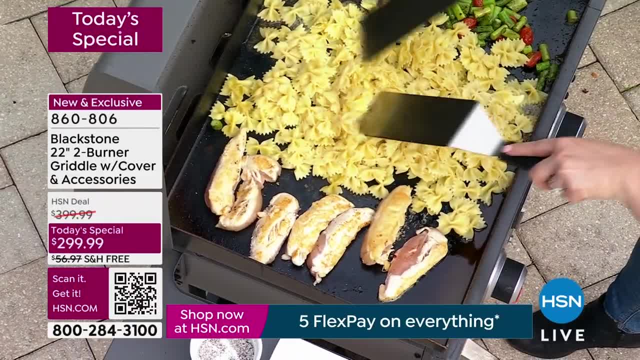 We have to have steaks next day, Yeah, Or the next day, Or whenever he feels like cooking them. Yep Right, Yep With this. if I want to make steak, I can make steak. Totally, I can do it on my own. 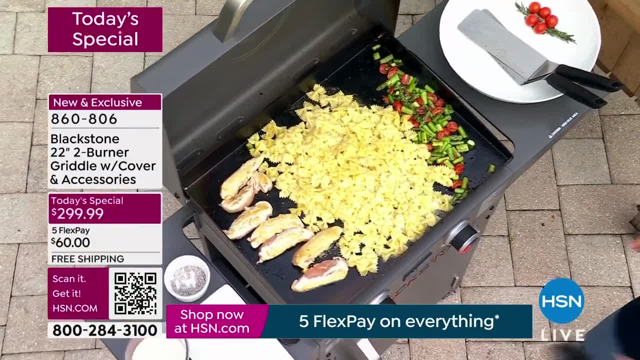 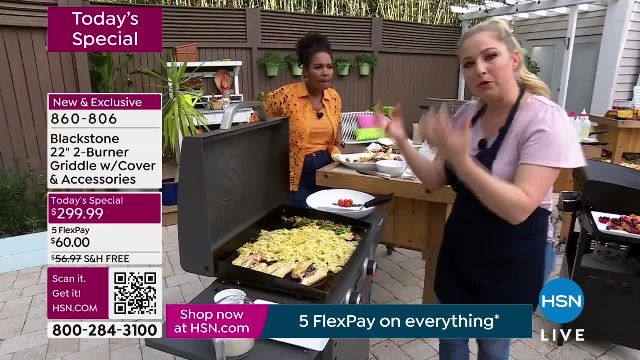 And you know it's going to be quicker than an open flame grill, Is it really? Yep, And then you can treat it. Have you ever cooked a steak on a Blackstone or on a cast iron skillet? Mm-hmm, You use butter. 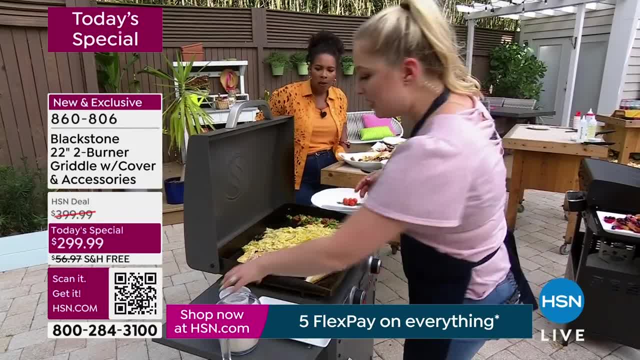 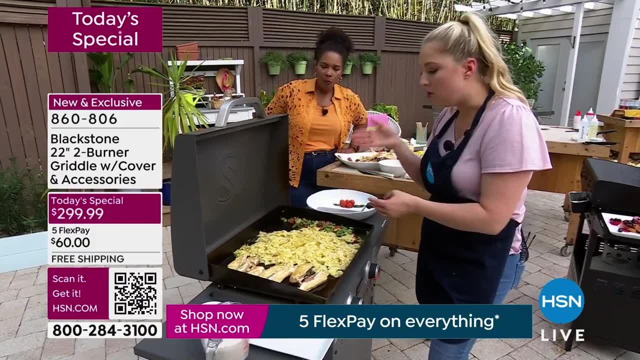 You use your rosemary, You're kind of basting as you go. Yeah, There's nothing like a steak on a cast iron skillet. It's the same thing. This is the same thing. This is cold rolled steel. This is going to last you forever and ever. 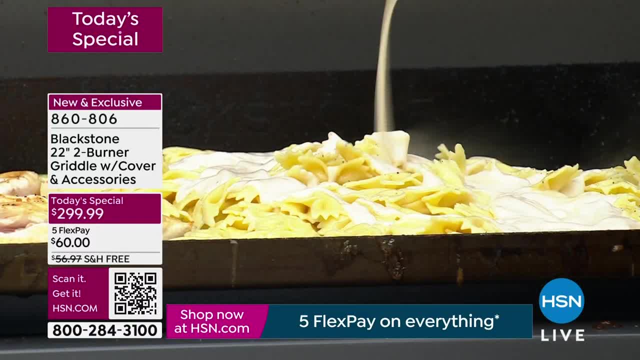 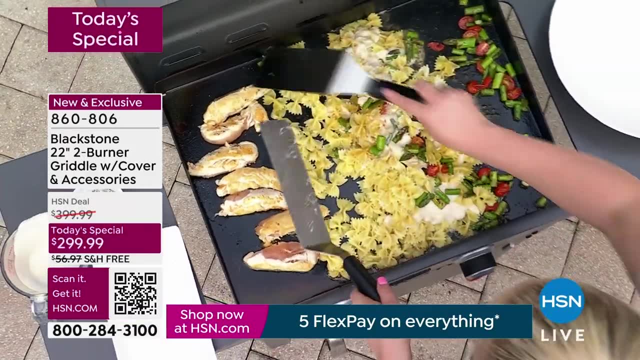 If you want a number, it's got a one-year warranty on it, But trust me, it's going to go well, well beyond that. This will last you a lifetime. This is the way to go It is. You know, this is something that I love to make when I have girlfriends over for wine. 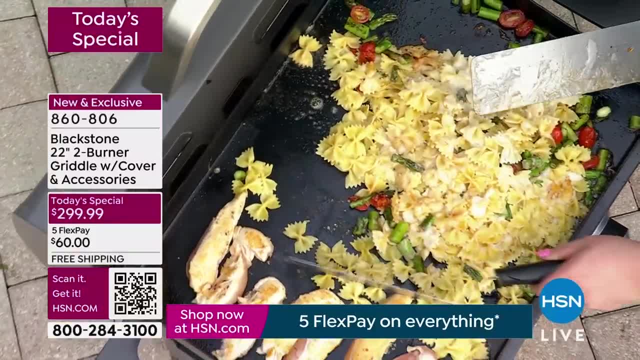 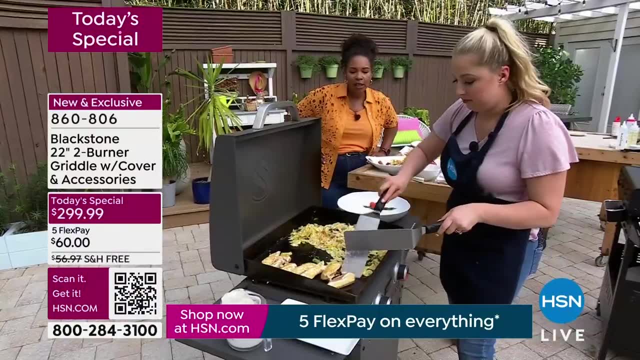 night Mm. I also love to do this for Bible study classes too. Yes, This makes for just a really easy meal that feeds a lot of people. I love it. Hey, there was wine in the Bible. There was wine in the Bible. 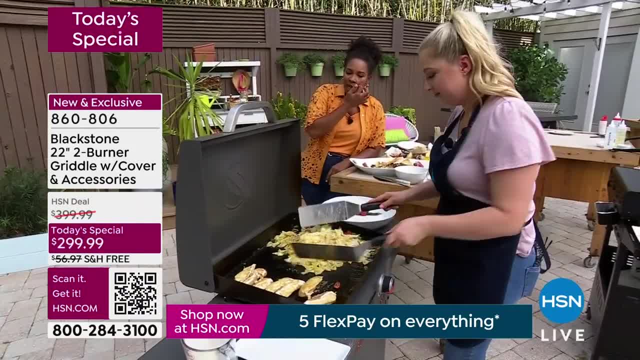 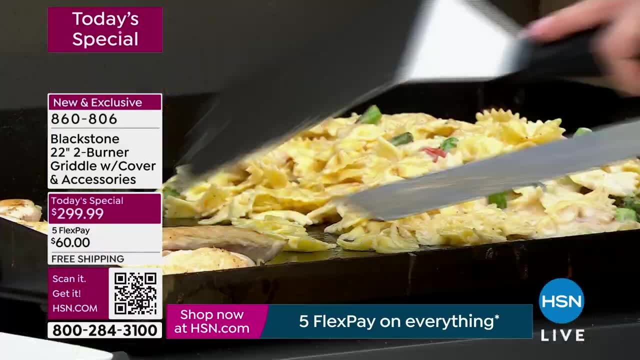 Amen, I love it. There sure was. Let me share with you. I know that our clock is we're getting, you know, kind of getting late in the show, And I know that we've already lost one of the colors, but we still have either this: 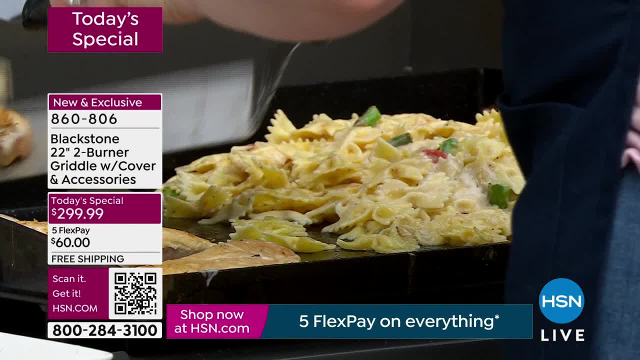 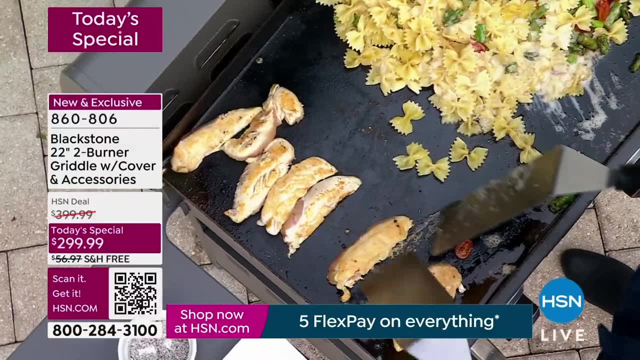 gunmetal color or in black. This is your time to go ahead and do it Now. we already took $100 off of our regular HSN price And you've got free shipping, which is great, Mm-hmm. And you're saying you know what? oh, I wonder if I could get it at a better price, an even. 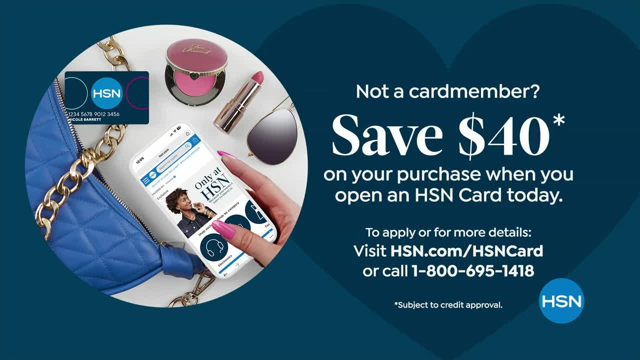 better price? Sure, Yes, you can, And that's if you're getting an HSN card. And so when you do, when you apply and you're approved, we give you $40 right off the bat. We put it in your account. 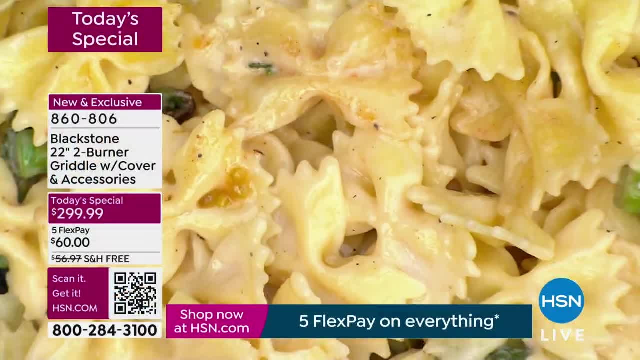 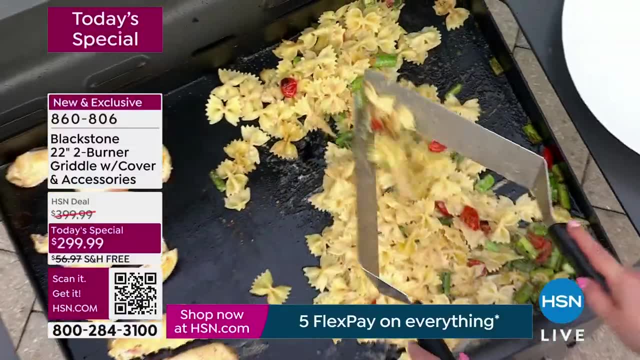 You can use it towards any of your purchases at HSN, And so, if it was, is it if it's towards this today's special? yours, not anybody else's, but your price would then be $259.99.. Wow. 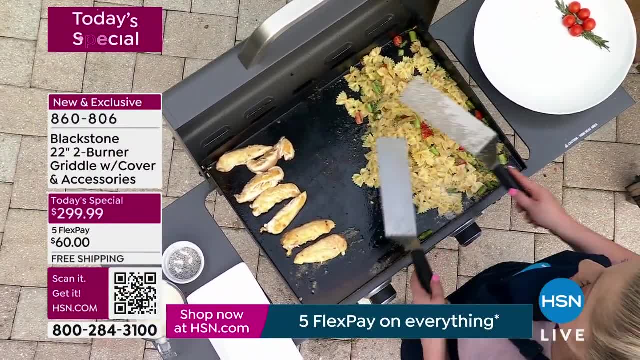 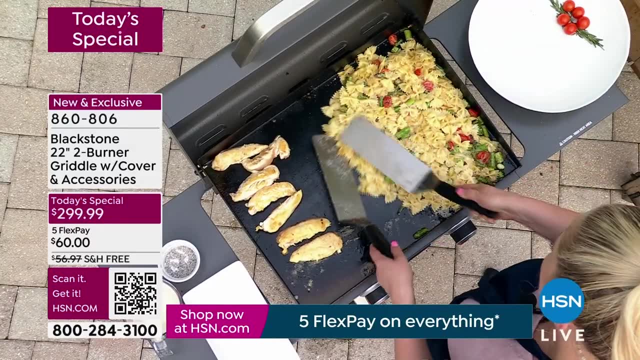 That's crazy. Yes, Which is unbelievable. Do your research. Yes, Because you are never going to find this deal, No, Anywhere else. No, I promise you, This is the time to go ahead and get it. Shop on HSNcom. 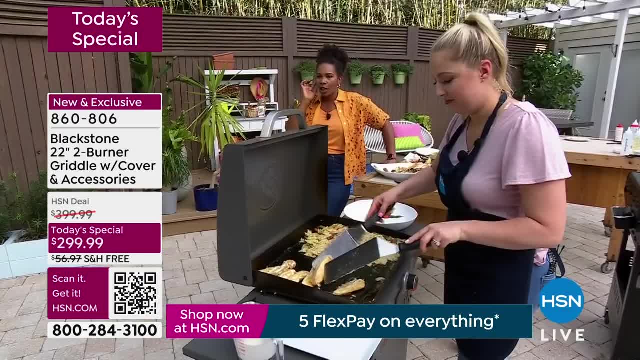 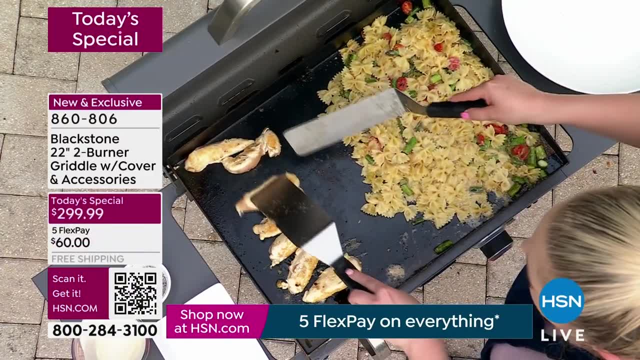 Use the HSN app, Use the QR code. Even on HSNcom there's lots of other kind of inside information about, like, if you want to watch how you, how you clean it again, how you season it again, you can easily do. 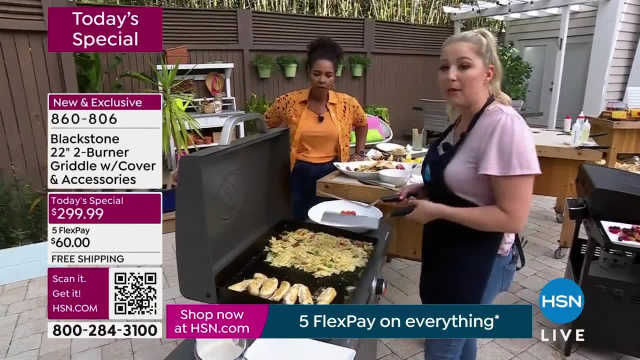 that. Oh yeah, there's a whole video on that. Yes, There is a whole video. Let's talk about that real quick, Okay, So you're going to take a few minutes for you to actually build it. set it up once you. 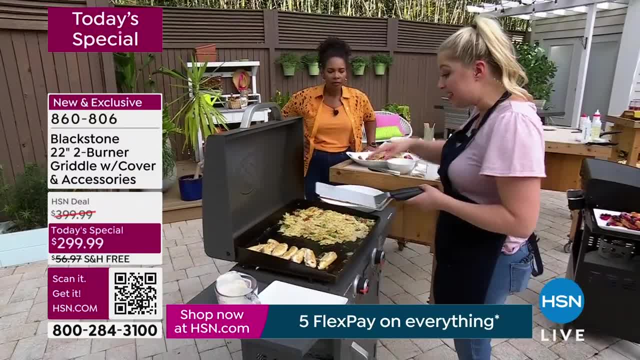 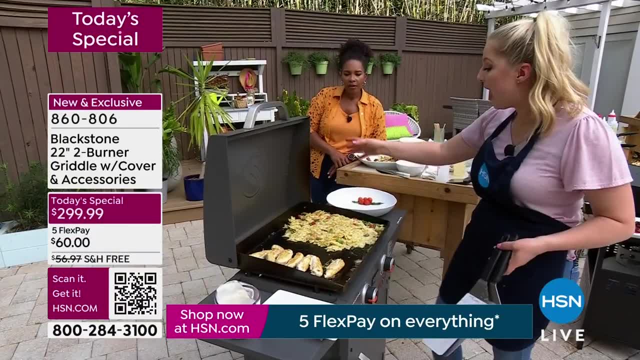 get it home. Okay. Once you set it up, the next thing you want to do is you want to season it right, like you would a cast iron skillet. It's so easy. All you're going to do, Tamara, is you're going to add your oil on top, whether it's 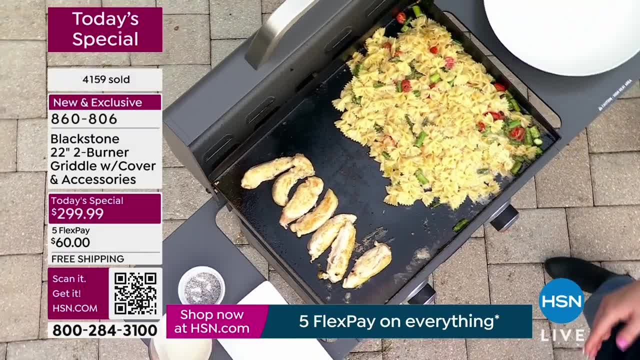 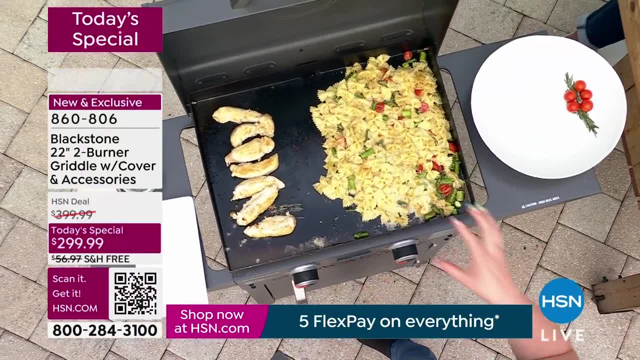 vegetable oil, olive oil, avocado oil- People use all sorts of things, Crisco, I can go on and on. As long as you completely oil it, you're going to turn it on high and you're going to burn it down. 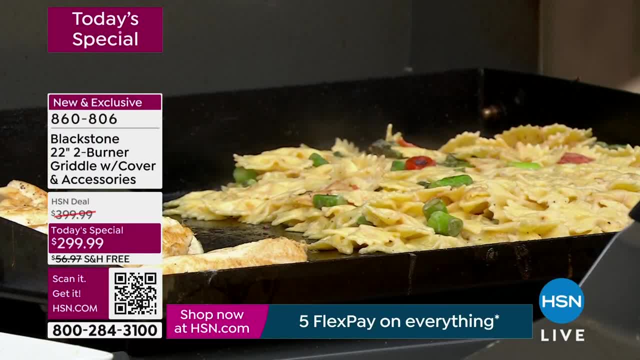 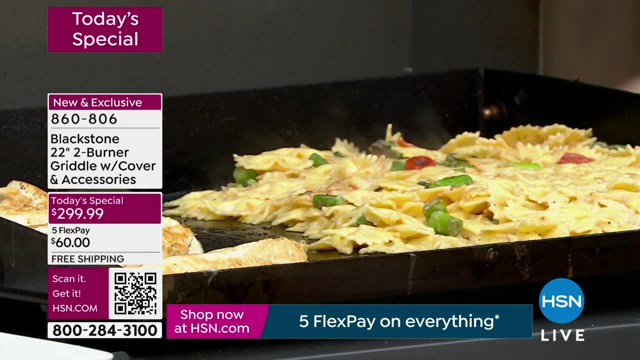 You're going to start to see the color change of the cold-rolled steaming. Okay, All right. So instead of that bronze color, when you get it, it's going to start moving outwards and turning black, just like a cast iron skillet. 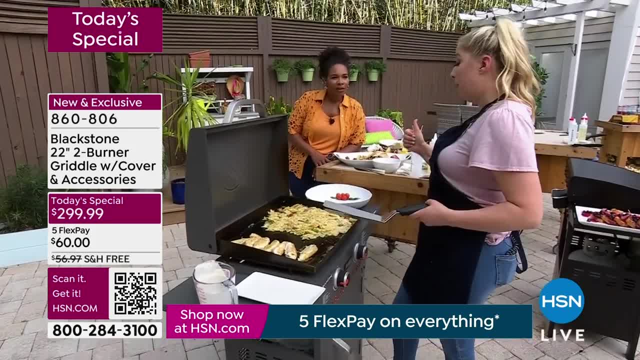 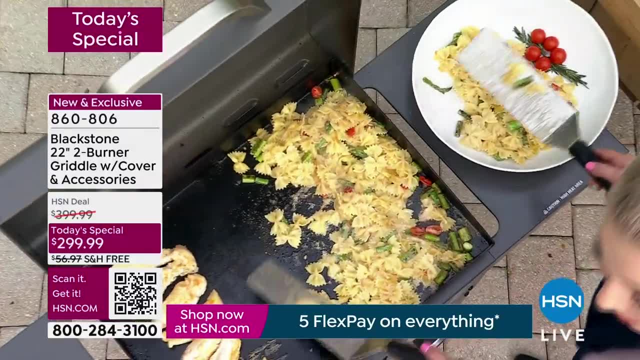 Yeah, So once it turns black, you're ready to go. Oh, And that's it Now, the first cook. I'm going to tell you exactly what your first cook is going to be. Okay, It is going to be a bag of onions. 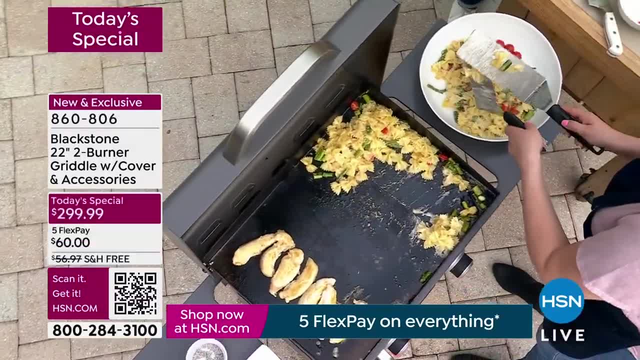 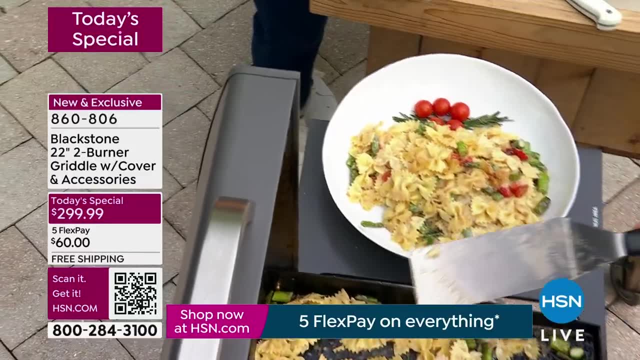 Oh, Okay, Don't use any kind of like bacon fat. I've heard that before. Yes, Your first cook, trust me, A bag of onions. Cook a bag of onions. Okay, Just like grandmother did. She's always said: just cook some onions in that and it'll render down the best flavor. 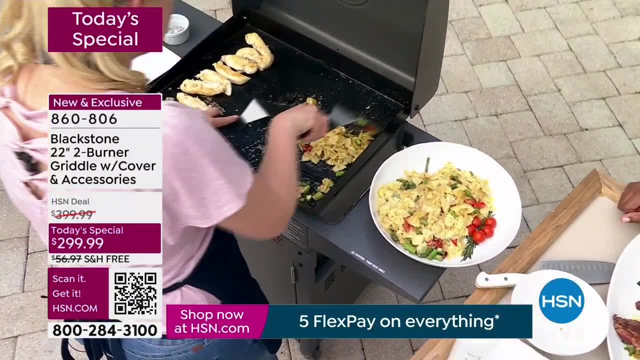 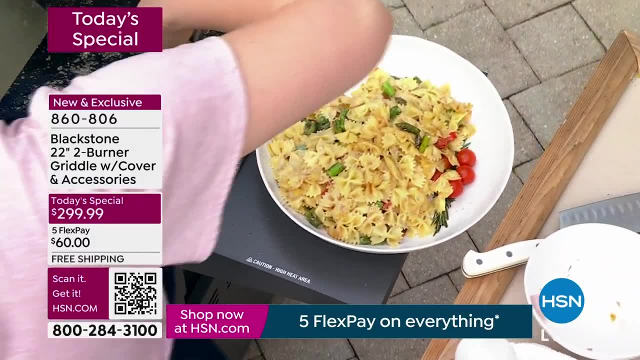 Remember. this is memory, This is going to lock in the memory of what you're cooking over the many, many years. That's why, As long as you take care of it, Yeah, And when you think about, like you mentioned, like grandma's cast iron pan, 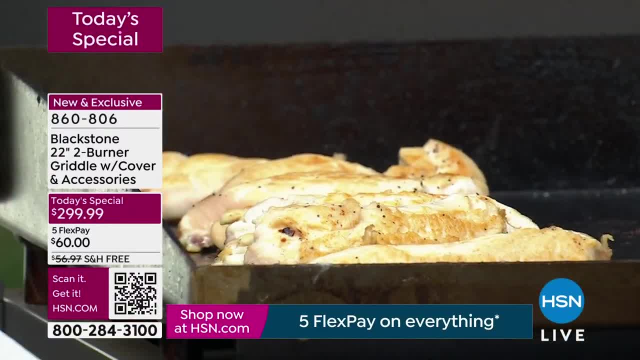 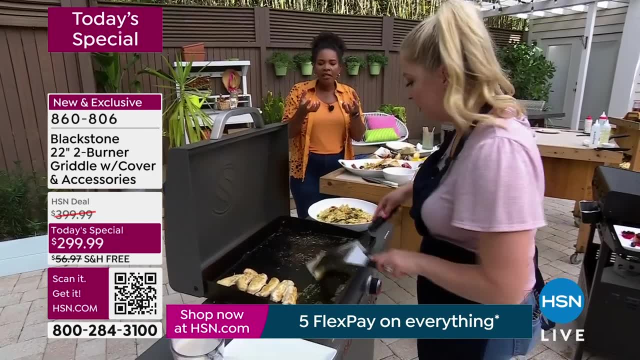 Uh-huh. People in the family probably have had arguments over she promised it to me. No, she promised it to me Uh-huh, Because there's something about Yep, That seasoning memory, Something about it That just makes the food taste better. 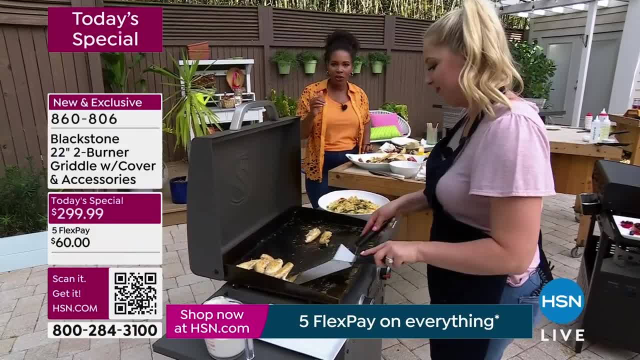 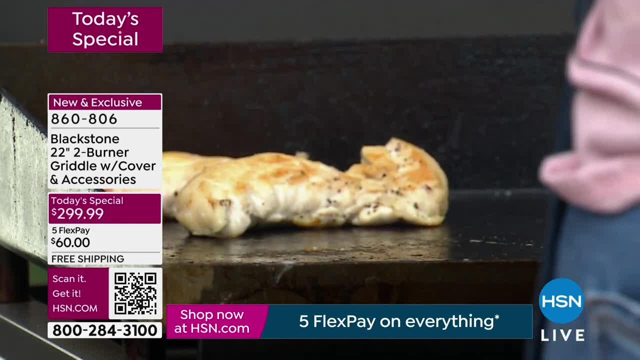 And that's why we're excited that you're getting this Blackstone Today special home And so that you can start to create those food memories. Food memories are some of the strongest in families. Uh-huh, You can remember somebody's you know had the best recipe. 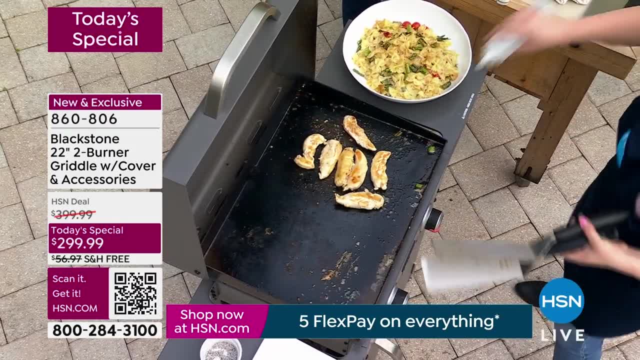 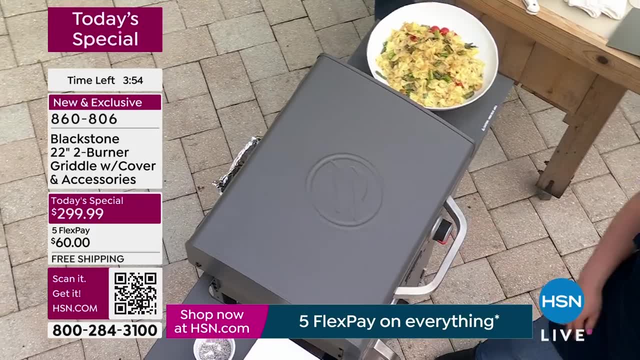 You fill in the blank: Totally The best burgers, Yep, The best you know. whatever it was, Whatever it was, You remember it, And then you kind of be part of that story And then you close the lid And I'm just going to steam this chicken off real quick. 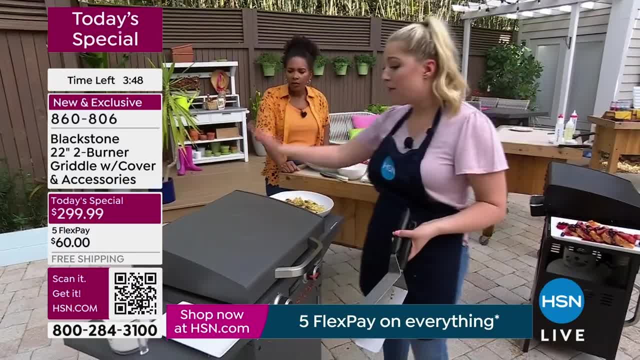 I want it to get nice and crispy on the outside, fully cooked on the inside. Remember, you can use this as basically an oven. Uh-huh, You can make cookies on here. Yes, ma'am, you can. Wow, You can make cookies. 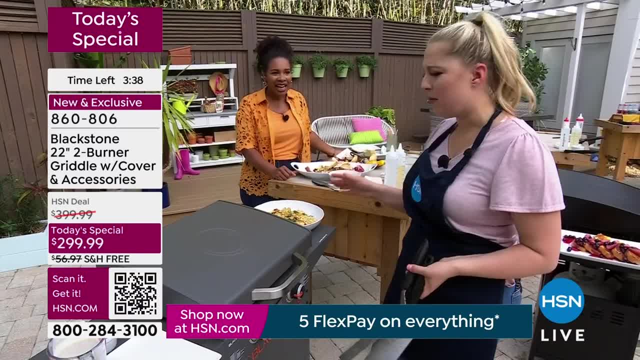 I've done brownies on here. Wow, I've done some crazy things on here that people would be like: wait a second, what You can't do, this stuff on a grill. This is going to do everything your grill can do. 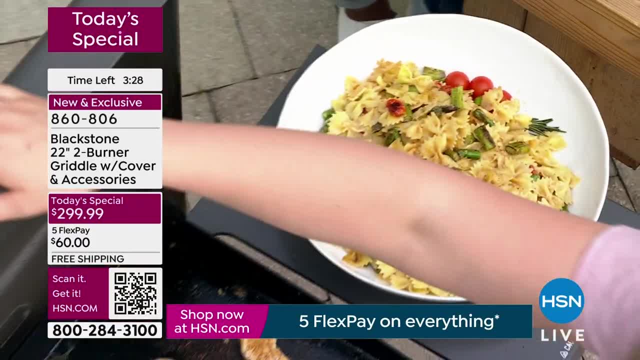 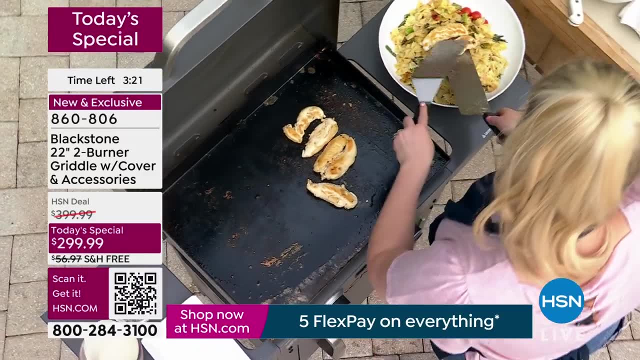 Yes, But it can't do. Yes, This is the most important. Oh, I'm glad that you said that. Yeah, Because some people are saying, well, I have a grill, Uh-huh, But you can't put pasta on your grill. 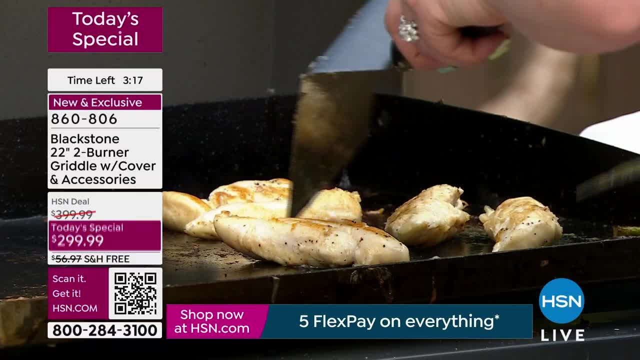 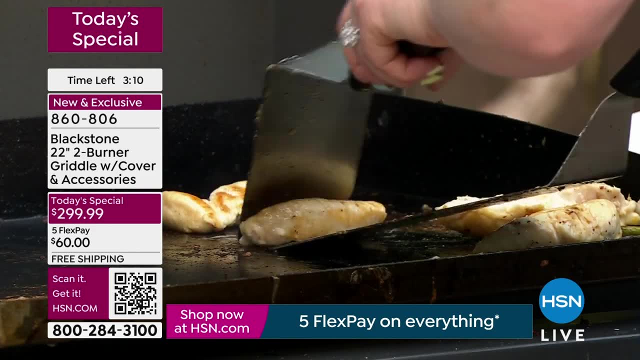 I don't care what kind of pasta it is, Absolutely not. You can't put rice on your grill. No, You can't put blueberries on your grill. You did all of this on your Blackstone. That's right In a matter of minutes. 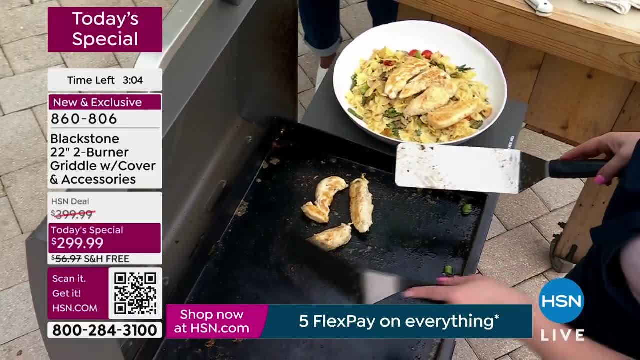 That's the thing you know. It's a matter of minutes. This is a popular dish I like to make. This is the dinner. This is the chicken. I leave this on the side. This is the side for my little baby girl. 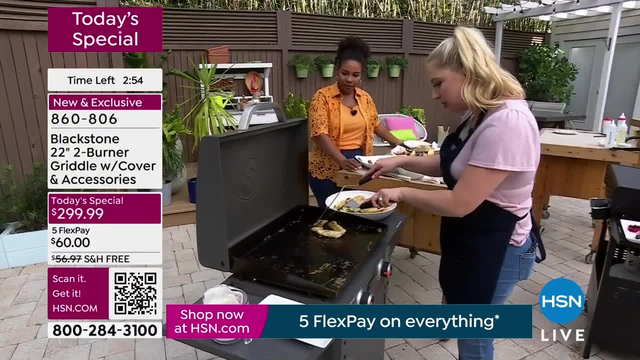 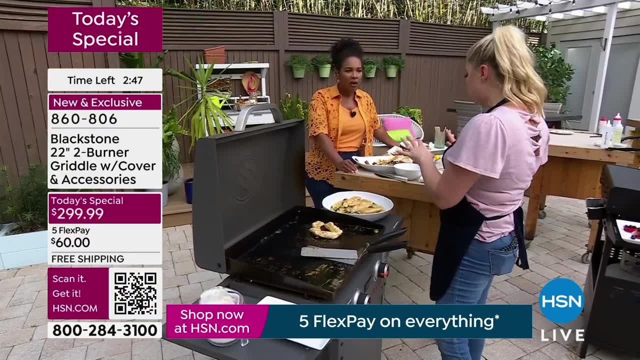 I get it really, really nice and all the way done. Crispy, crispy, crispy, That's how she likes it. I add a little bit of sauce to it. I'll add a little bit of leftover Alfredo sauce, And she loves this. 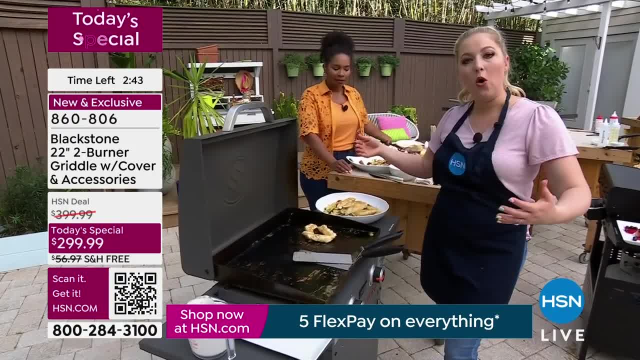 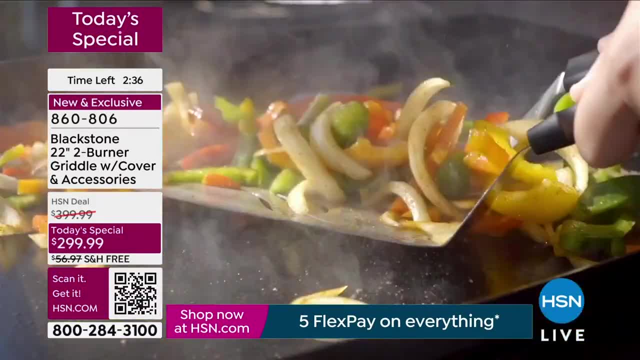 Wow, So I want you to think that you are able to control who's eating what time. Uh-huh, How much you're putting out there. Yes, Easy cleanup What's in the food? How much you're spending on the food. 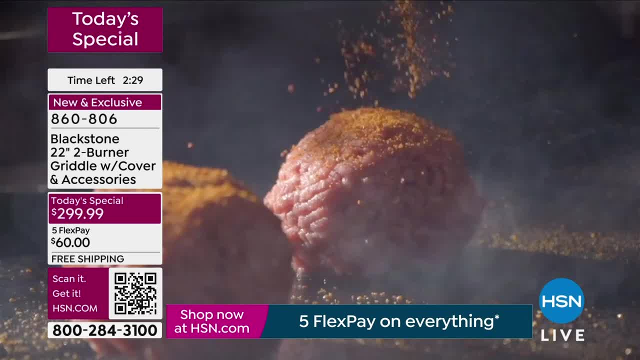 That's right, And you're doing that with every meal. With every meal, Not just for dinner, Not just for steaks and burgers and dogs. Right, This is for every meal. This is when you're cooking for one or two people. 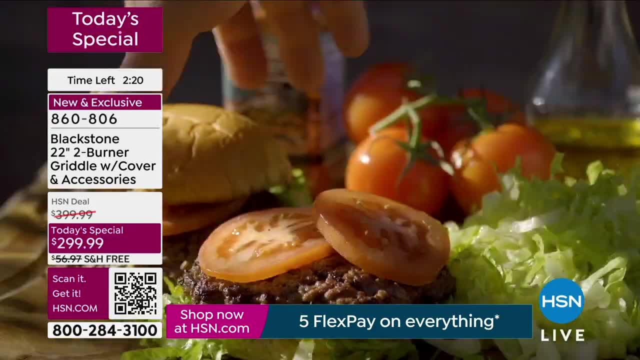 This is when you're cooking for five or six people. Yes, This is when you just want a different flavor to the same kinds of food that you eat every week. Uh-huh, And maybe you're a little bit bored with chicken, You know. 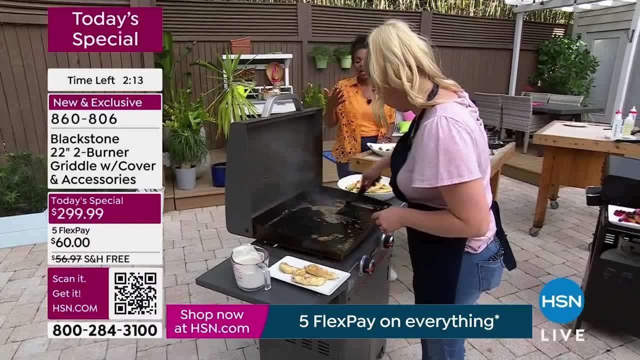 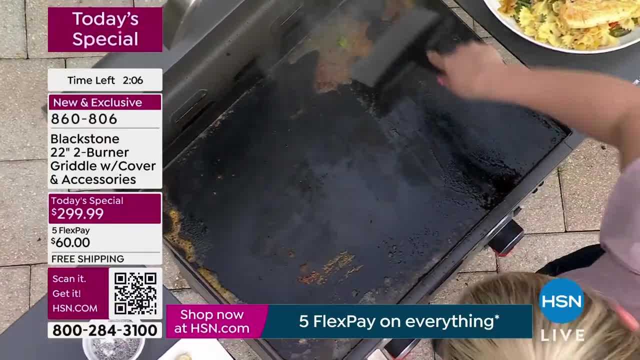 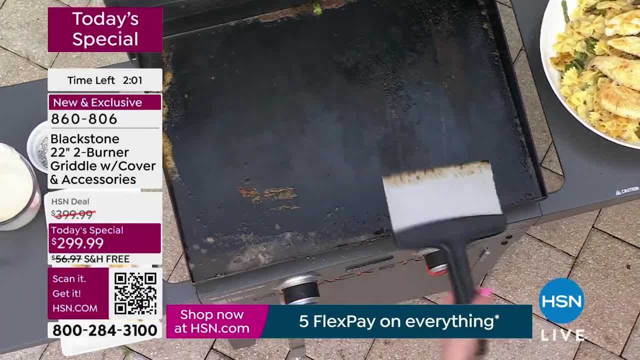 Hey, Taco Tuesday, I know, Get over to my house Speaking of tacos. Let's have some margaritas and some tacos. Speaking of tacos, the pulled pork that you made, the tacos you made, Yes, Divine, You tried it. 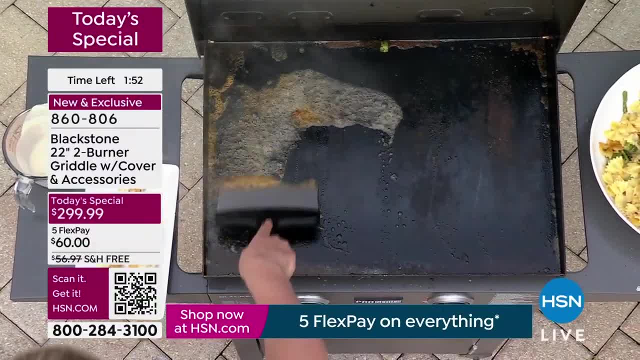 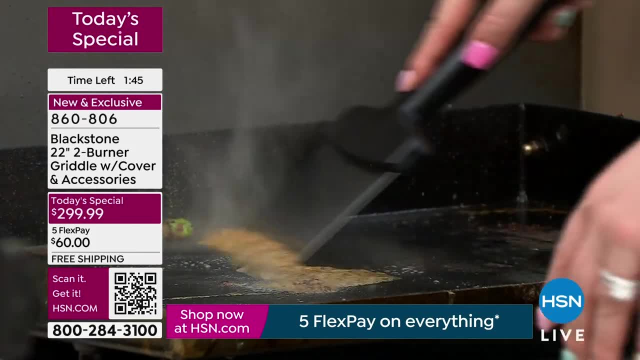 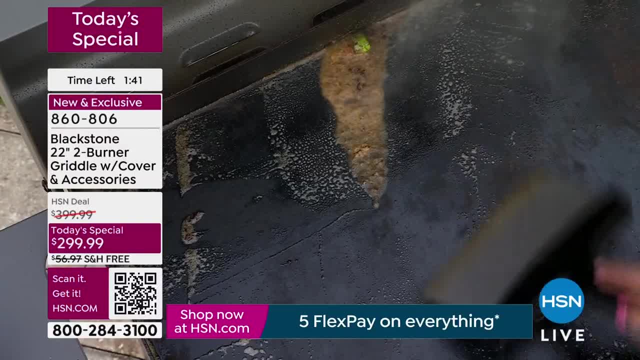 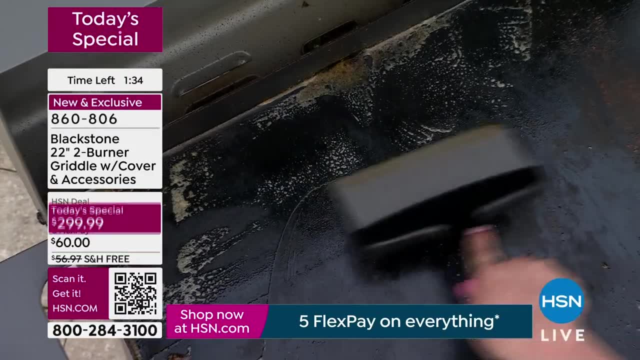 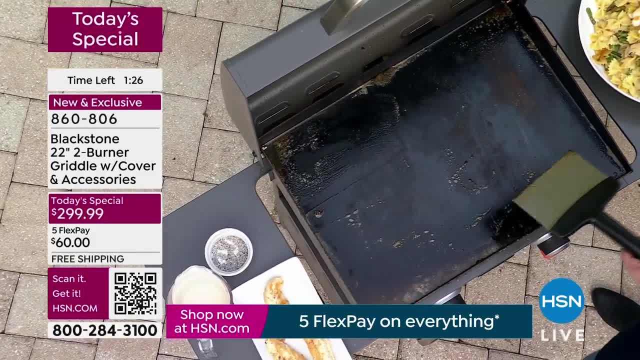 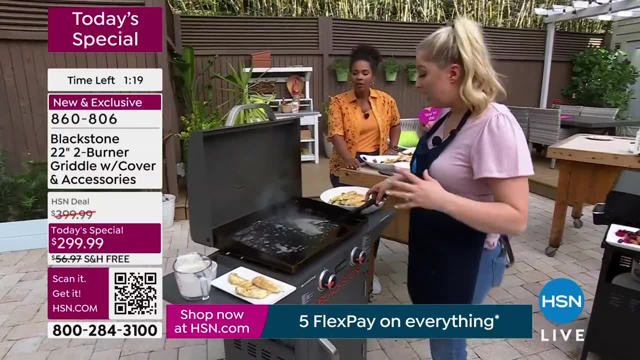 like I need more recipes. we have over one billion streams- What One billion streams- of all of our YouTube channels, including mine, that houses all those fun recipes. Whether it is and it's kind of it's, everybody has their own you know, their own, you know. 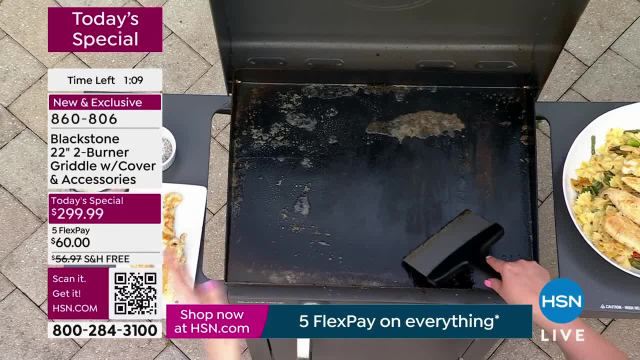 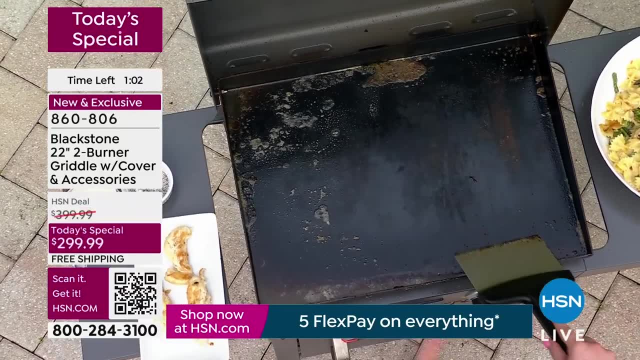 their own recipe. Right, Everybody has their own. There's a griddler, I'm a griddler. Yeah, I'm considered a griddler, But I'm the- I'm the busy mom, the weeknight meal recipe girl. 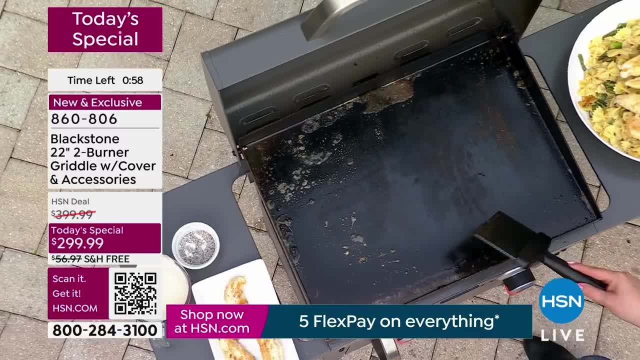 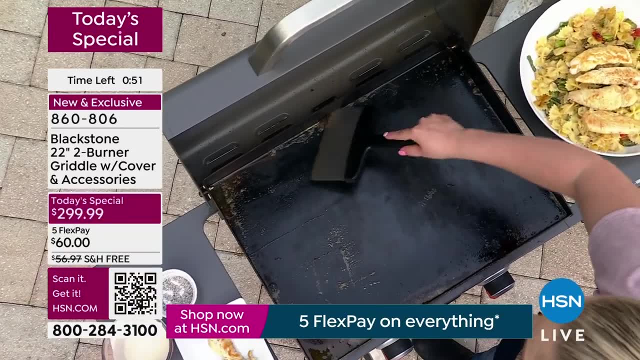 Okay, Then we have this big gnarly guy who's like, he loves outdoors. he lives in a tent- Yeah, You know he's cooking some crazy things. And then you know, you have, you have a vegan, you have a vegetarian. 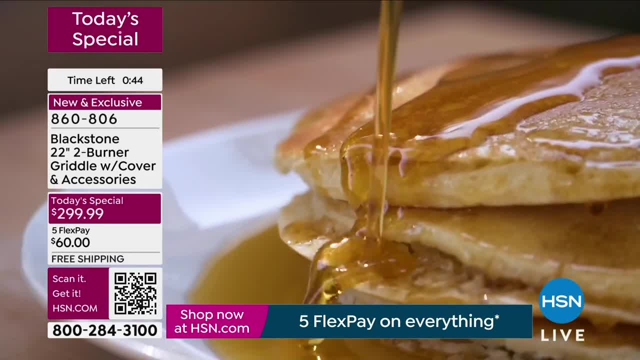 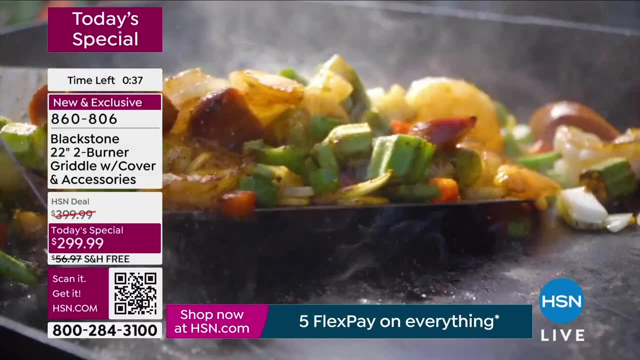 So I want you to kind of go out there look at fun recipes, because once you start trying, you're going to want to be on this thing every day, all day, every day. It is so fun. There's a reason why, look. I mean, everybody's been having fun over here. 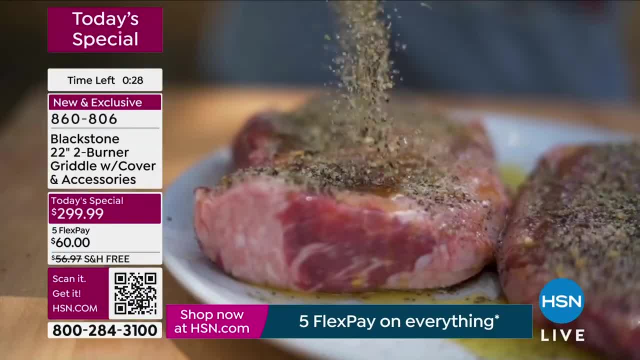 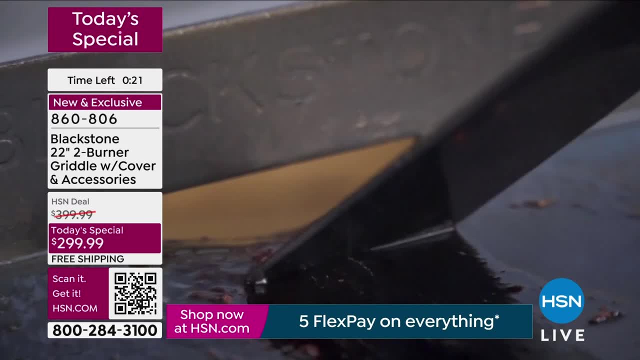 We've had all the crew come in Every host that I've been with today they said I haven't had this much fun, I know, And forever on set. I know, Because they forget what it's like to try something new, like actually try it. 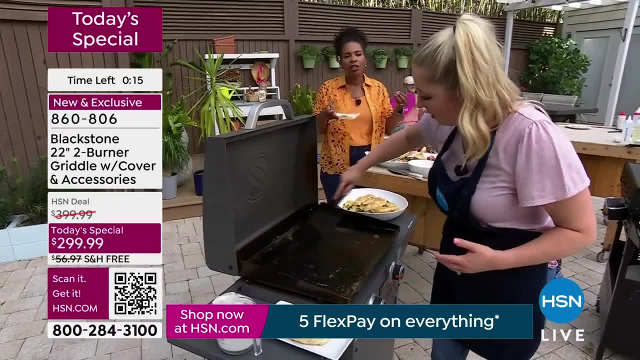 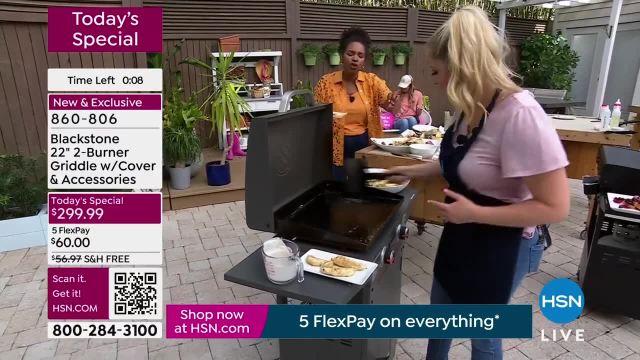 It's and the food is. the food comes out fast, It comes out delicious. You're watching it, You're seeing it done. Yep, You feel like you have a part in it. If you want to add, say, can you put a little bit of extra, whatever it is, on yours? 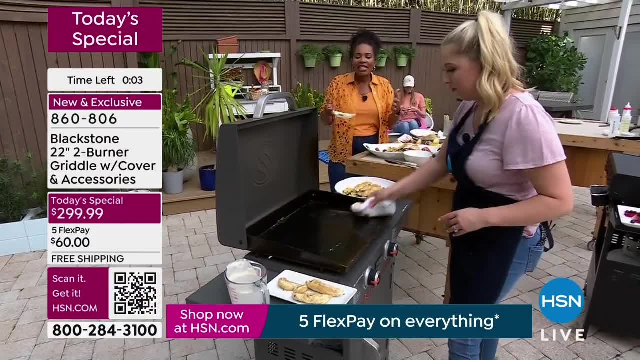 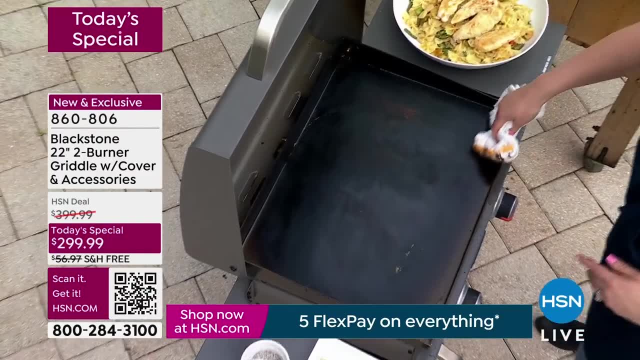 Whatever it is. A little extra cheese on mine, Yep, And you can see it happening. This is restaurant style cooking. Gotta love that. It is restaurant quality: eating Yep And serving yourself and your family. That's it. You are not washing dishes at the end of the day. 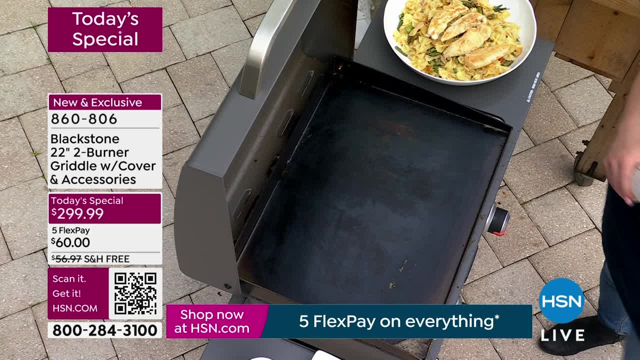 No, ma'am Taylor has made enough for an entire crew of people. I have- You gotta love that. And she doesn't have to wash a single dish because you don't. You don't wash dishes when it comes to your food. 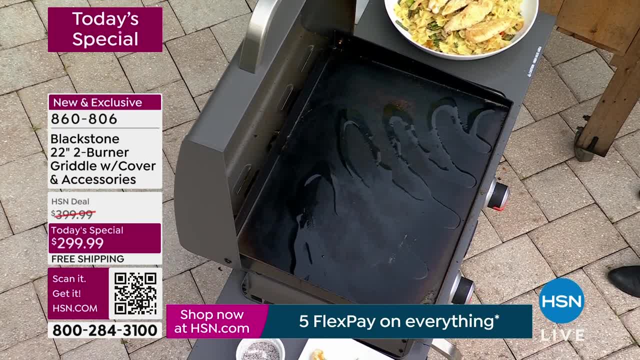 You don't wash dishes when it comes to your Blackstone, because you cooked your entire meal right here. That's right, 22 inches on this space. You're getting everything that you need. You just add the food and you add your own propane tank. 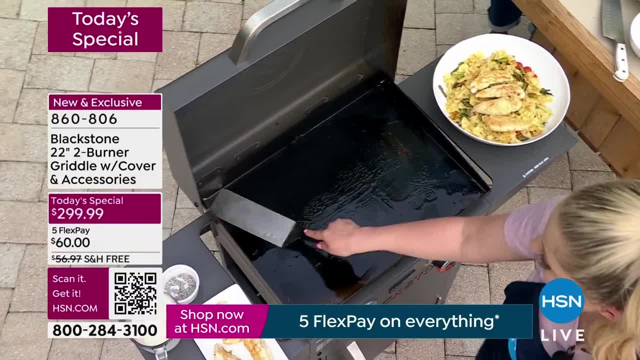 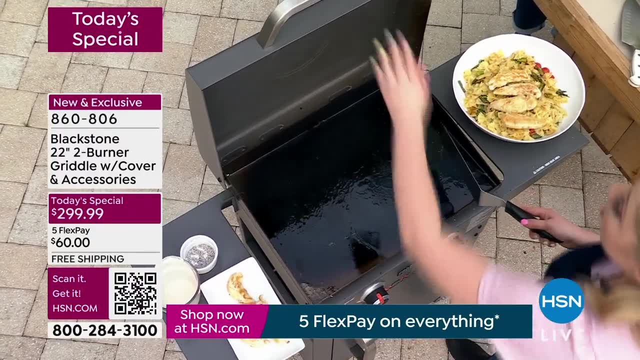 And that's it. Blackstone does the rest. And don't forget to add your oil when you're done. You want to add your oil and let that oil really sit. Turn your griddle off, Let your oil sit, Cover your hood like that and then put your cover on. 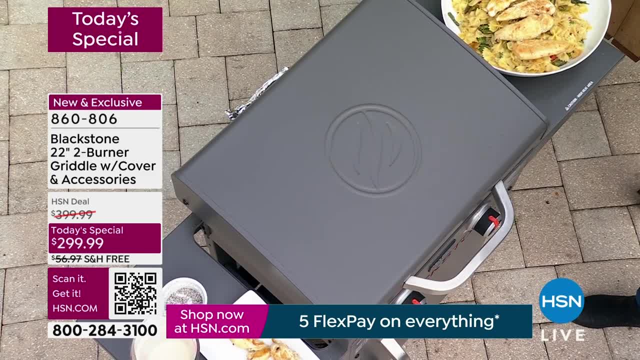 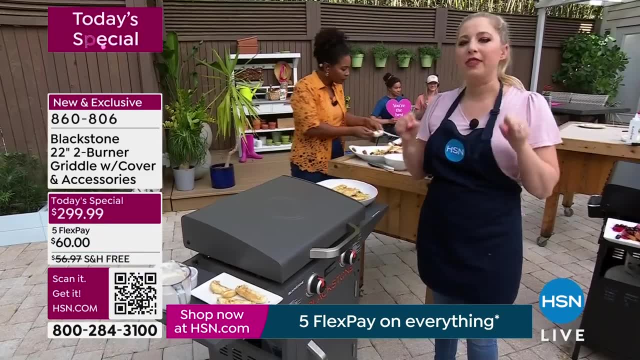 And that is it. I'm heading inside with my dinner here, I'm not having to worry about anything else. The worst feeling, Tamara, is when you're sitting down, you're enjoying your dinner and you're thinking about the cleanup. 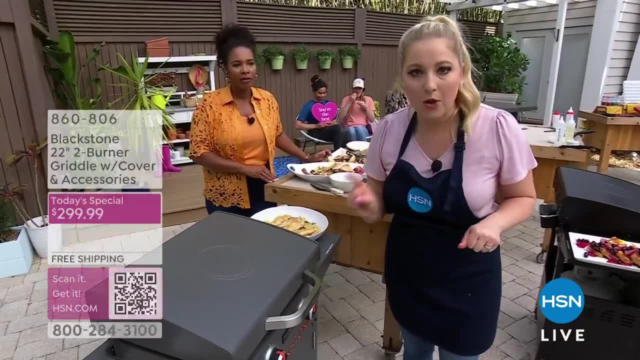 I don't care what anybody says. That is the worst part of cooking and we all know it. Ask my husband: Yeah, We don't want to do it. I know you're watching, Taylor. thank you so much. Thank you so much. 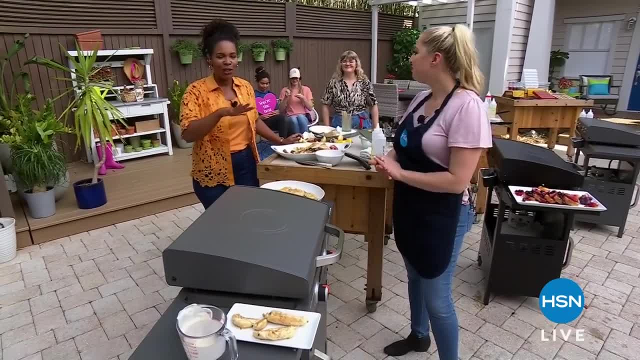 It was so fun to be with you today. This was fun. Enjoy your Blackstone. We're gonna take care of this for dinner. You can go ahead and pick up your Today's Special, and I know we've got J King coming. 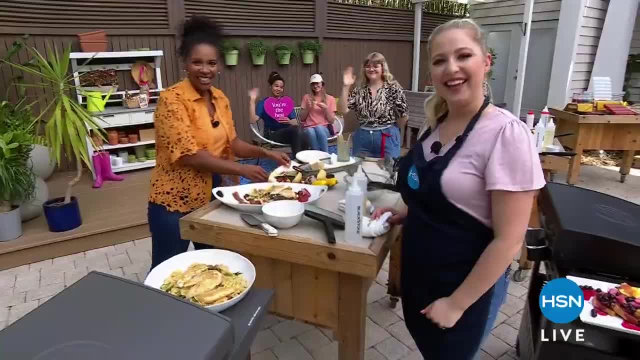 up next. We'll see you again next time. Bye-bye, Bye-bye.